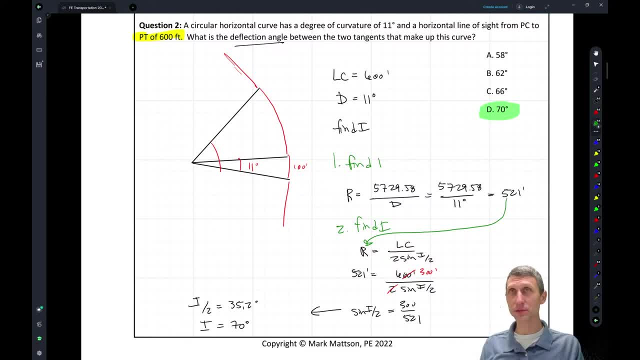 I think this is just just talking over these two problems just quickly, but hopefully the resolution stays good, Hopefully the video stays good and hopefully there's not a huge lag here. So thanks for staying along for the ride, but let's keep going, And if 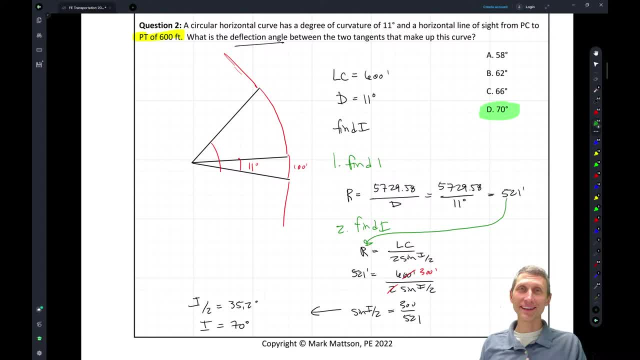 all else fails, what I'll do is I'll just record this, not live, and post it later. So who knows? but I appreciate at least you guys have have had the ability to to come back in here and get your questions answered, at least live, and hopefully I can address those in a 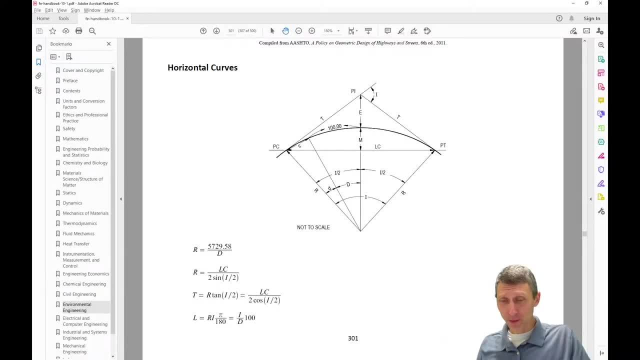 in a prerecord as well, if I have to do that later. but this will be good. We'll keep going as long as you know, the computer doesn't blow up So which in questions involve radians. it kind of this is the idea here. 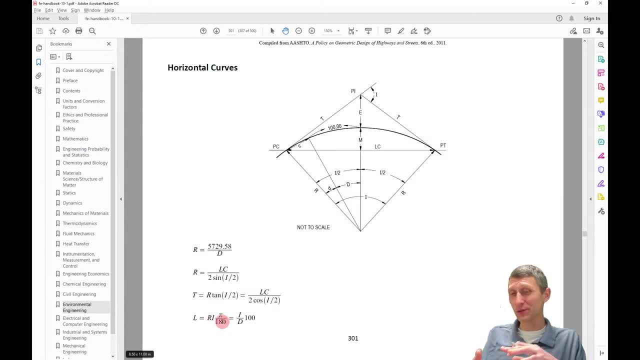 this PI over 180 is where we go from degrees to radians. So normally all these eyes are in degrees, So so you don't have to worry so much about degrees here. And I was hoping, I was really hoping that that you know. 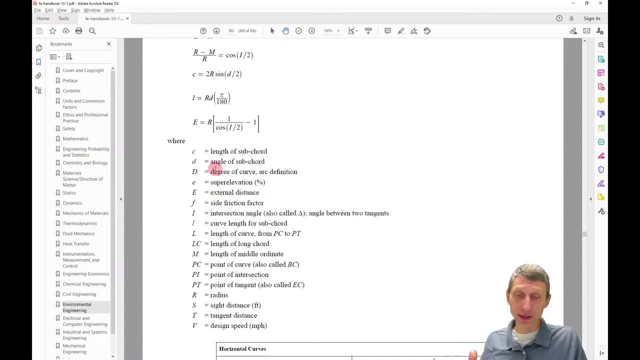 that they defined this in here, where this is a degree in degrees, but they don't exactly so even I hear it's the intersection angle, also called delta. It's not defined as degrees but but when you do the math out- except for like these problems with the Ober 180 where you're converting from degrees to radians- 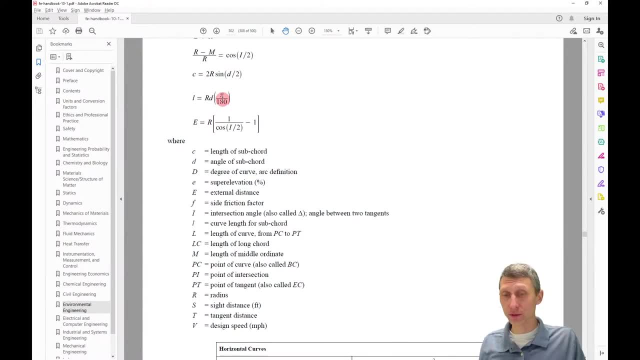 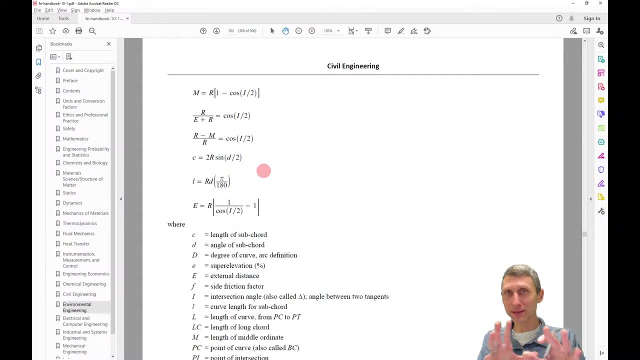 That's where life, where you're going to use degrees is, is is as far as I remember. remember, i mean, i i've looked these. um, you know, i taught the transportation analysis course for a couple semesters and you kind of have to get just like with all this stuff. i mean, you guys took a. 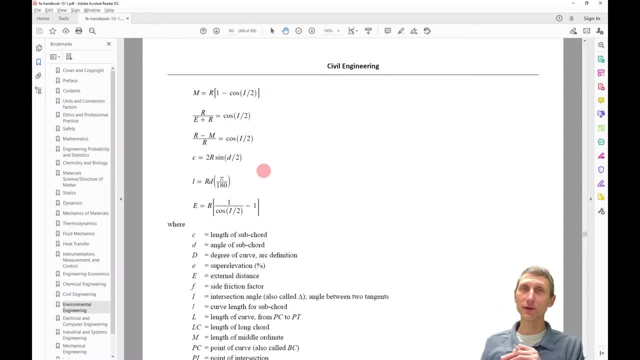 transportation class at some point in your civil degree, right, and the idea here is you have to kind of go back through and remember this stuff. so the the reviews aren't completely comprehensive, right, they hit on a lot of those topics, so they hopefully help you to see where you're rusty and 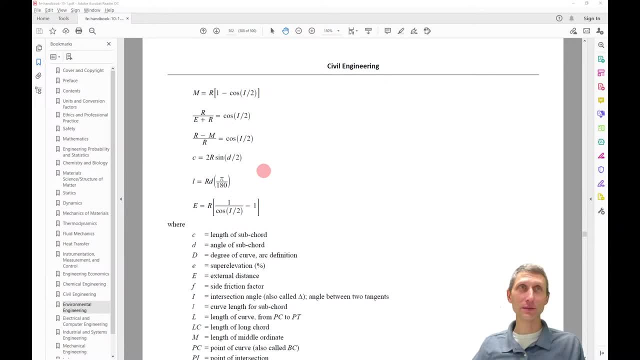 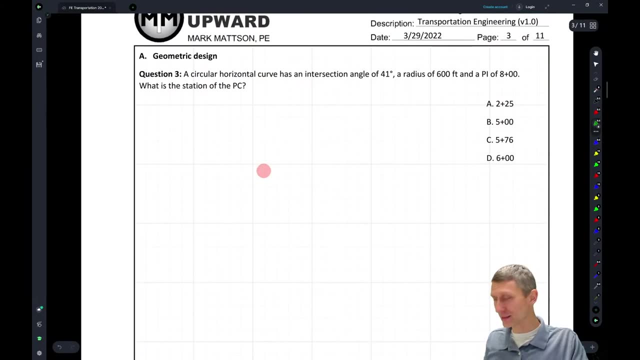 can also get some additional. you know, help you to know where you need some additional practice. so a couple of these questions, horizontal curves and let's keep going to question three. so question three: we have more, uh, we have more horizontal curves, so horizontal curve is an intersection. 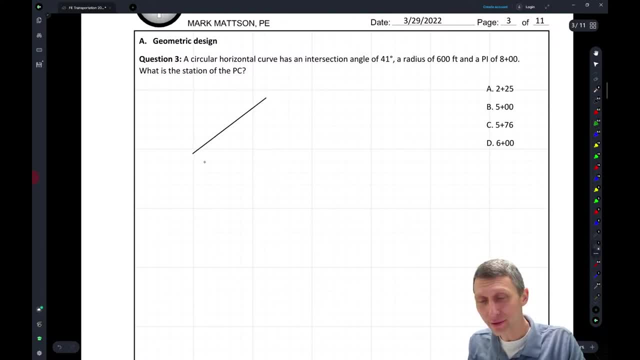 angle of 41 degrees. so again, whenever i have a problem like this, i like to just draw this out. so i know that i have 41 degrees in here, right, i know i have a tangent coming in, a tangent leaving, and those tangents are going to be the same as the tangent leaving and those tangents are going to 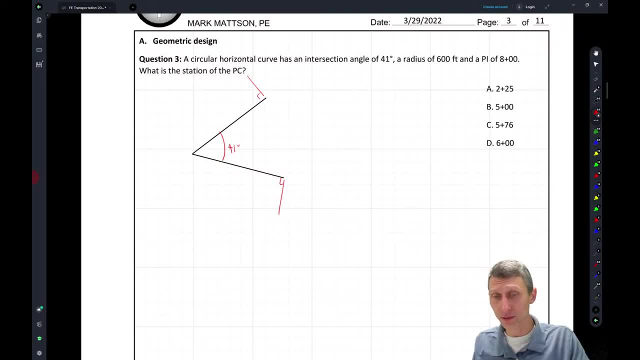 be the same as the tangent right. they're 90 degree angles. they're tangent to the the curve right, but they're 90 degree angles, they're tangents in here and that should make a that should work pretty well, right? so we know that this radius- i wasn't too creative here, but radius 600 feet, pi of eight. 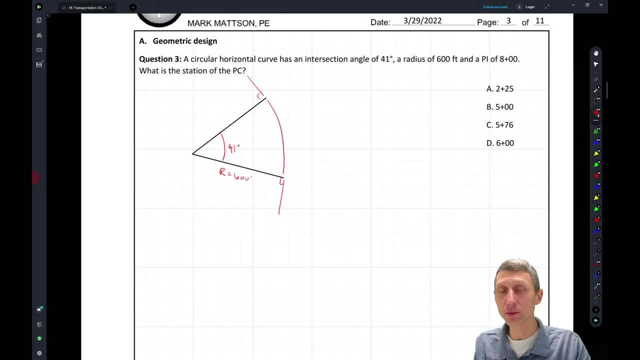 plus zero, zero. so again that point of intersection. i kind of mentioned it when we were looking at, uh, the reference handbook. but that's if you were to extend these, these tangents straight out, right, so if you extended this and you were to extend this, and you were to extend this and you were to 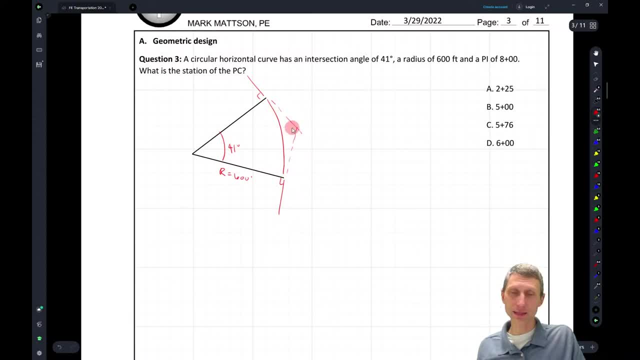 extend this tangent. i didn't do a great job with a straight line, but if you extended these tangents straight out, you're going to get your point of intersection between those two lines at this point. and that point of intersection, we're told, is eight plus zero, zero, and we're asked for the station. 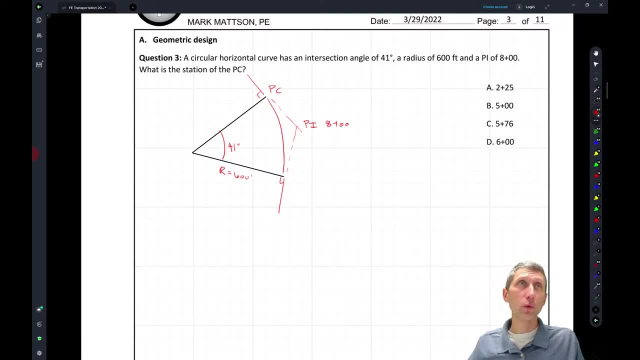 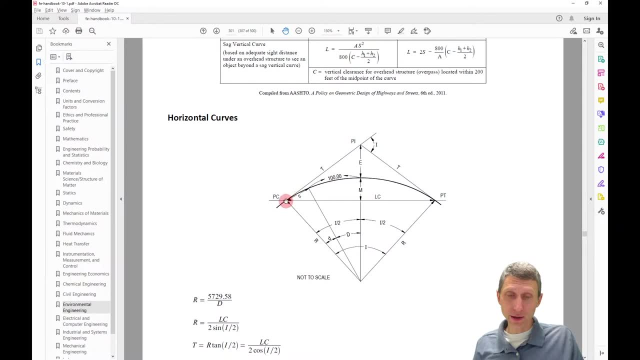 of the point of curvature, the pc. so the way curves are are laid out in the field. um, you have a essentially point of curvature here, right, and you have this tangent, you have a tangent, you have this, this angle up here as well. but this, this t distance, is the distance from the point of 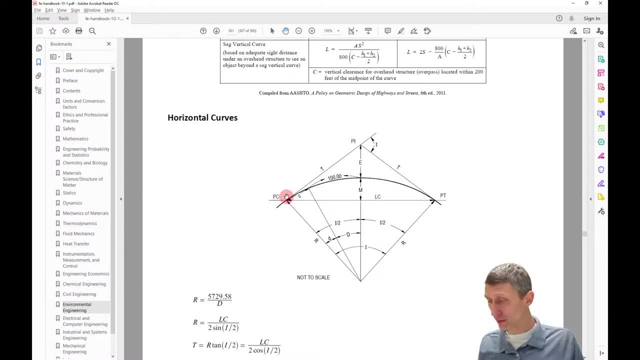 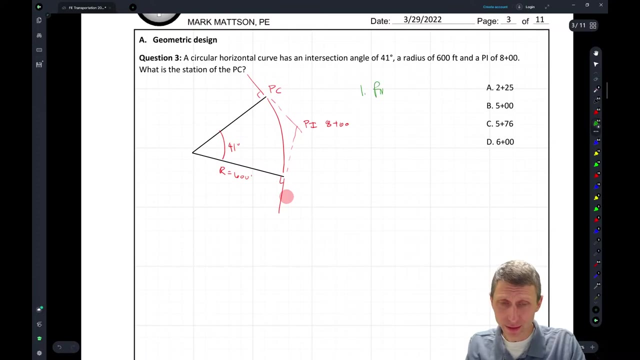 intersection back to the pc. so the cool thing with this is um, again, it's not a super crazy challenging problem, but it's one of those problems we have to know kind of a couple steps. so with this, the steps that we're going to take is first: um, we're going to find that distance t. 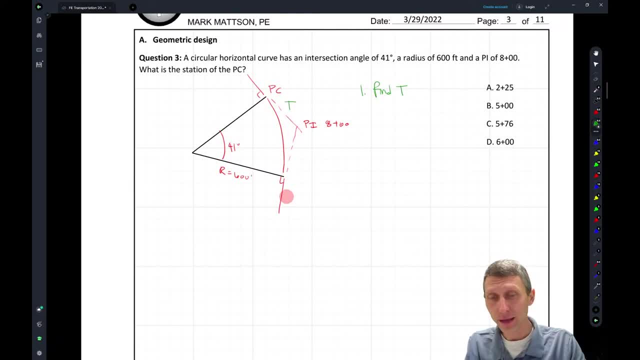 what's t? t is this distance right from the pc to the pi, and then, second, what we're going to do is we're going to subtract, right, we're going to subtract t from pi, so pi minus t, and that's going to give us our point of curvature. 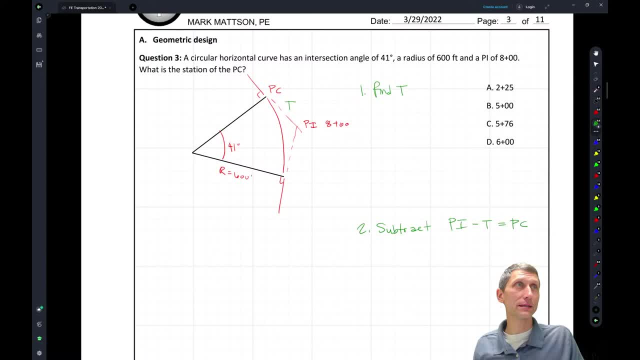 okay, so hopefully this makes a little bit of sense. um, hopefully it's not too crazy and we're able to make this, this work. so, uh, sorry, i'm just trying to get one other thing set up here. man, tonight's been a rough night with um, with with getting everything working, but i think we're working now. so 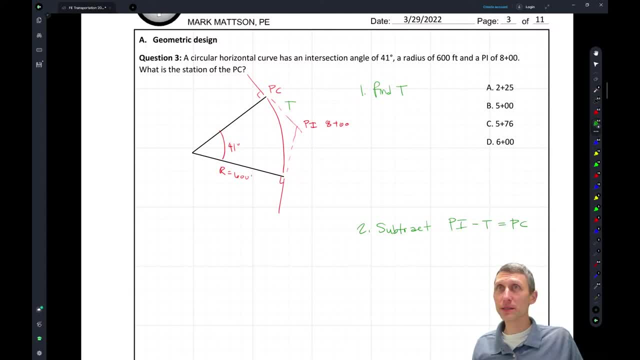 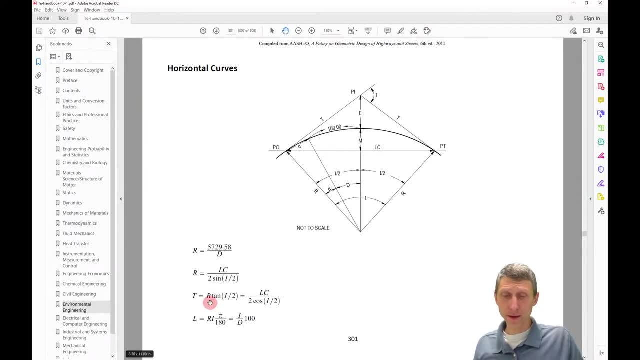 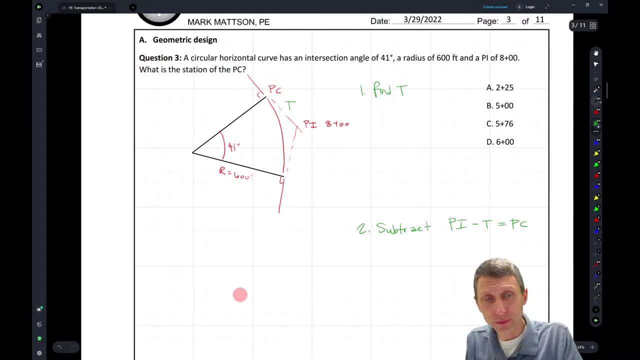 so this is good. so let's do those pieces right. so t? um we have an equation here in the, the handbook that says: t is, you know, um? r times the tangent of i over 2.. so we can come back and we can solve for that right. and t equals. 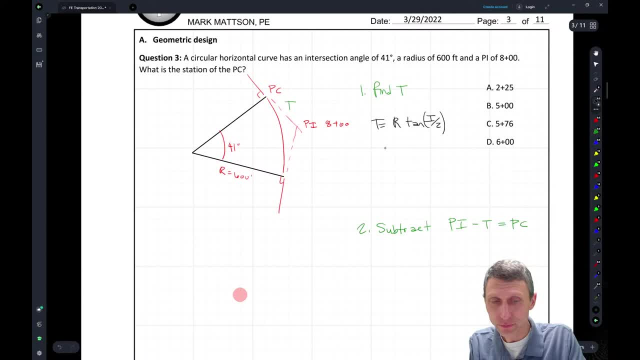 tangent of I over 2,, which is equal to what we were told that the radius is 600 feet times the tangent of 41 degrees over 2,, which equals- you know this t value is sorry, dropping my calculator here too- 600 times the tangent of what 41 over 2.. So 41 over 2, and I get about 224 feet, So 224. 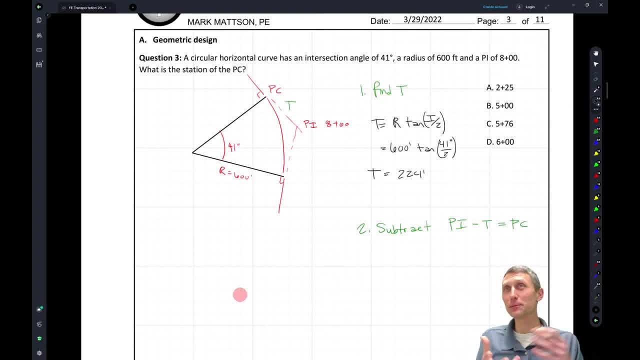 feet And stationing. all stationing is is it's per 100 feet. So typically when you're laying things out on linear projects, you have a 100 foot tape or you have a 100 foot station in between and you just use that to lay things out. So what that looks like is 8 plus 0, 0, right. 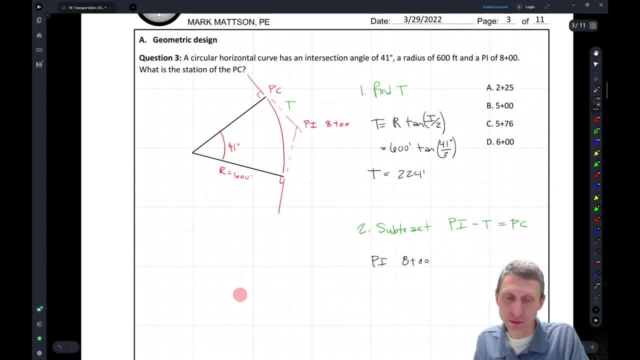 This is what it looks like. So this is what it looks like. So this is what it looks like. This is what it looks like. So this is what it looks like. So this is what it looks like. So this is what this point of intersection is: 8 plus 0, 0.. You could also just write this as 800, right, This is. 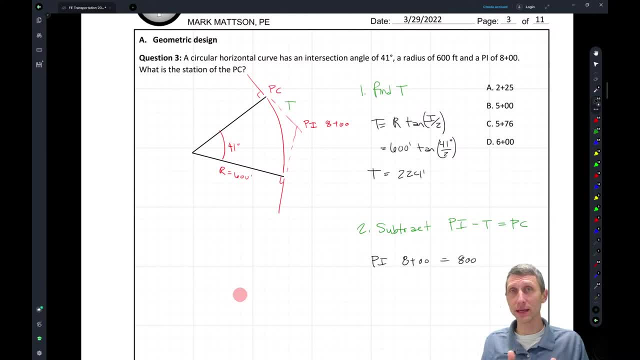 just 800.. The plus 0, 0, it's kind of like the idea of you're starting at 0.8, and then you're going 1,, 2,, 3,, 4, all the way up to 100 until you get to 0.9, right, Or 900 feet from your reference. 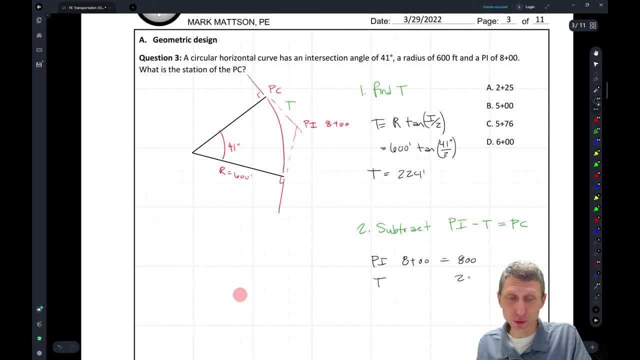 point. The tangent we said was was 224 feet. So when we subtract these we're going to get our 75. So here it's 576 feet, which also equals 5 plus 76, right. So I'm working kind of left to. 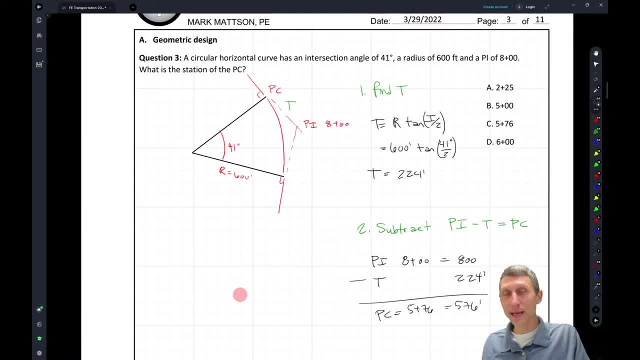 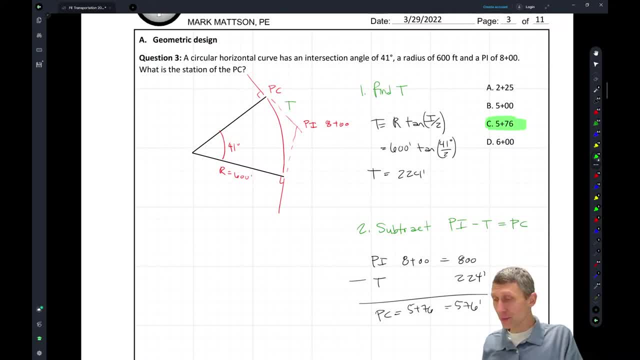 0.5 plus 76.. Okay, But that gets us into the stationing idea and it gets us into kind of this next: you know this, this next, this next problem as well. So we're going to go shift from. 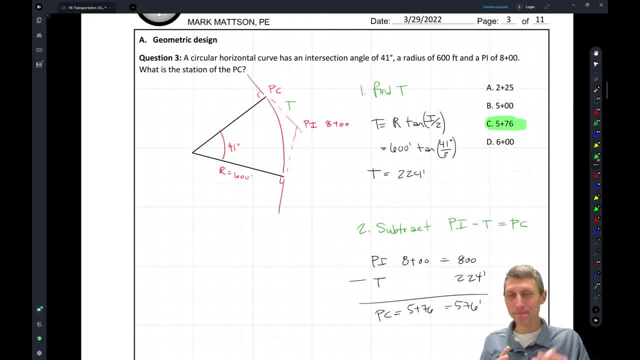 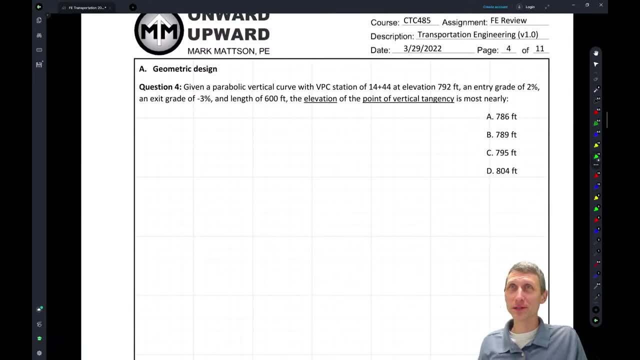 horizontal curves to to vertical curves. But you know, as we go here it's it's. you know some of those curve problems are going to be two-step problems. Some of them are going to be easier than others, but hopefully it works. So is the PI minus T in the handbook. 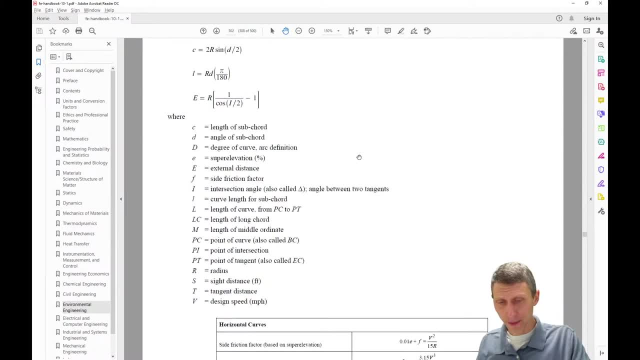 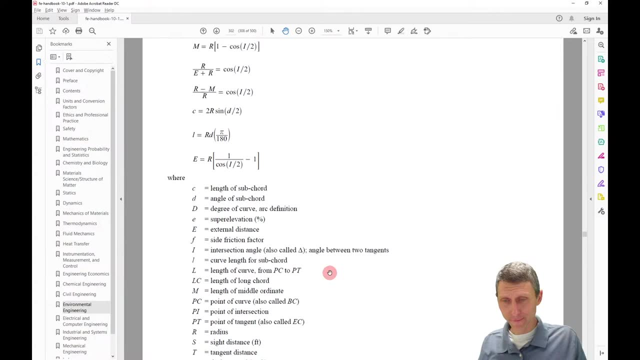 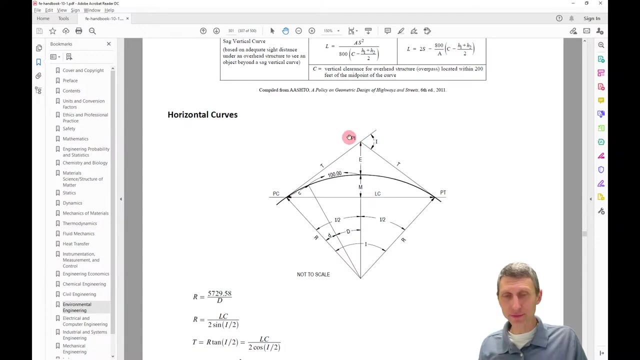 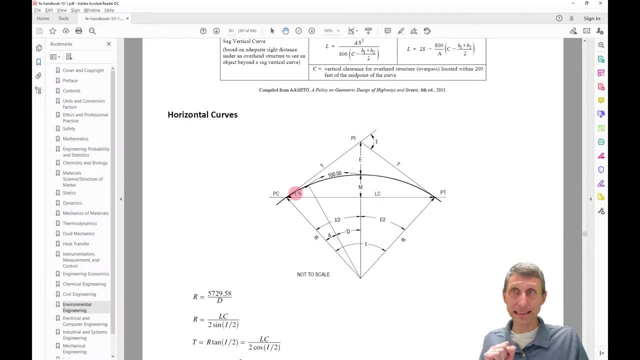 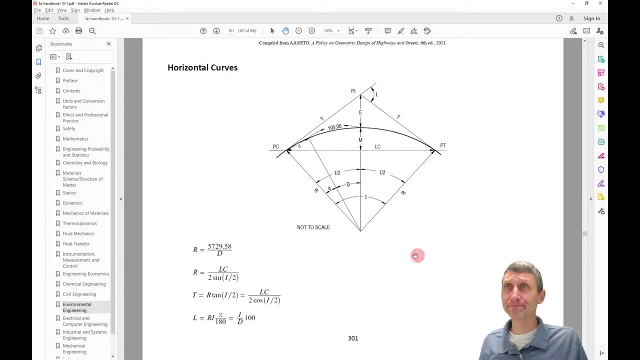 here, T is here, and PC is PI minus T. Okay, So so I don't think that that equation actually shows up there. It's not a super crazy thing, So so let's keep going. Okay, So, let's keep going and we'll keep. 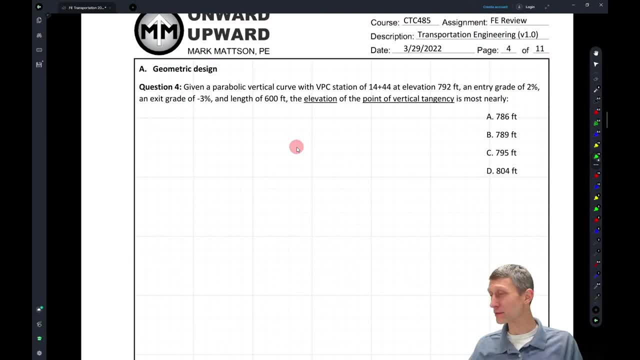 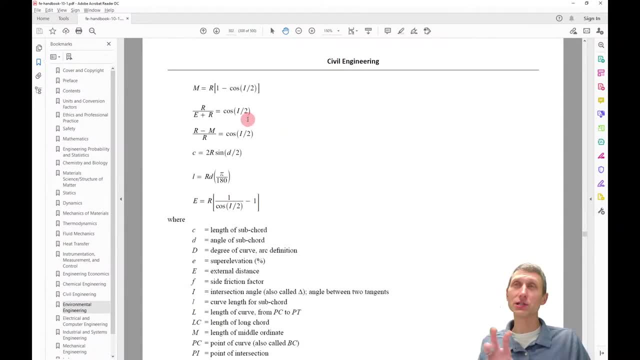 going And now we get to vertical curves, So horizontal curves. I honestly I could have probably spent a whole hour just on horizontal curves and gone over more questions on here with M and R and E and you know all these other pieces of it, Right? So there's a lot of other. 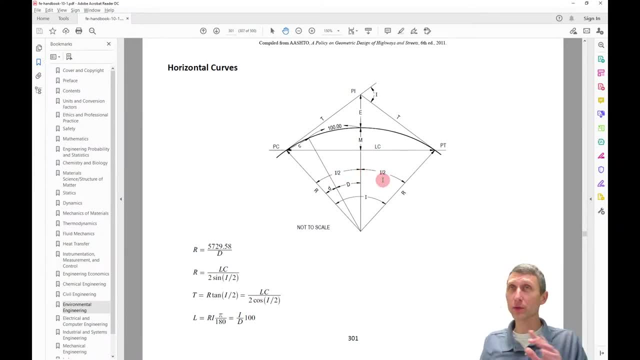 pieces. It's worth. it's worth going through some of those curves. So let's keep going. It's worth looking at some of them. you know, and you can rearrange this all over the place, but I kind of wanted to hit some of those pieces about the angles, about the chord length versus 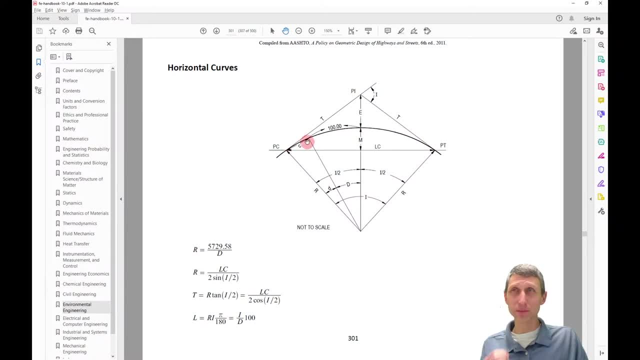 the, the, the arc length, the stationing, the, you know the PC, the PI and that sort of thing, the degree of curve Right. So if you know what the pieces are, you're just looking for formulas. 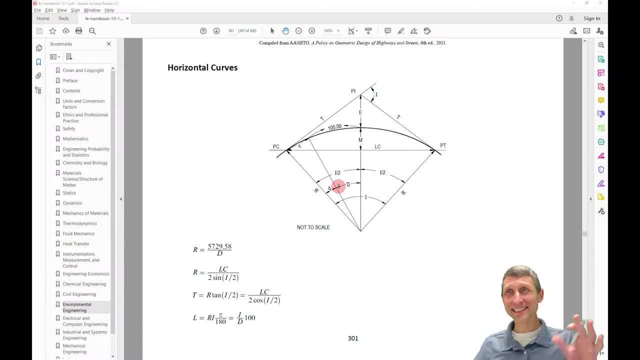 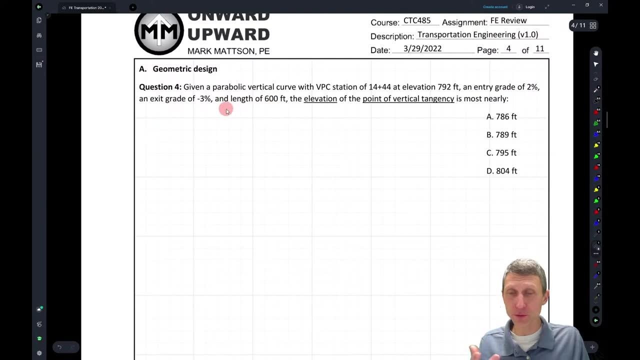 to kind of plug and chug to a certain degree, And sometimes it helps to use common sense here. So, so let's, let's take a look at this as well. So this one: we have parabolic vertical curves, So most vertical curves are parabolic, They're not. 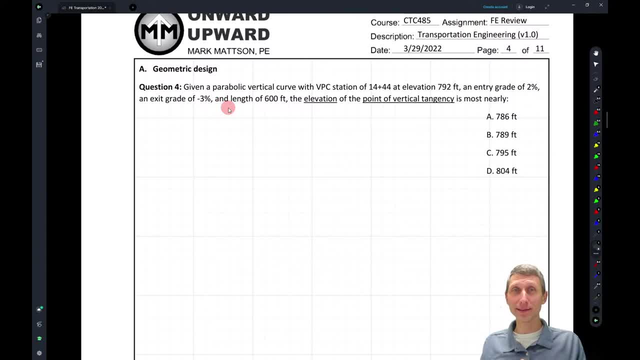 circular. That helps as you're going over, just with the whole gravity thing And you don't feel like your stomach's in your you know you don't feel your you know that whole rollercoaster thing where you're, you're accelerating too much or whatever, And that's the the vertical curves. 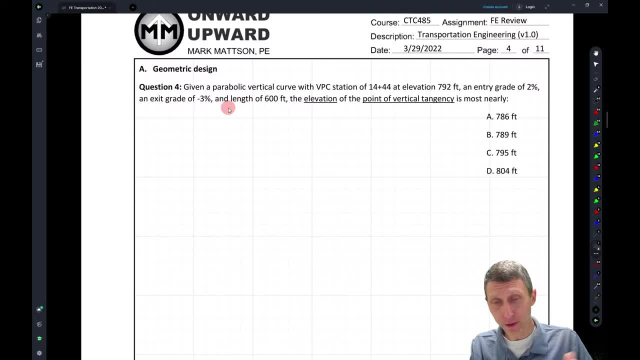 try to help with that. But here we have a parabolic vertical curve. Again we have a VPC. So we know what. we're starting at 14 plus 44. I and we have an entry grade of 2% and exit grade of 3%. So we're coming in a little bit shallower than. 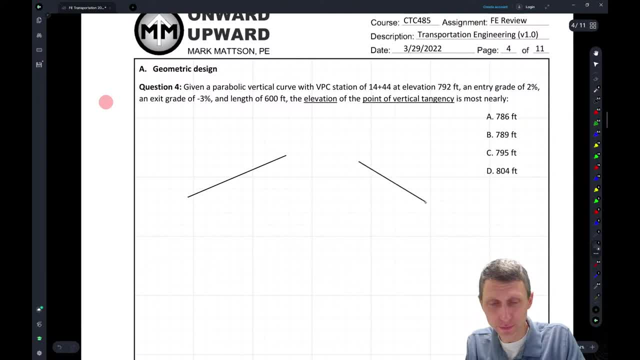 than we're leaving. So we're coming in, you know, at 2%, we're leaving at 3%. I'm just gonna exaggerate that here. So we're coming in at 2%, We're leaving at 3% and I'm leaving the negative. 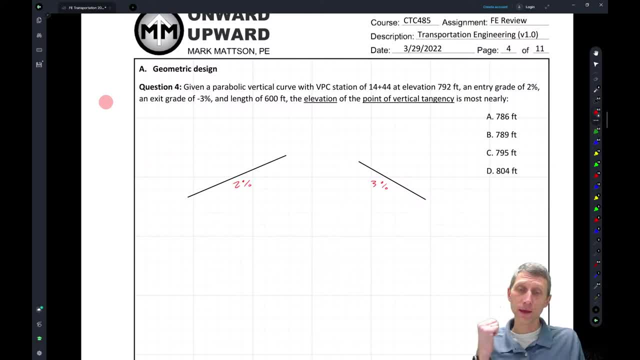 sign off there. but the idea is a positive grade is typically going up and negative grade is coming down And we're gonna have this curve that I, if I could see what I was doing a little bit better, it would make it even better here. And let me 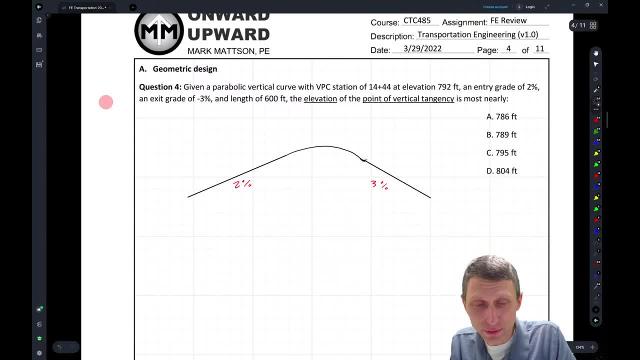 there we go. That's close enough. So so that's you know, that's our, that's our curve. We know a couple of things. We're told a couple of things. We're told that this point of curve, or the VPC, the VPC has what It has an elevation of. do I have an elevation? 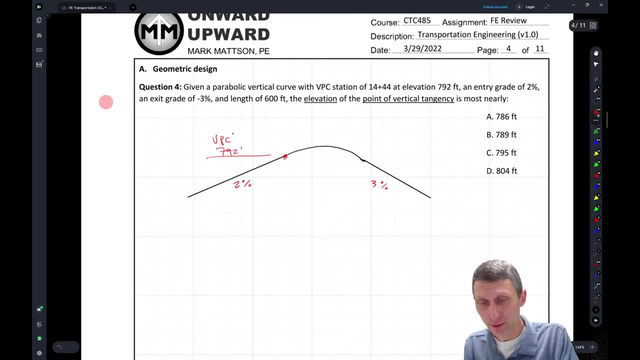 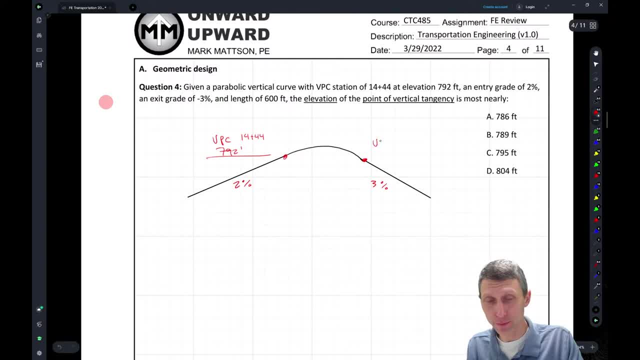 of the point of vertical tangency. So this is our VPT And what we want is that, that elevation. what is that elevation? Okay, Good, good question. But this is where it helps to have maybe a little bit of you know. we can come back into our handbook, We can use some of these formulas. We 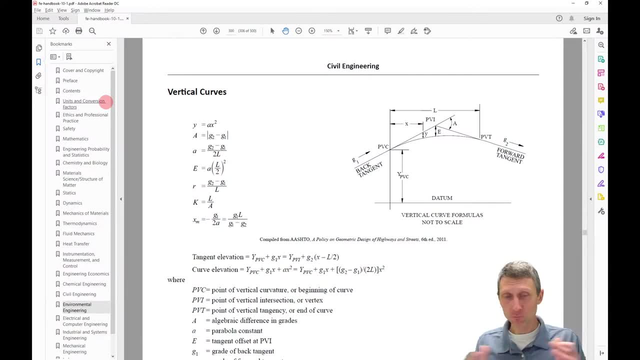 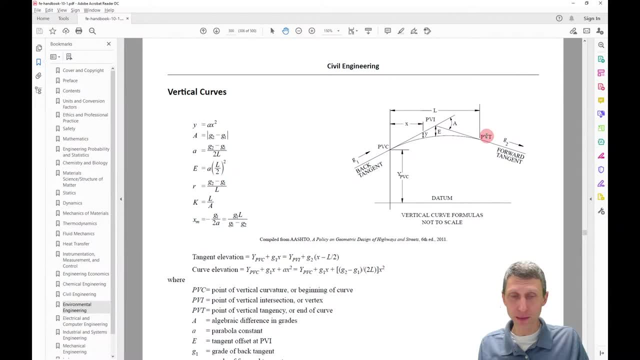 this is the beginning. We have our back tangent here, We have our length of curve, We have our PVT And this is where we are given some, some values. here We have tangent elevation right. The tangent elevation is the point of vertical curvature plus G1X And the point of 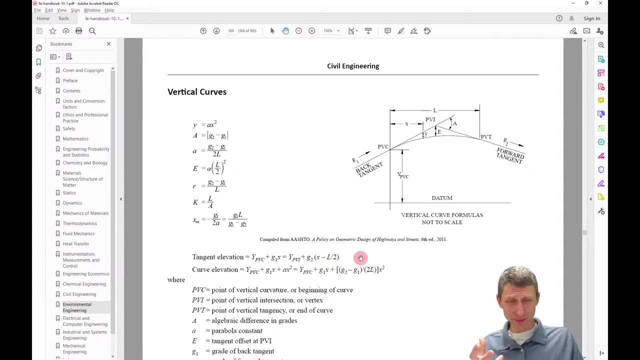 you know, YPVI is, is, is, you know, G2X minus L over two. So, and then there's this other equation down here And these equations look complicated and honestly, I don't really like the equations that, the way that they're. 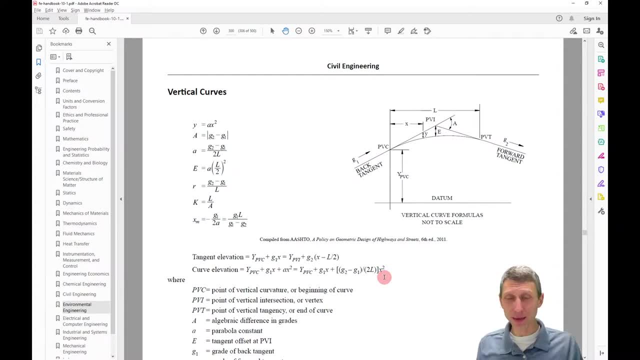 presented in the book, that much because they are the handbook, that much because they they make it, I think, more complicated than it needs to be. But let's just, let's just think about this equation. I'm going to take a look at this tangent elevation equation real quick here. 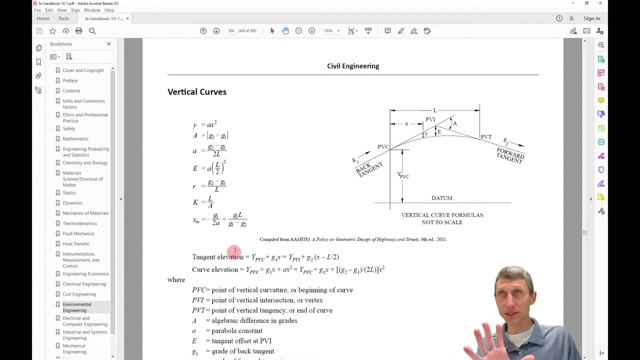 And what's the tangent elevation? Let's just back up for a second. Tangent elevation is the elevation of the tangent right Of the line The curve elevation is? is, you know, the curve Curve elevation? What we want is the point of vertical tangency, So we can kind of use either. 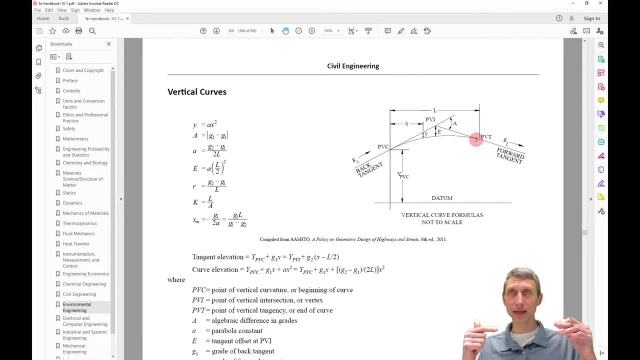 of them. but let's just take a step back for a second and think: what are we trying to do? We're trying to figure out. well, we start here, we go up a certain distance, we come back down a certain distance, right? So that's kind of what we're doing. So let's come back to what we have here. 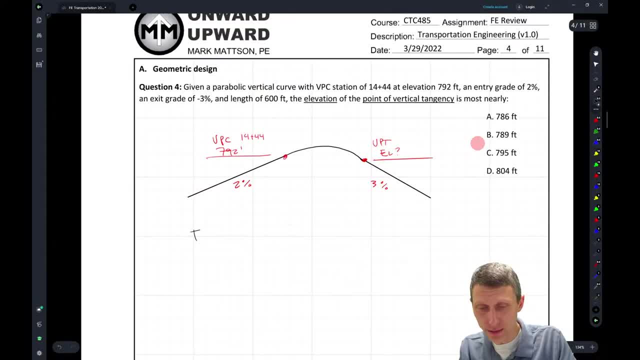 I'm just going to write that tangent elevation formula down. So the tangent elevation, tangent elevation equals Y PVC plus G1X And it also equals Y PVI plus G2 times X minus L over two. Okay, So this is. this is kind of cool, but how does that help us? Well, you know what we are told. 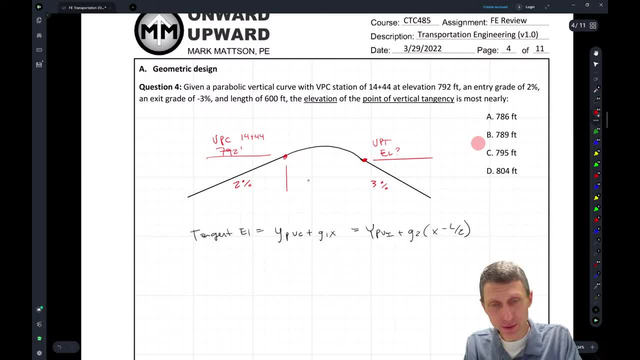 is. we're told the length of this curve is. are we told the length of this curve? Yeah, we're told the length of this curve. Again, just using consistent numbers here, just because probably I had it in my mind when I was writing the. 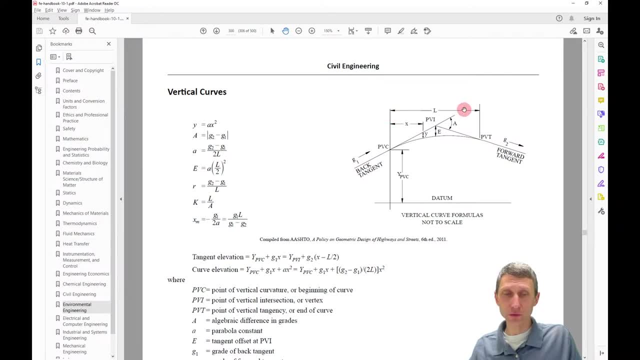 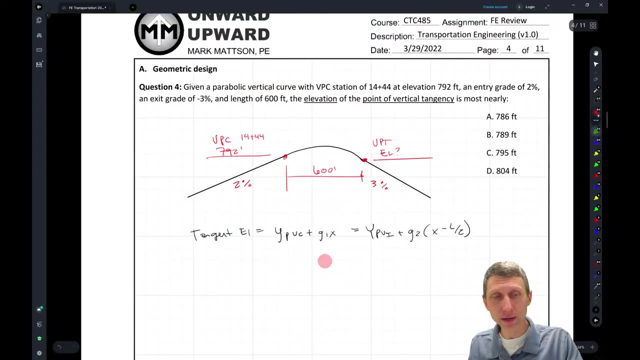 questions. but the length of the curve that's our L is is 600 feet. You see, this X, X minus L over two. that's going to be sort of significant here, because what we have going on here is this is the tangent kind of like, or this is the elevation of that tangent from the PVC to the PVI right. 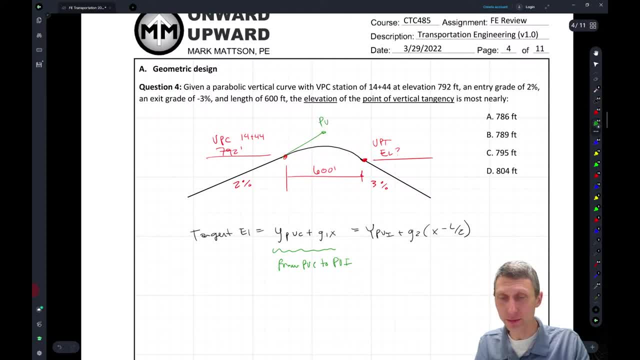 So this is kind of like this point. So I'm just going to kind of exaggerate this a little bit. but this is up to the PVI. So this is, like you know, equation one over here And then equation two again. let me try to write. 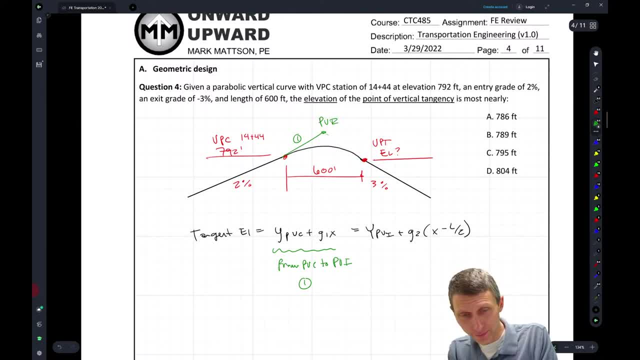 this a little bit better here, Man, I got my computer cocked a little bit to try to keep it cooler, But let's see. So this is kind of like this part's, kind of like equation two: right, This goes from the PVI to the PVT point of vertical tangency, or it goes back tangent. 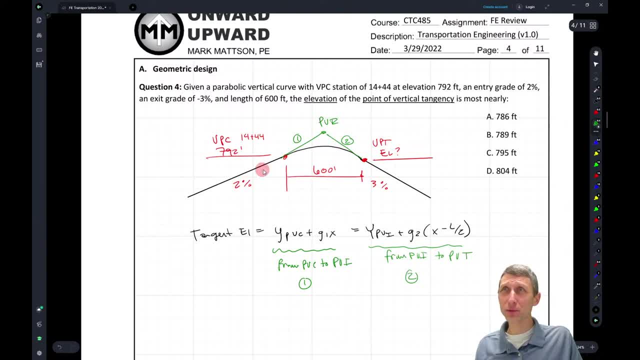 right. But if you think about this, what are we doing? Well, we're at 2%. We're just going to go up 2% until we hit the middle here, and then we're going to come back down at 3%. That's it. 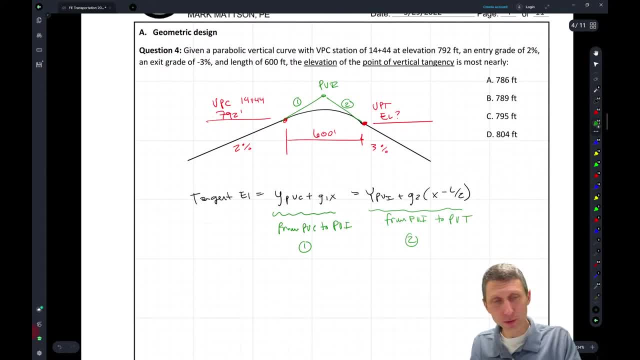 right. So when we think about this, right, all that we're doing is we're saying, okay, we're going to start at 792 feet, We're going to add. what We're going to add, X, X is, and this is where- yeah, I think this is where you put that in the chat, But yeah, 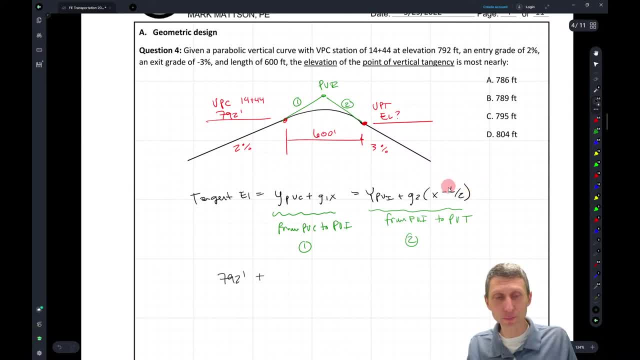 this distance and you'll even see it right here, that L over two, right, That L over two is going to be the distance from the PVC to the PVI. So this is going to be right, this is going to be. 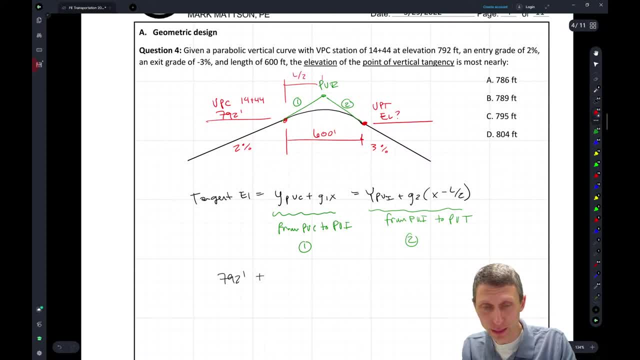 a distance of L over two and then we're going to have another distance of L over two. So, in other words, it goes up 2% and then it comes back down 3% for the distance of L over two. So what does? 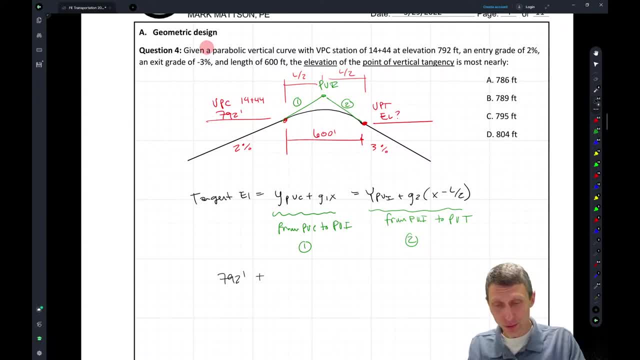 that look like It goes up 2% and then it comes back down 3% for the distance of L over two. So it's going to look like this: We're going to say essentially, we're going to say plus 0.02. 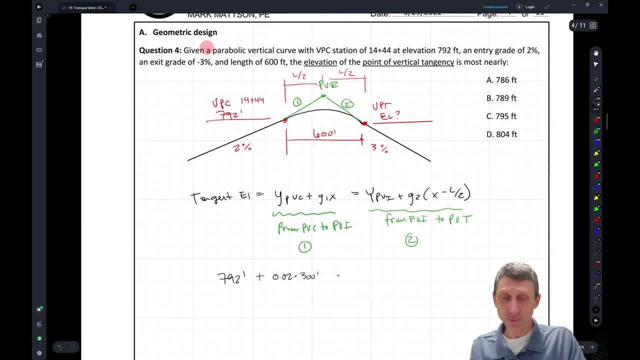 times 300 feet minus, and then we're going to go back down 0.03, sorry, 0.03, not 0.03,- 0.03 times 300 feet, and that's going to be our distance. So what we're doing is: 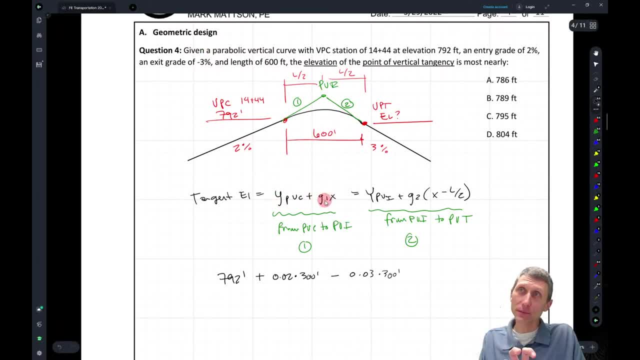 essentially, we're saying, okay, we're going to take this formula, but we have to go up to the PVI and then back from the PVI, back down to the PVT. Okay, so it's a piecewise formula, but then we're going to go up to the PVT and then back down to the PVT. So 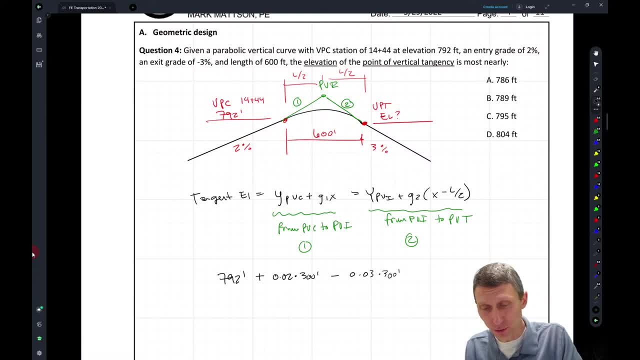 the handbook doesn't really tell you. it's a piecewise formula and that's what you have to use to get here. So, but even just using some kind of common sense, okay, we're going up a certain distance, we're coming back down a certain distance. Once you know, it's 300 feet up. 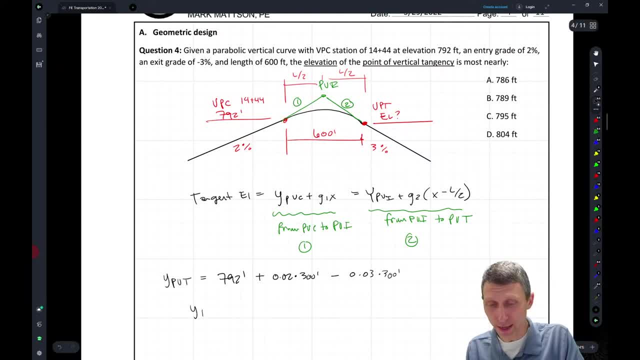 300 feet down. you know the slopes and you can solve this. So the YPVT is going to equal. what do we have? 792 plus 0.02 times 300, minus 0.03 times 300, and that gets me down to 789.. 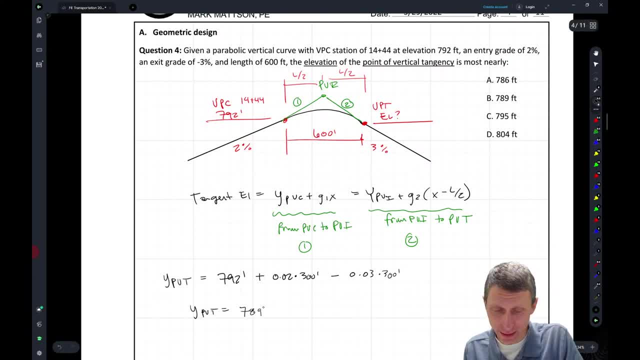 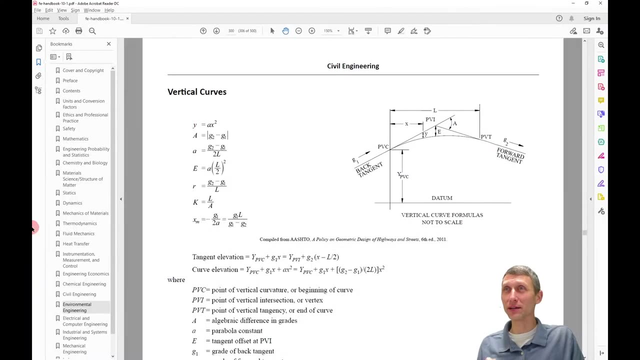 Okay, so 789 feet, which I think works and we're good. But again, it's understanding kind of a little bit of what the formula looks like. it's understanding a little bit about what the equation's actually giving you because again, this equation here, it doesn't really tell you. 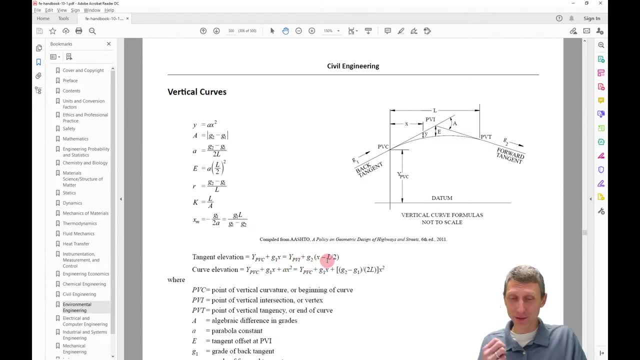 all the bits and pieces of what that equation is, but you know, as you get used to using this, it'll work. And even this curve elevation, right? this is just a parabola, right? this is a parabola. 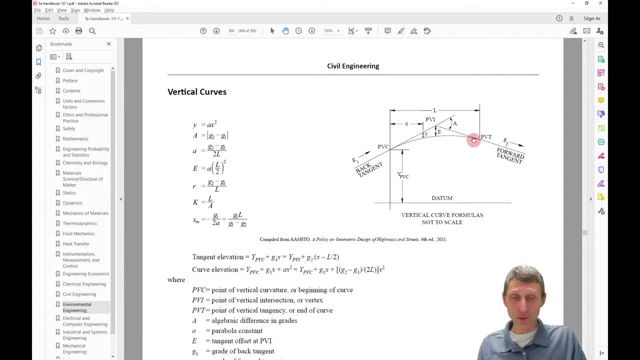 here, So you could use this to decide whether you're going to be able to do it or you're going to this as a parabola and make it work, right? I mean, we could even come in here and use this formula. 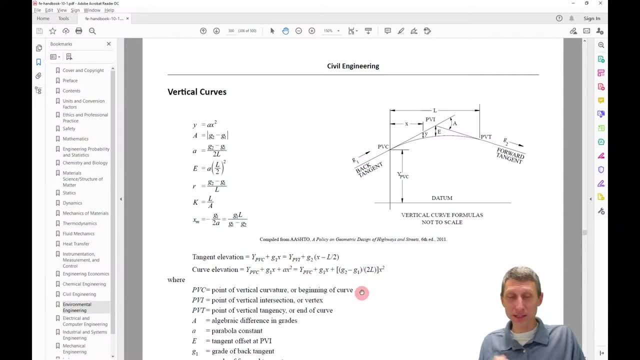 to get. we could use this formula to get the point of vertical tangency. So, if we use an X value of 600, right, We could do that, We could do that and we could use an X value of 600, but this formula is a lot more complicated. 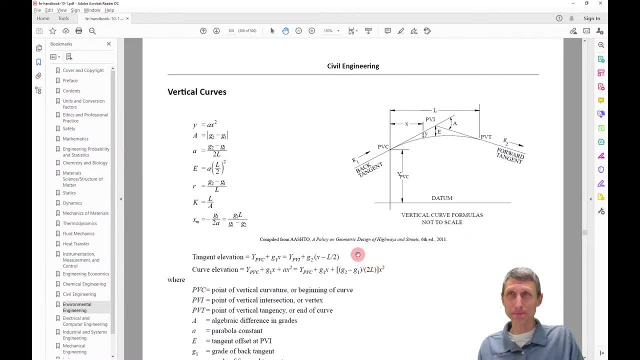 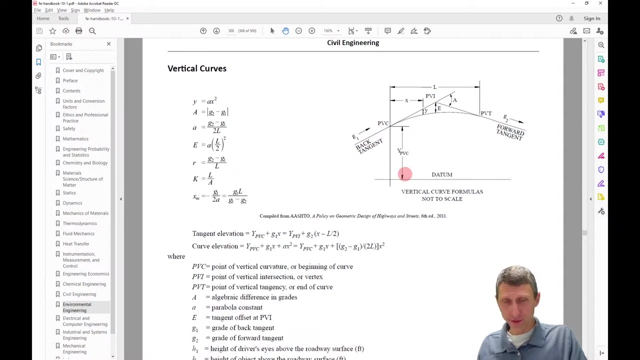 than what we just did with the, you know combining these two formulas, And so hopefully that helps a little bit, Hopefully. I wanted to start with this question because it just gets some of those parts and pieces out there to make some sense. So XM, XM, where is XM? 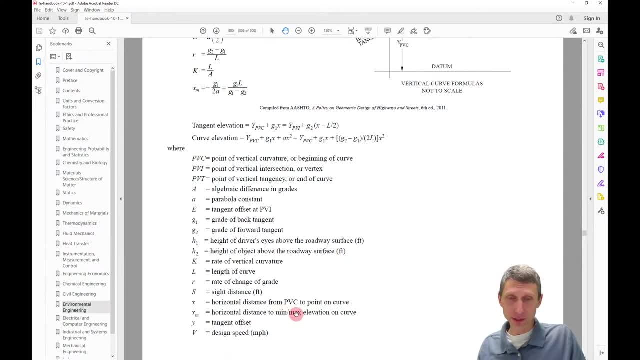 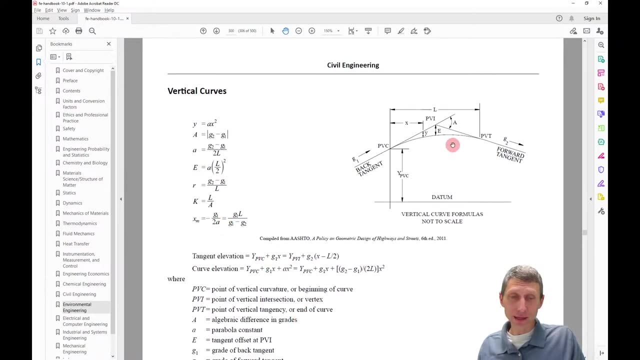 Are you talking about the mid, the horizontal distance, the min max elevation on the curve? We could be, you know, we could be required to find that as well, So the XM. that would get us to like the crest point here. 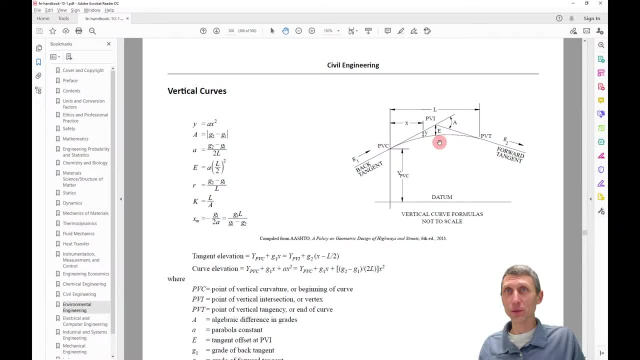 but that's not necessarily going to be in the middle of the curve right. So we could find XM if we needed to or wanted to, or the question might ask for XM, which is going to be different than what we just did, right. 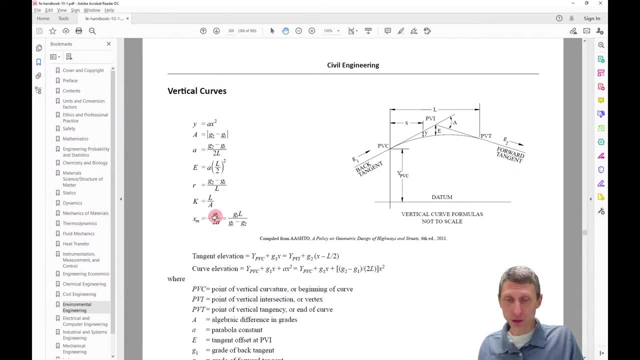 So if we want to, if we need to find XM, we can use this formula to find it, but to find it it's going to be a two-step process. Well, actually you can do it in a one-step process because they give you the one formula here. 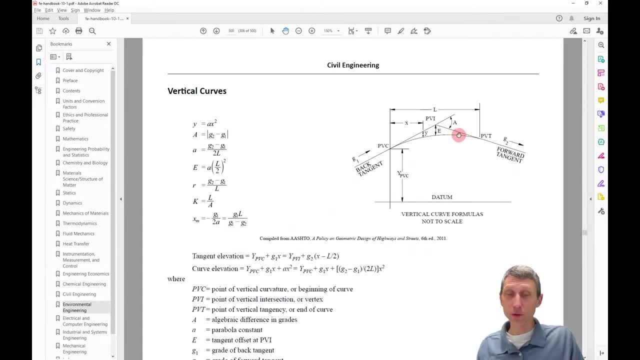 but that's going to be the top, That's going to be the peak elevation here, And if you really wanted to punish yourself, you could use this formula: take the derivative of it, set it equal to zero to find the X value, or it's going to be max, right. 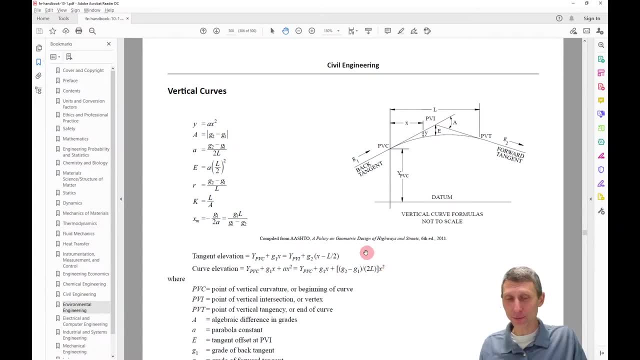 I mean, there's other ways of doing this as well, but basically that's. I mean, if you look at this formula here, right, That's kind of where. that's kind of where it gets to is, if you take the, you know the derivative of this. 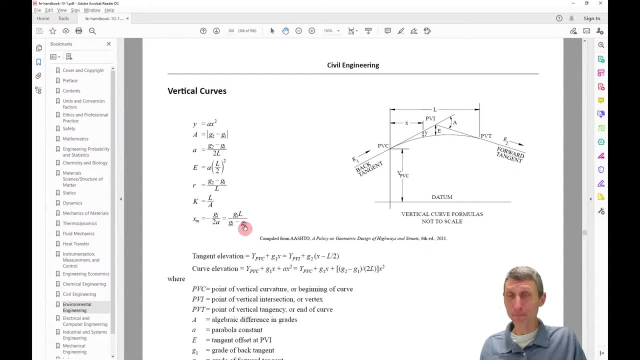 it's going to. it's going to work out like that, And so we don't need to find XM in this case, but we could find it if we wanted to. That would be another legit question that could get asked. All right, what's the crest elevation? 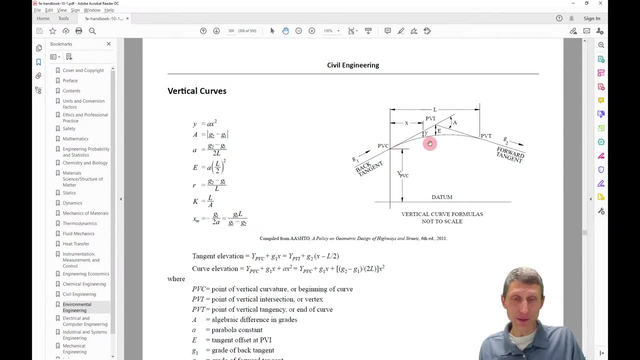 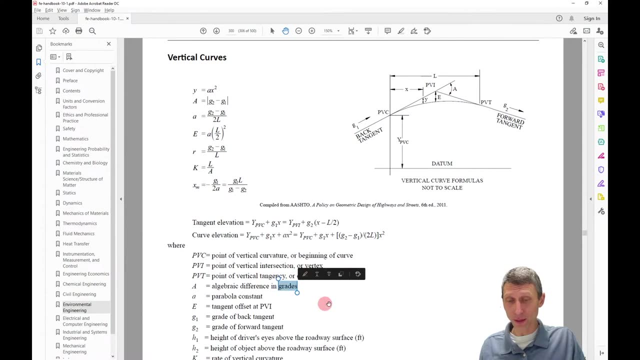 What's the crest elevation of this curve right? If you're given the point of vertical curvature, what's the crest elevation there? And you might be asked to find that. but that's this. you know. XM value down here as well. 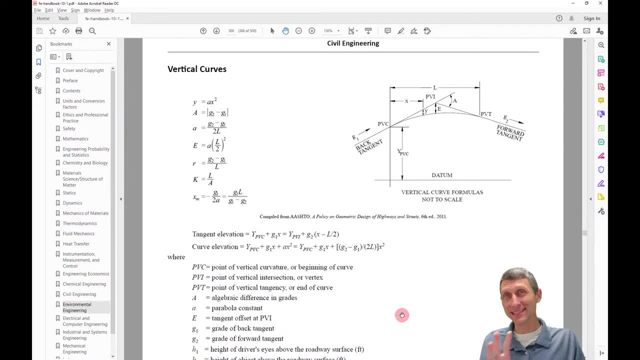 So another valid question, but again this is: oh, I wish we had time to do like a whole session on just curves, you know, but maybe, maybe we'll need to do that. come back to it, Let's keep going. 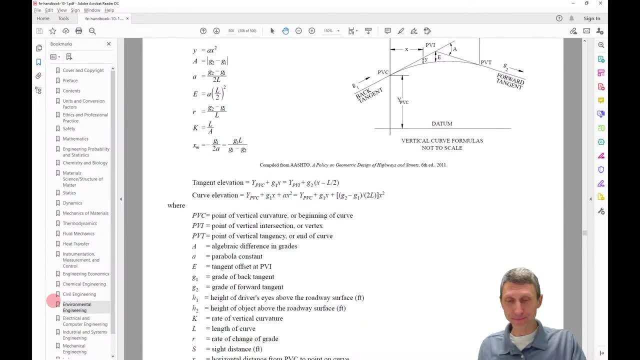 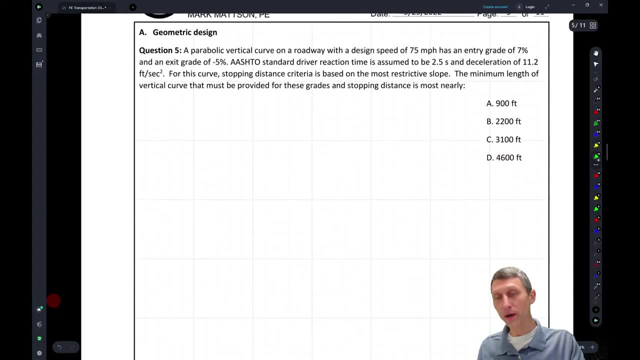 Okay, let's keep going And we'll go to question. We'll go to that. We'll go to the next question here as well. So the next question looks like this: We have a parabolic vertical curve and this is probably one of the more complicated questions. 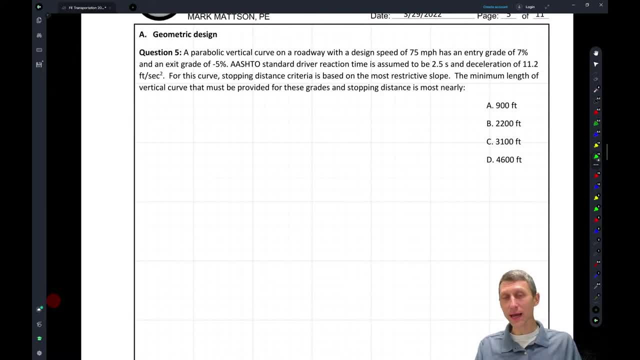 on vertical curves because it asks about stopping distance right. What's the point of stopping distance on a curve? Well, if you're coming up over the curve right And let me draw this curve in, So we have. we have a parabolic vertical curve. 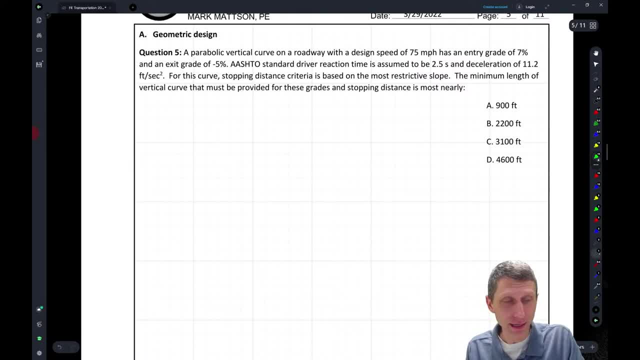 and a roadway with a design speed of 75 miles an hour. Man, this is like an interstate right And we have a 7% entry grade. That is like that's a super steep grade And I mean this is like continental pass. 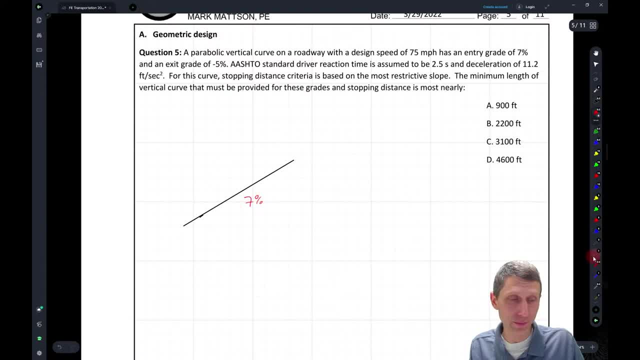 up in like the Rockies in Denver, That's like a pretty pretty steep, pretty steep- you know grade there- And then you're coming back down at 5%. So that's a little bit shallower here, right, Going up at 7%, coming back down at 5%. 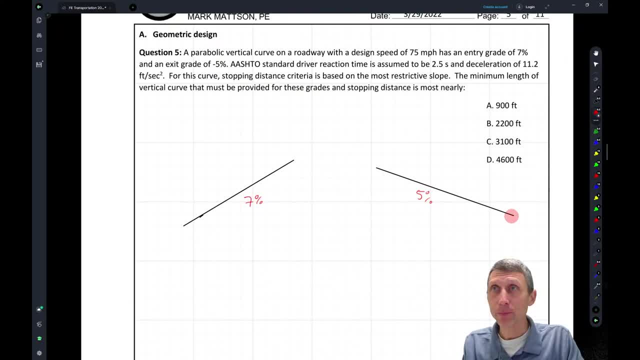 Okay, we have a roadway speed of 75 miles an hour. again, That's like an interstate, And what we're doing here is we have this curve that's going to connect the two, And when we have 75 miles an hour, this is going to be a big curve, right? 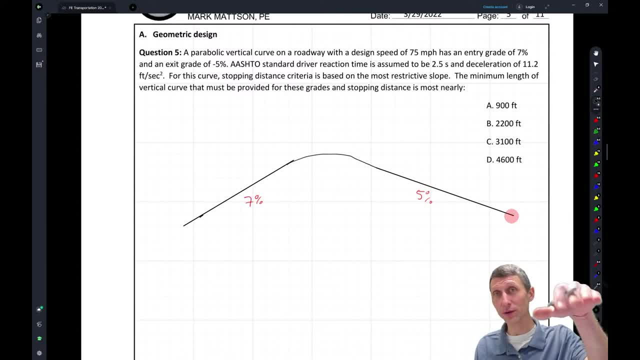 It's not going to be this little thing, And because interstates you're really gradual, because when you're going faster you feel it. So we have a standard reaction time of 2.5 seconds. deceleration rate of 11.2 feet per second. 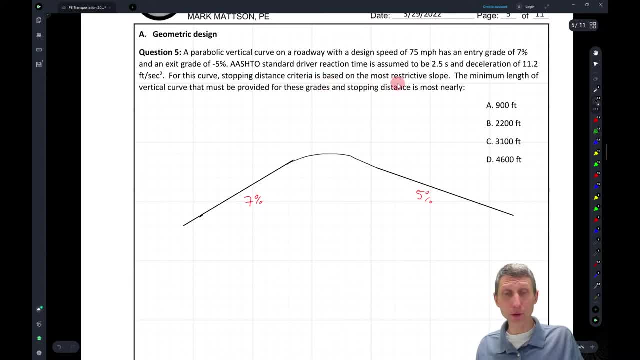 And we're told to do the stopping distance based on the most restrictive: the minimum length of slope, Okay, The minimum length of a curve that must be provided for these grades, and stopping distance is most nearly So. so why do we care about stopping distance? 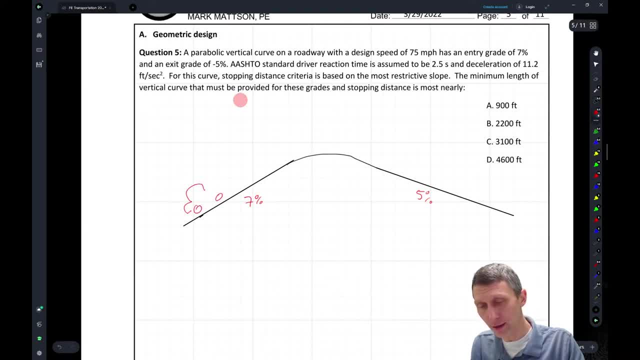 We care about stopping distance because as you get your car on here right- And maybe it's a truck with the- you know your RV in this and you got a big trailer here and you're holding something I don't know. 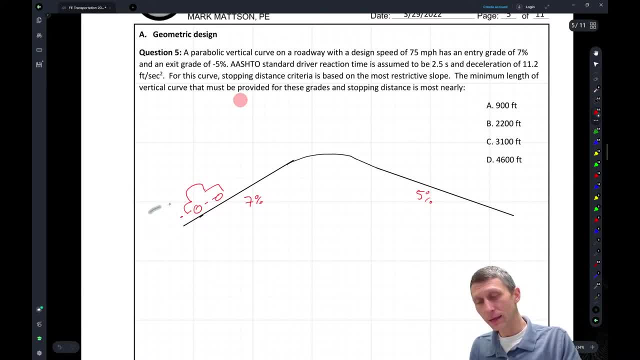 But maybe you're going up and over, and let's just say not that this would. let's just say: you know, a deer walks out into the middle of the road. Okay, A deer walks out into the middle of the road, right? 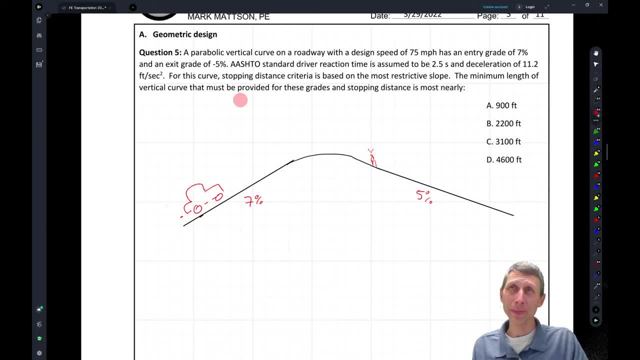 Sorry, not a very good deer, but let's say a deer walks out of the middle of the road. When could you see it right? I mean at this point, technically, you couldn't see that thing right. It's underneath the other side of the curve. 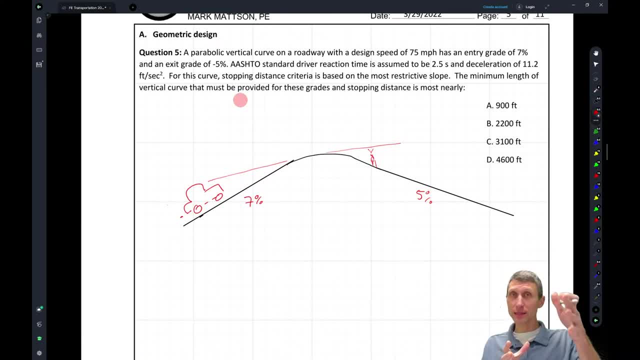 And. but what we want to do is we want to make it so that if there is something in the road- and typically it's a two foot height, but if there is something in the road, so deer is a little bit tall, but we want to be able to have enough time to stop. 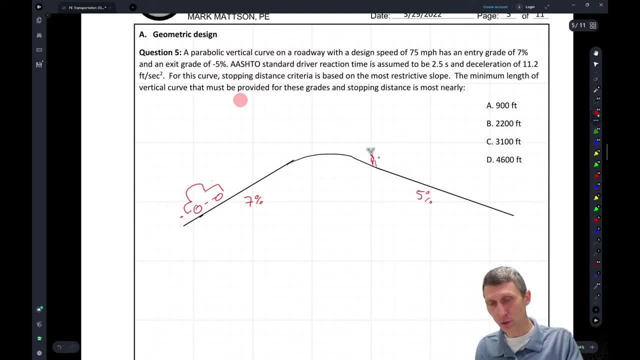 Okay, And that's where this stopping sight distance comes in. So what's that going to look like? Well, we have to figure out what that, what that distance is. So we're going to come back, We're going to take a look at our formulas here. 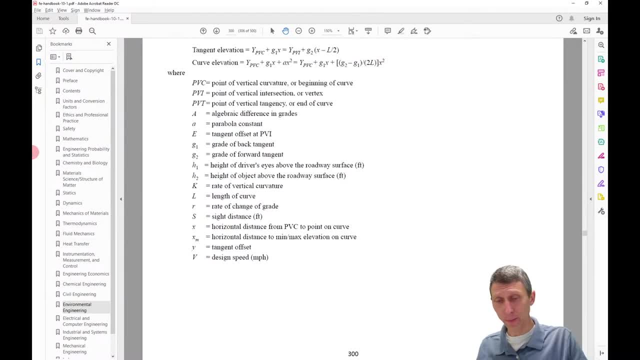 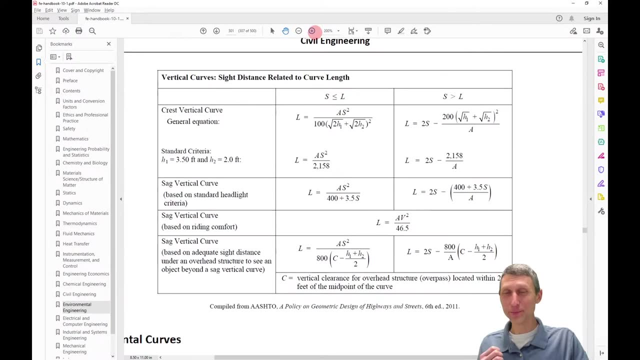 and hopefully this doesn't scare you, but there's going to be a lot of formulas and we're actually given a table, a table of formulas that makes it even more, more or worse. that's not really proper English, but it's worse than it could. 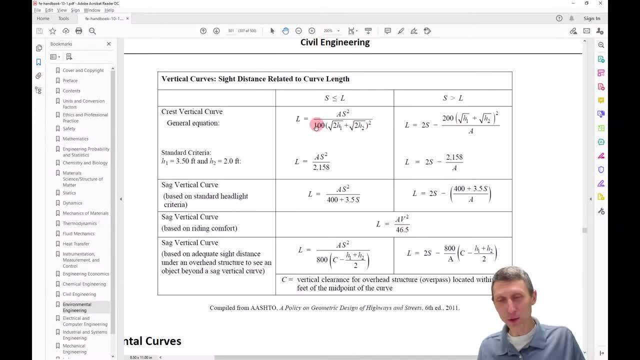 We, we, we even want it. We want it to be okay. So this gives us a whole bunch of equations, and this is you know. we have one side of S is less than L, and then we got a whole bunch of formulas. 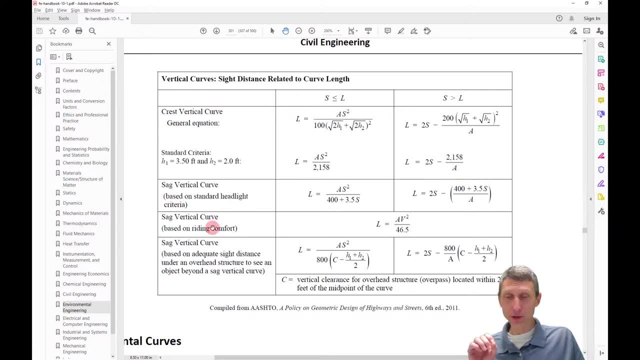 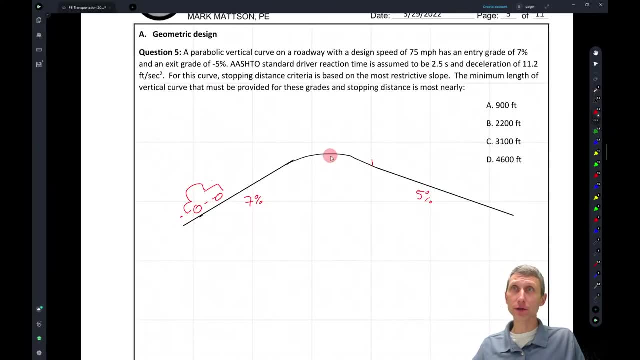 We have a S is greater than L. We have crest vertical curves versus sag vertical curves And the good news is we already know that we're a crest vertical curve. So the crest vertical curve we know because we have a positive entry grade right. 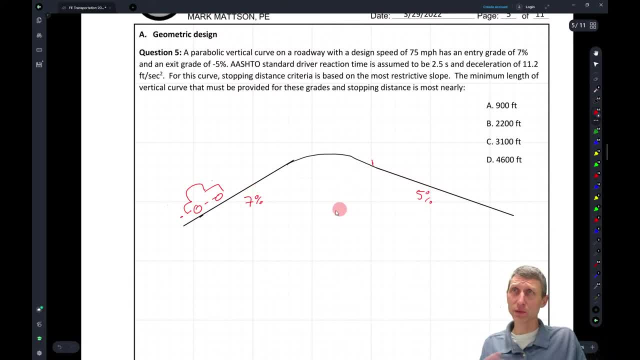 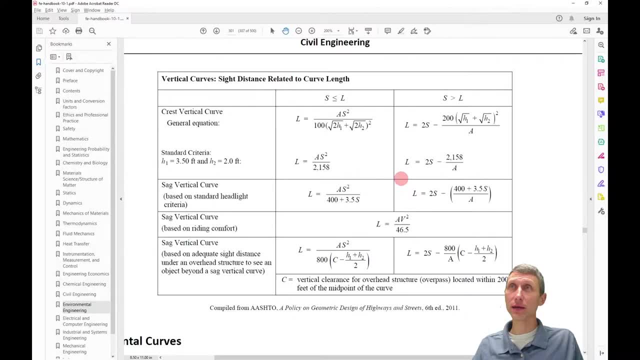 We're going up to start and we're coming back down as we as we go. So this is a crest, So that's kind of the first step, right, We know that. and then we have to say, okay, well, no, we know that we're a crest. 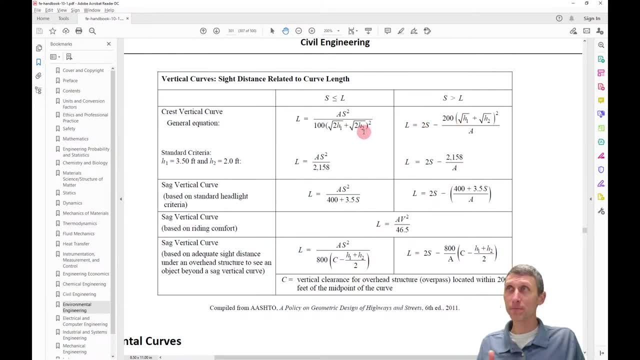 Now we need to know which of these formulas to use. okay, And which one to use is dependent on what S is and what L is. but we don't know what L is until we know what S is. So there's this chicken and egg thing. 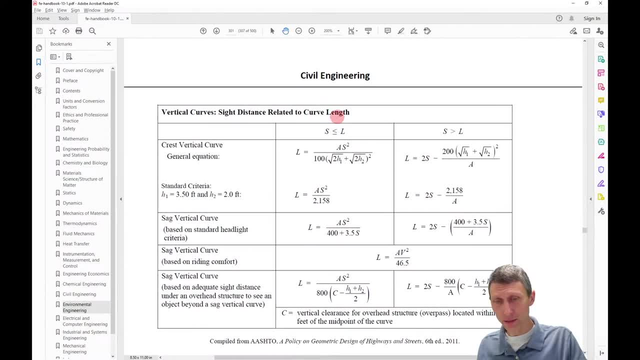 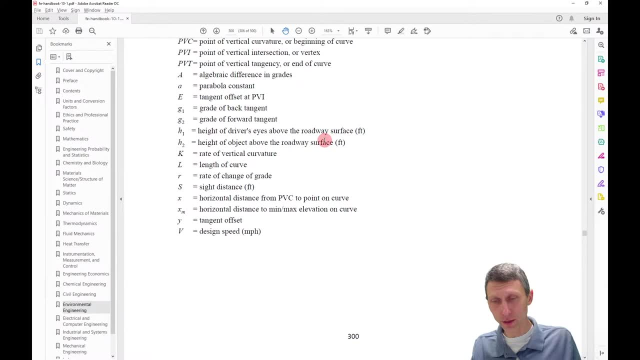 that we have to figure out here and we have to come back down. Actually, we have to come back up a little bit and take a look to see where are s is. so here's our s. s is our sight distance, and how are we going to find our sight distance right? 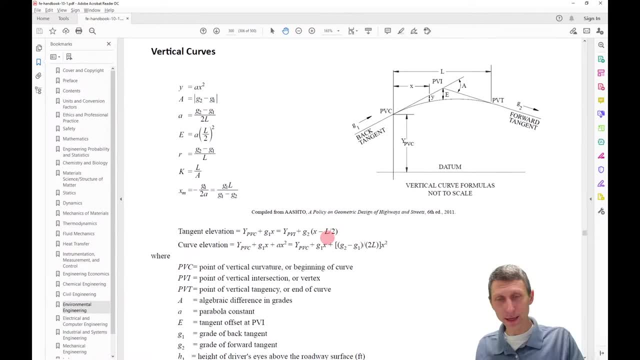 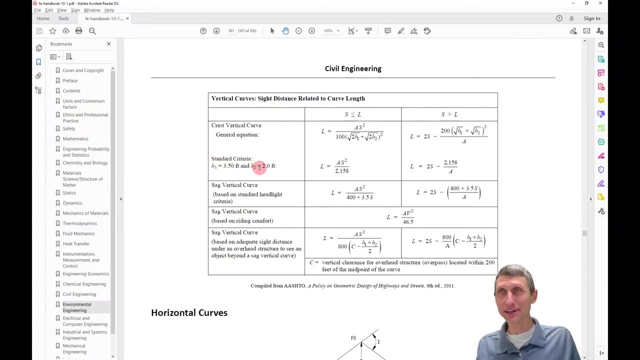 that's, that's. oh man, what is that? sight distance? where is it and how do we find it right? well, that's where we have to be able to go. um, we know we have our standard criteria here. this is for that. stopping remember the two foot two foot object. um, a driver height of three and a half feet. 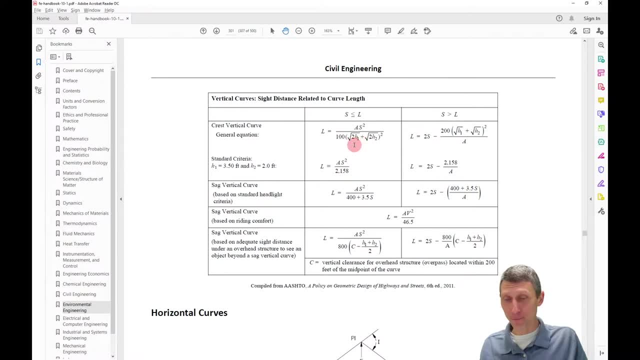 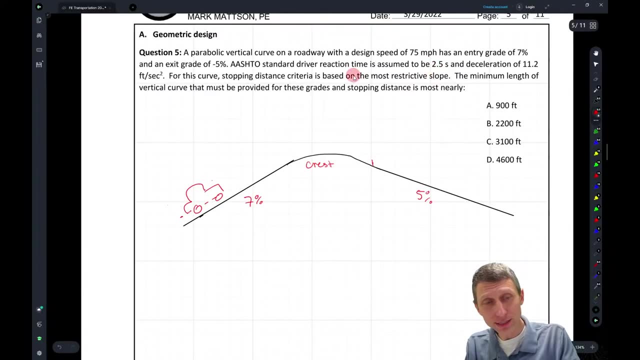 this s is going to come from the stopping distance. so anytime you're given in the question, if you're given, like the, the reaction time, right, this reaction time of two and a half seconds, the 11.2 feet per second, those things are gonna um, those things are gonna trigger in my mind. 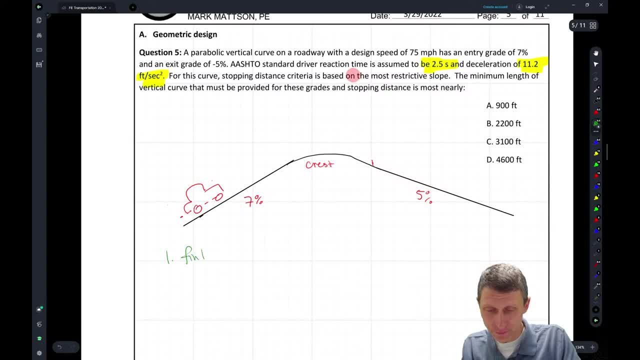 that first. what we have to do here is we have to find a stopping- you know a stopping uh sight distance. or stopping- you know sight distance here. so let's go find that formula as well, because in traffic engineering there's formulas for everything and so many of them are empirical that you just have to go look them up. so, uh, let's. 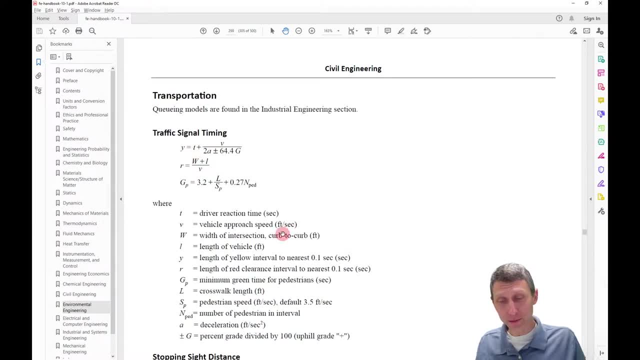 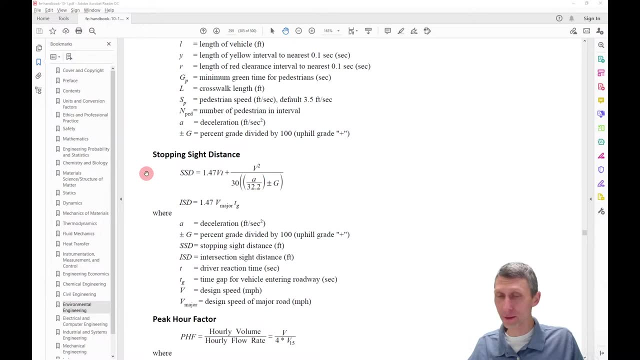 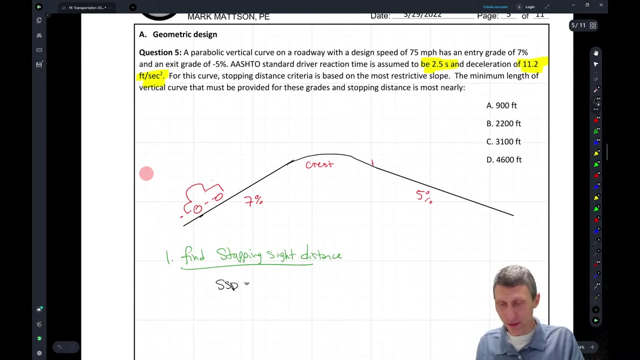 take a look and see where we go. we have our signal timing. that's not what we want, but here's our stopping sight distance and s is really ssd here. so we're going to take this ssd formula and come back over. so let me use that formula. i'll write it in here. but the stopping sight distance, or s in our 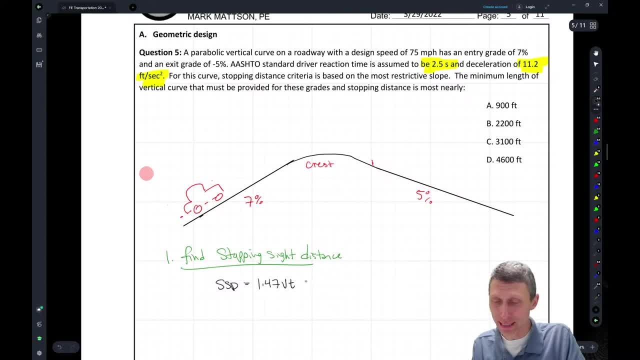 case is going to equal to 1.47 times vt plus v, squared over 30 times a, over 32.2 plus or minus g. and this is where some of these formulas- uh, you might have learned it a little bit differently and sometimes it's just sometimes- you might be given like a friction factor right. so sometimes, 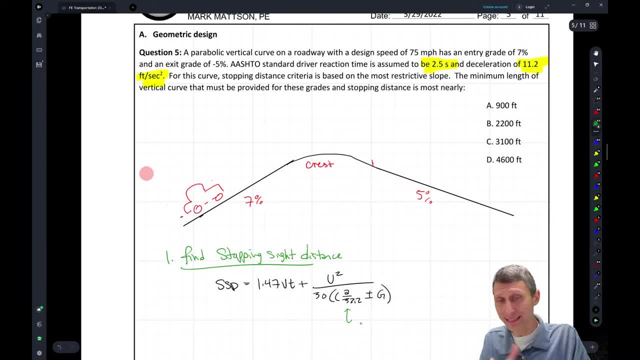 um, you'll, instead of being told that there's a deceleration, right, you might have some like friction in here, okay, and that friction is going to be on the order of like 0.3 to 0.35 um point in that range, right, but but in this case we're given the deceleration. 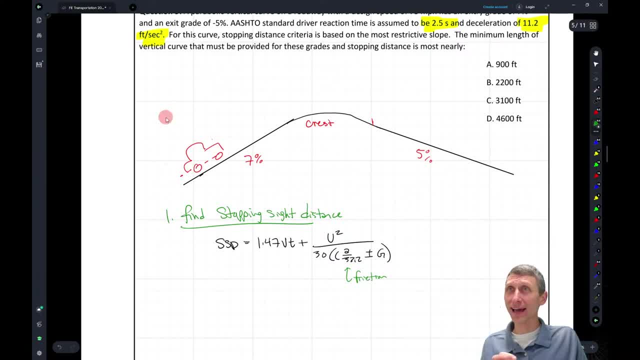 i don't know. i mean, maybe if there's somebody out there that's taken the test recently, i i think they're going to give you this reaction time. i think they're going to give you a deceleration, but there's a chance they might not. 11.2 and 2.5 are pretty standard reaction times for 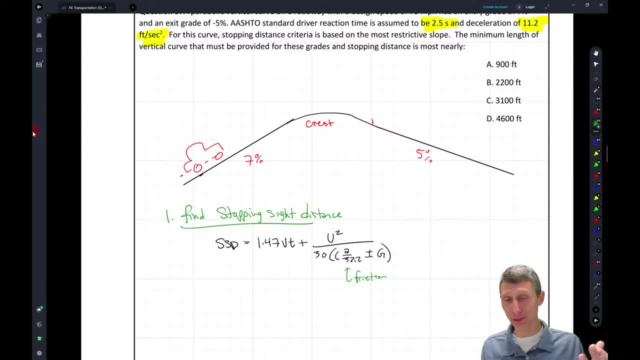 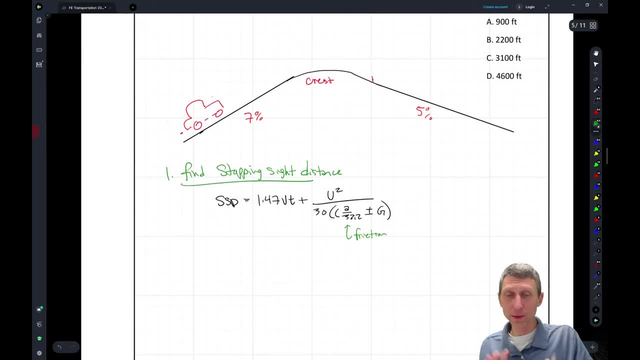 astro, it's possible they expect you just to know that, like they, you know some other things, but i i would think they'd give that to you. the other thing that you have to be careful with with this, with this formula, is just units, so i'm going to come back to the handbook. 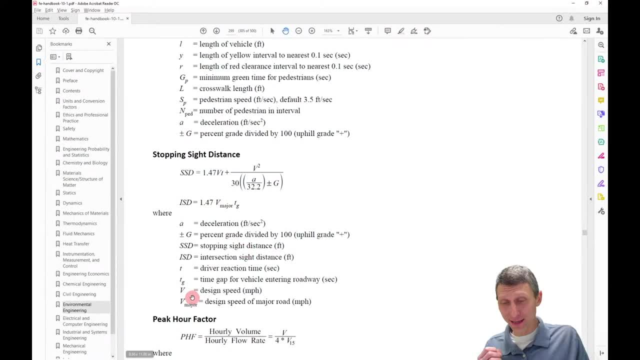 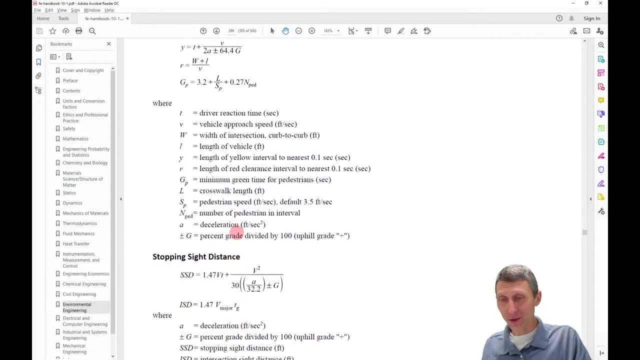 for a second. but units, um. when we're doing this, we see v here is in miles per hour, t is in seconds and you're thinking miles per hour times seconds. how does that work? it doesn't work until you have the 1.47. so are those, you know, going back matt to what you said? are those? are those numbers in here? 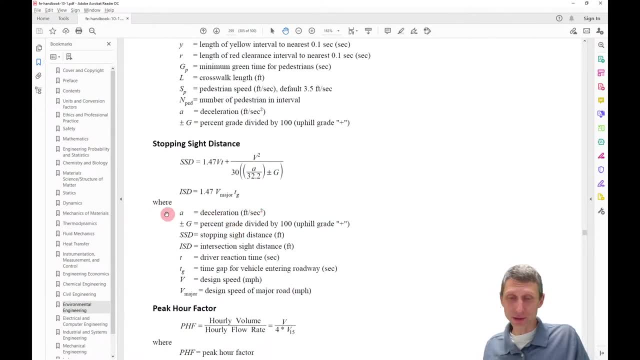 are those those um accelerations in here? this is the deceleration. a right, it's not. i don't see an 11.2 here, right, i don't see sometimes 10 is used. i don't see that here. i don't see the reaction time. 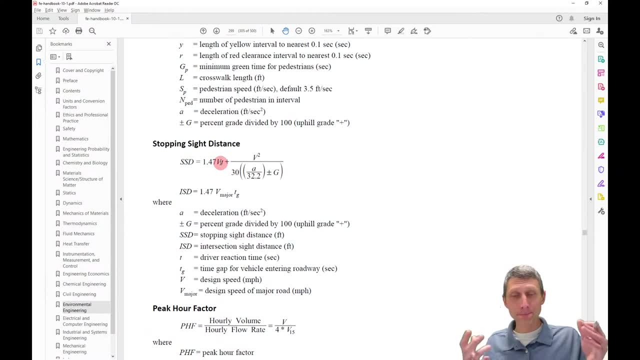 of t of 2.5 for an unexpected event. so i'm hopeful that that they would give that to you. uh, but maybe you could put a comment after you take the test, like no, they didn't give it to me, i, i don't know. like um, i i don't know, but that's you know. the the time is typically one for like a. 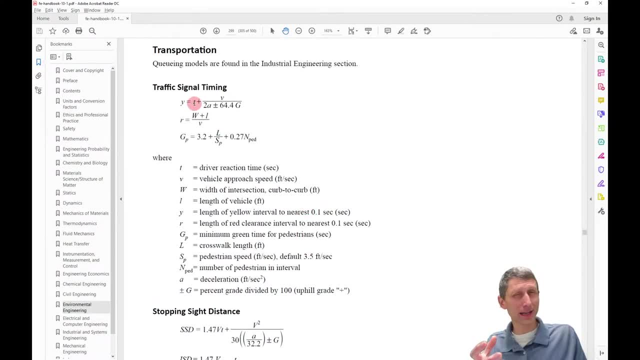 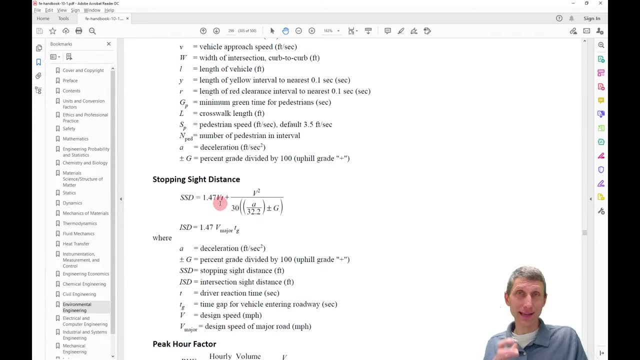 bent like, for example, a yellow signal. you expect it to turn yellow. it's been green for a while. that might be one, because you're ready to hit the brakes, whereas something runs out in the middle of the road. you're not expecting that it takes a minute to a second to figure out what's. 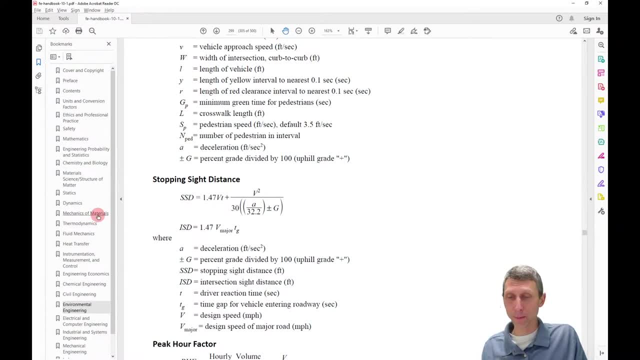 going on. that might be like two and a half seconds till you finally hit the brakes and do something, um whether you're gonna swerve or stop or check around you or what's going on. so those times you gotta know. and then g, here is. g is another one, which is: i think they do a decent job here of 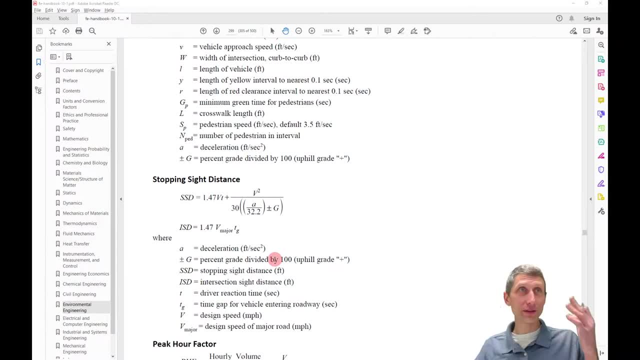 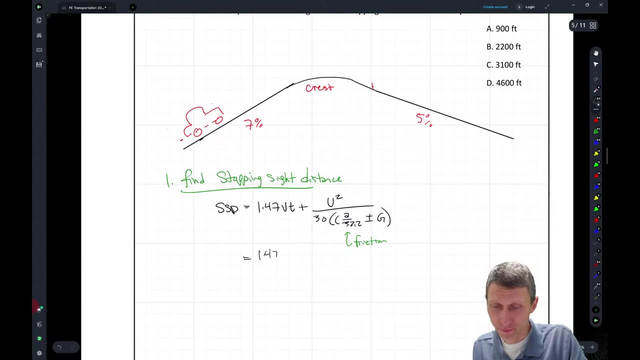 so they, they tell you that you're going to use a decimal. so once you get those units down, it makes this a little bit easier. but what we're going to do here is we're just going to plug those in and we're going to say 1.47 times v, which was was our design speed. you know, again, this is like a. 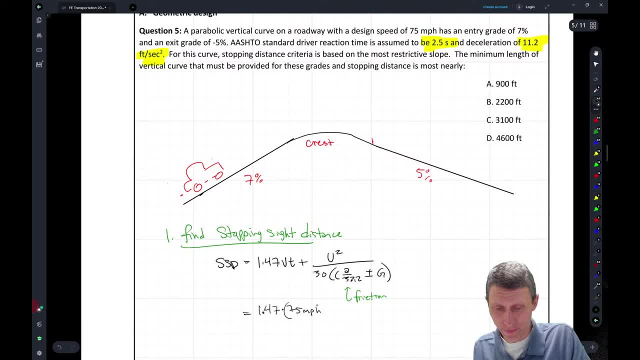 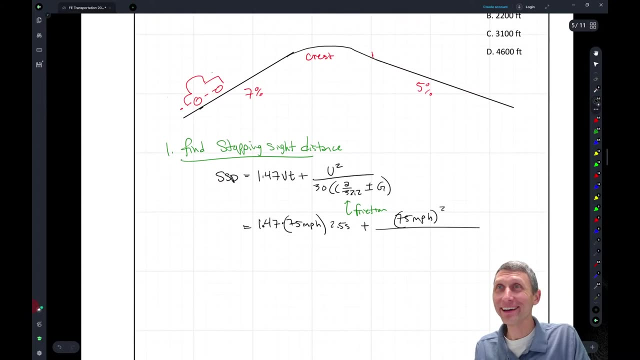 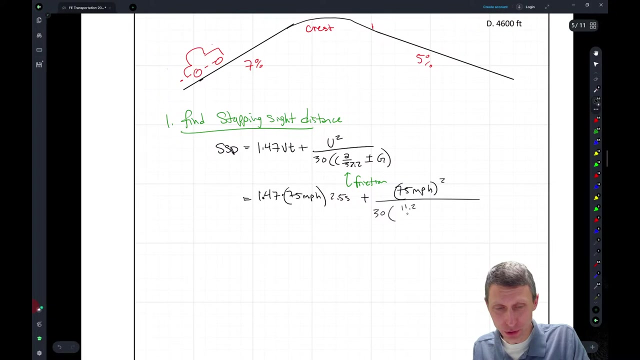 this is like a interstate: 75 miles per hour times t, 2.5 seconds, plus what's v squared. v squared is 75 miles per hour squared, sorry, squared divided by- uh, let me make some more room up here- but 30 times a, which is 11.2 over 32.2. so again, that's your i. i could write feet per second squared in there. 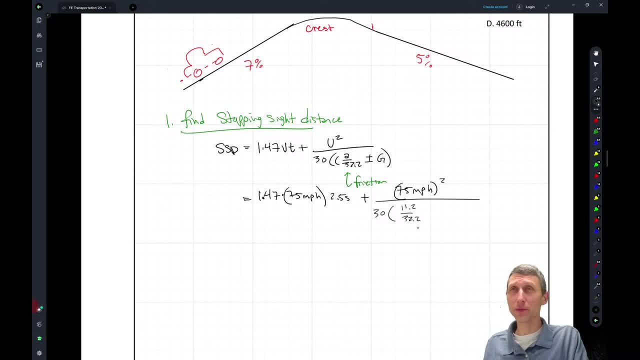 but um, what's 32.2? do you remember? 32.2, that's feet per second squared, that's gravity. that's that's in. um, that's that's english. you know units, that's your american standard unit. so that's, uh, 32.2, two feet per second squared is gravity, uh, and non-metric right. and then we're going to add: 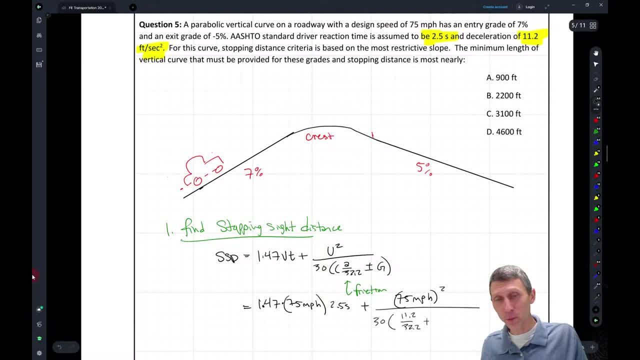 in here the grade. so the question is: which grade do we pick? right, we're told the most restrictive slope. um, so in this case, which? where is it going to be harder to stop? it's it's going to be easier to stop going up a hill. it's going to be harder to stop going down the hill. okay, you're going. 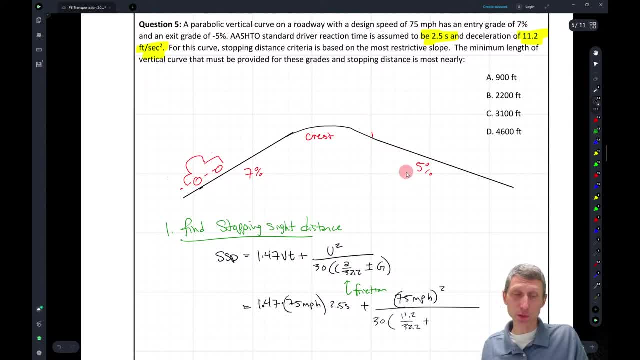 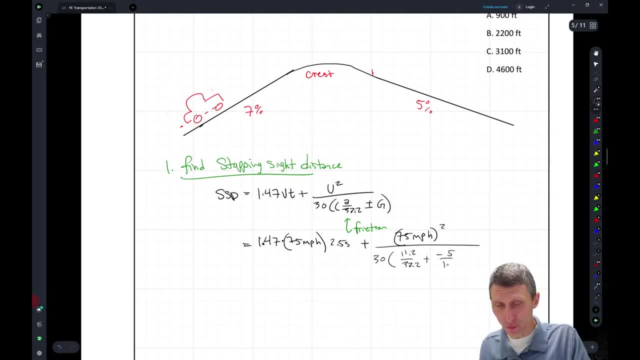 to have gravity working for you here. you're going to have gravity against you here. so that's where. that's where we're going to come in here and we're going to put this, you know, negative 5 over 100 in there to get our slope. so if we put all that in, we get a stopping site distance and 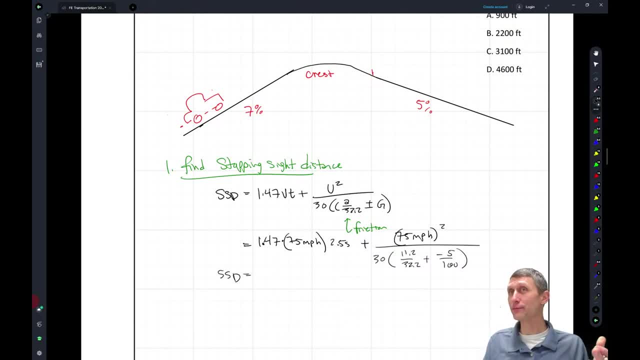 this is going to be a pretty long stopping site distance because 75 squared is a pretty big number and the number that i got was, i think, 905 feet, so maybe somebody could do that. check me on it, but it's a big, long equation. hopefully you can make that work. 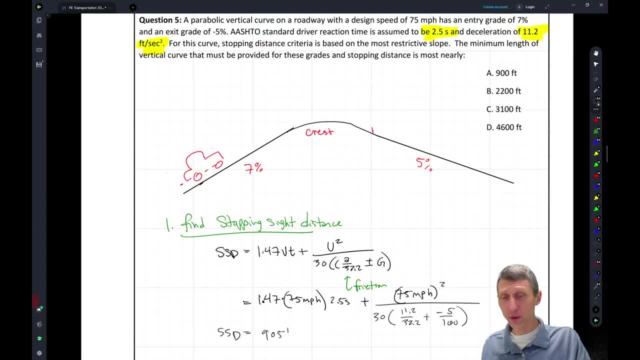 in, in, um, in what you're doing. so if that was the, if that was the question, that'd be great, but unfortunately that's not the question. we have to keep going and find our um, our length of curve right. we have to keep going, our length of curve. 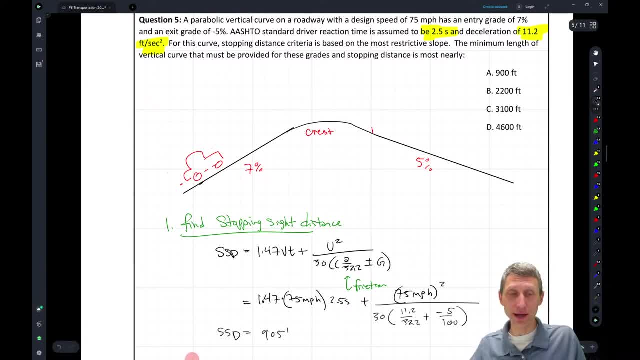 yeah, yeah. so good question: why not just subtract it 100? you could i just put it in there to try to remember that this started off as a negative grade. i mean, this is a plus or minus here, so it's you know you could do it either way. um so let's come back to the handbook, though, and 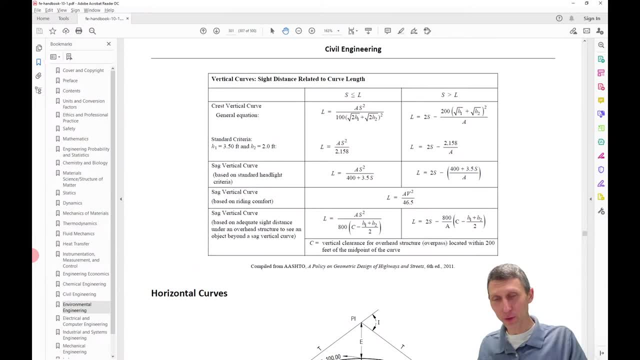 take a look at our, at our curves and our in our formula here. so s is less than l. well, again, we don't know what l is. so how do we know if s is less than l um? we, we don't. so this come be this kind of works out to be a little bit of brute force, right? so we have two equations. we 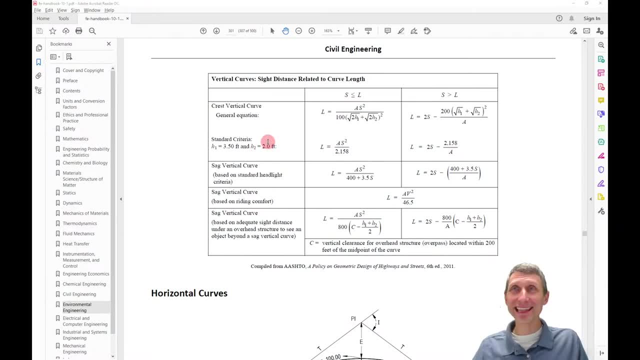 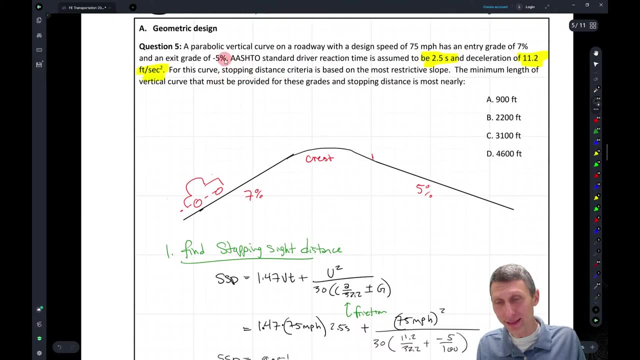 have a general equation and a standard equation and in this question i think did i tell you i, you know i, i don't think i told you i. i think i said standard driver reaction times. this curve stopping site is on the restrictive slope, minimum height of the vertical curve: that. 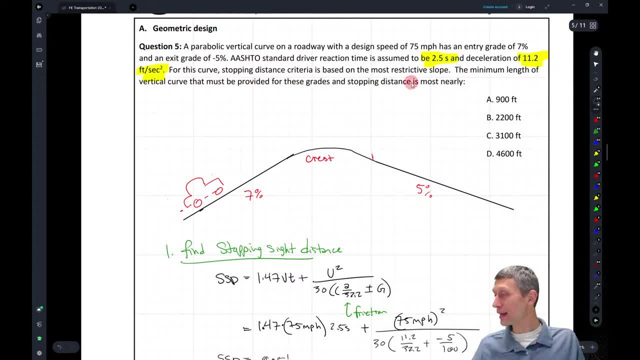 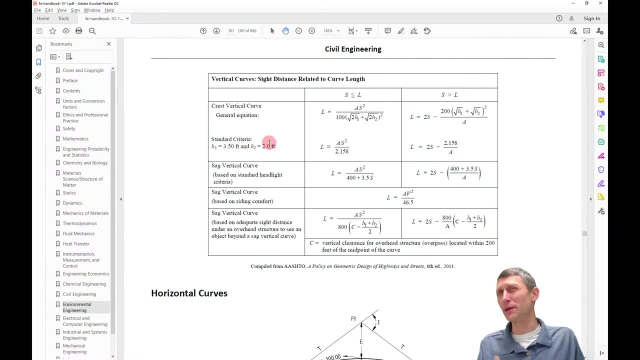 must be provided for these trades. i didn't tell you that it's, that it's the standard ashto standard, but if that's not told, it's probably going to be assumed. i mean, the the ashto standard is pretty typical. so if it's not, if you're told something else, i'd say use whatever else they. 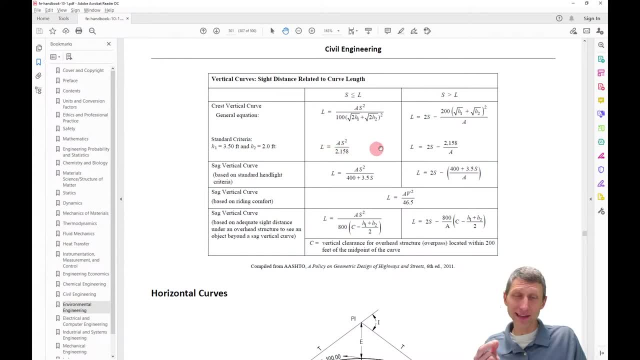 give you, if they don't, that that helps us a little bit, because now we can boil the down to these two equations and see which one works. so to do this, you're going to start with one. you're going to make an assumption. right, we're going to assume, we're going to assume. well, 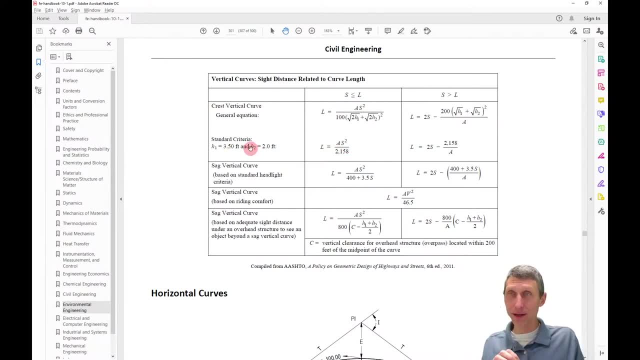 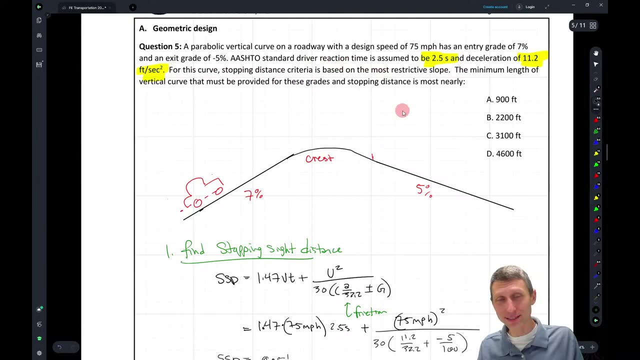 i said the standard reaction times, which is a little bit different than the standard um site distance height. so it's- or maybe i didn't, i don't know- standard reaction times. i could say i could probably add in here um reaction time and astro standard, you know. stopping. 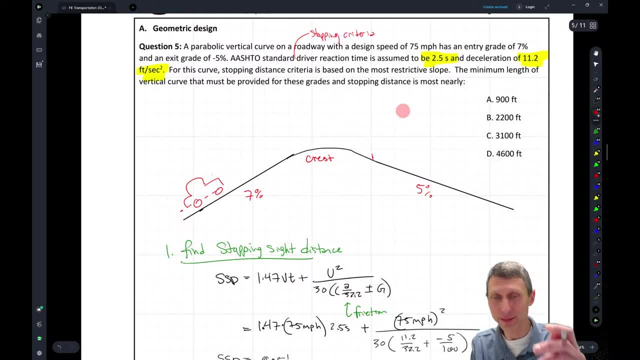 uh, criteria, uh, you know, like something along those lines- and and and reaction time, so i could add that in there to make that a little bit more clear, but let's, let's go with it. so what we're going to do here, though, is what we're going to say. is we're going to say, you know, to find l? um, we're going to you. 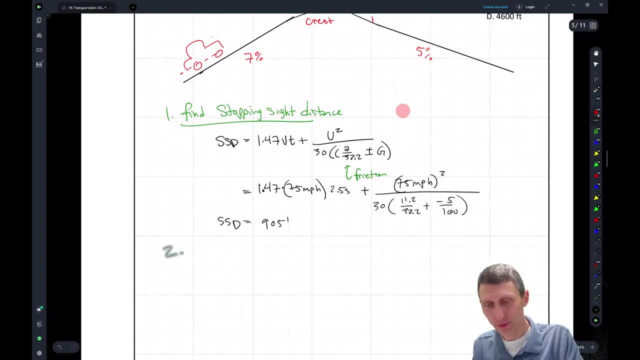 know for step two here, come on, i want green. there we go. we got green. now, um, for step two, what we're going to do is we're going to assume that s is less than l. that's going to allow us to solve this right. so if we assume s is less than l, 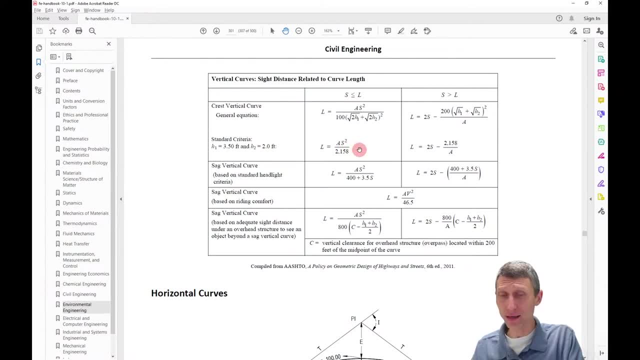 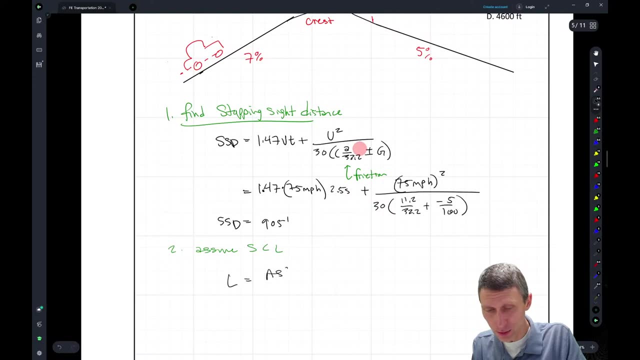 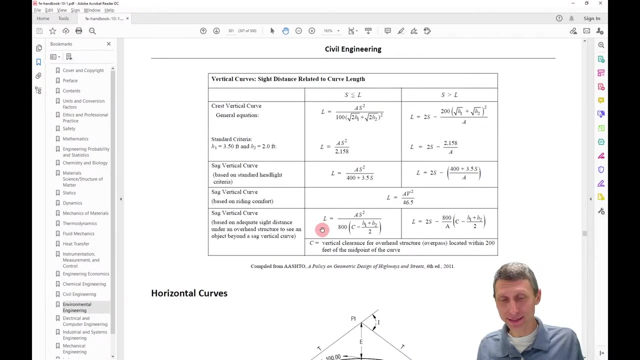 we're going to say. we have this formula here now: l is a s squared over 2158. so let me just write that in one. in it, the length is equal to a s squared over 2158. what's a right a is is what a is. 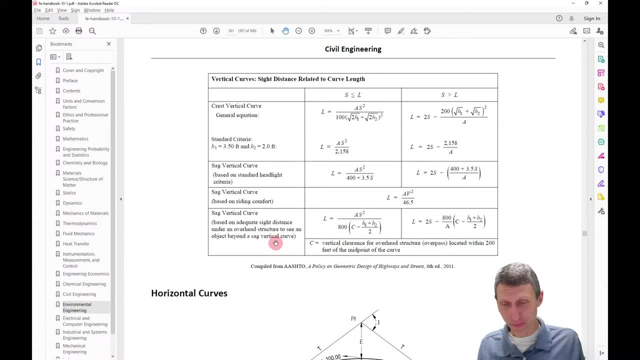 where is a a a a, come on, it's in here somewhere. uh, there, is it not in here? it's got to be in here, um, or is it up further? it might be up further. i know i saw it in here just the other day. i was. 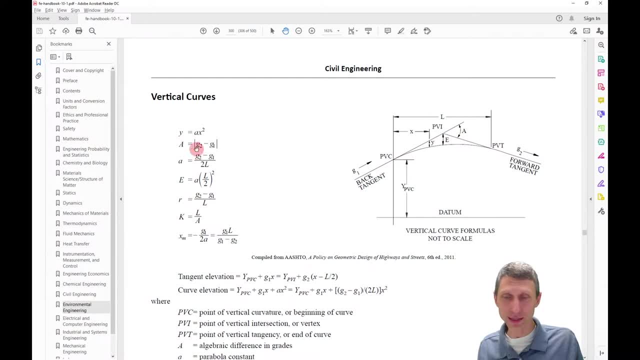 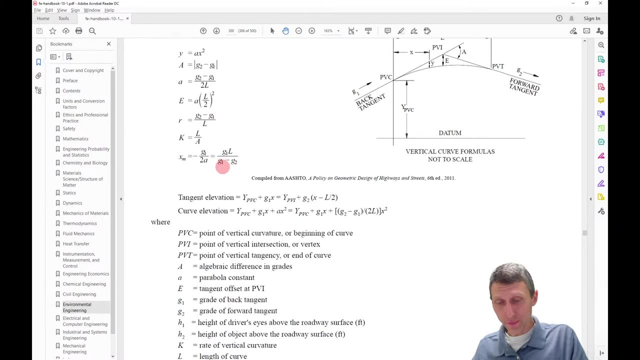 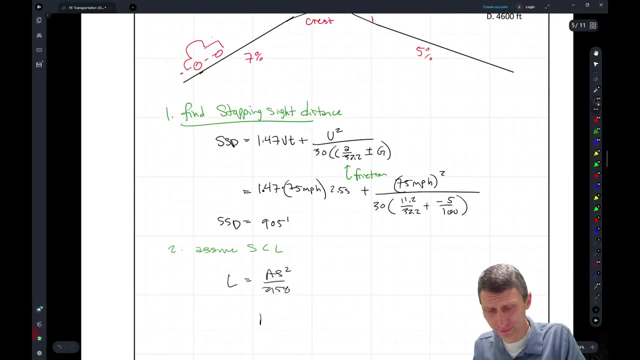 i was just checking these problems. a is the algebraic difference between the two grades, the absolute value. that, uh, the difference between the two grades. so, um, you know that's the algebraic difference in the grades. we can find a right. so we know that a equals i can't. 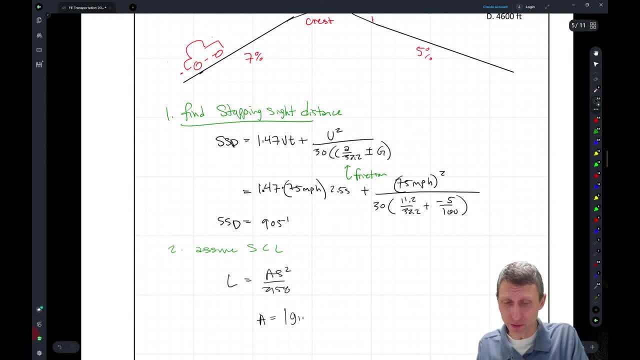 remember if it's g2 minus g1 or g1 minus g2, but it was the absolute value, so it doesn't really matter. um right, so a is going to equal g1. what do we have? we have 7 minus minus 5.. so that's going. 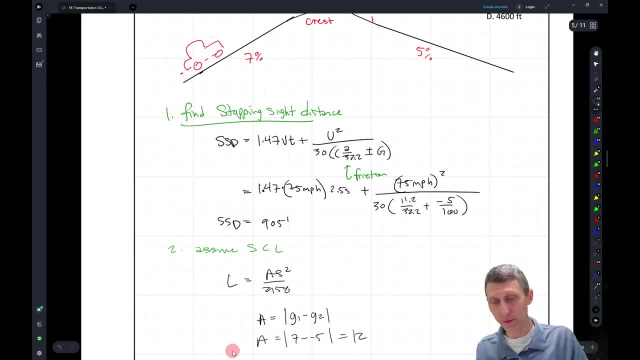 to equal 12. right, the absolute value of it's going to be our grade is going to be 12.. um, so we're going to come back here. we're going to say 12 times what's our stopping distance? 902.5 squared all over um 2158, and it's going to give us some value here. so that value, 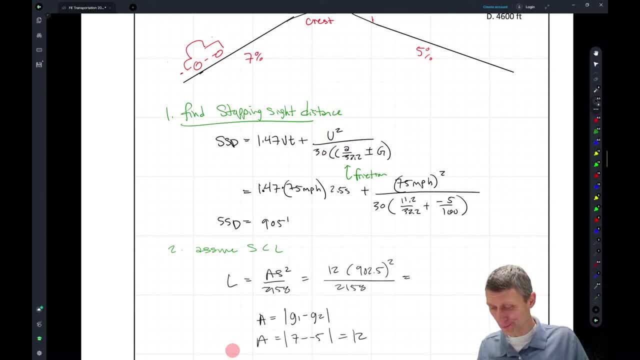 is going to be big. it's going to be, um, i think i got like 4 500 right, so like 45, 56 feet, so it's a big long curve, uh for a big, uh, you know, a pretty fast road, um, but yeah, it should be 905. i think it was 905.2. sorry, that's what i have in my notes actually is 905.2. 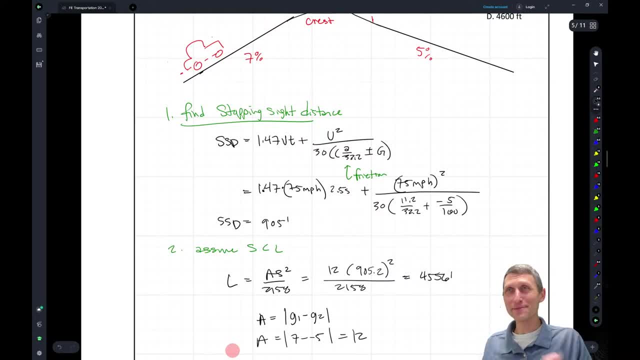 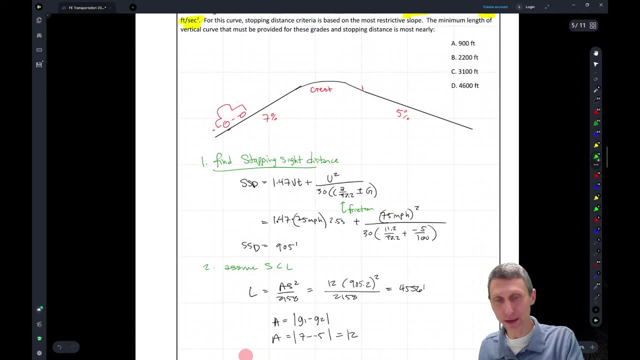 you guys are gonna have to help me tonight i'm i'm checking too many computer things trying to make sure that we're not we're not too screwed up here, but i think that works and it gets us back to an answer up here. so big long curve, um, you know fast. 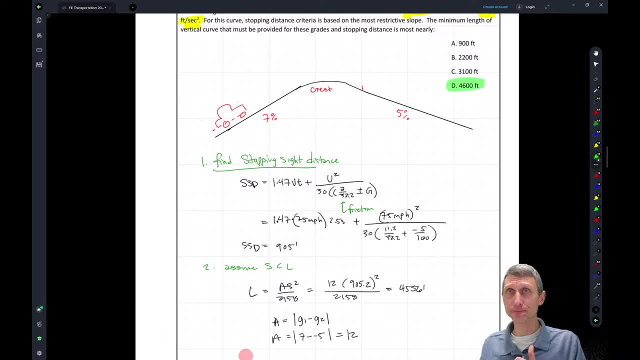 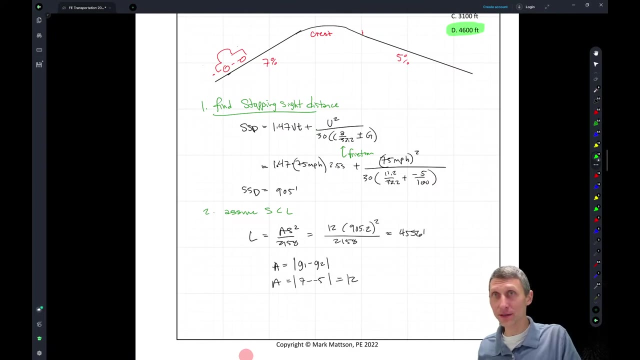 fast road, steep, slopes and um, all those things combine um to make it big, okay. so i think that works and let's keep going. um, yeah, thanks for uh, thanks for pitching those. those uh answers, okay, let's, let's keep going. so, curves: um, you know the curves again, if we come back to our formulas here, 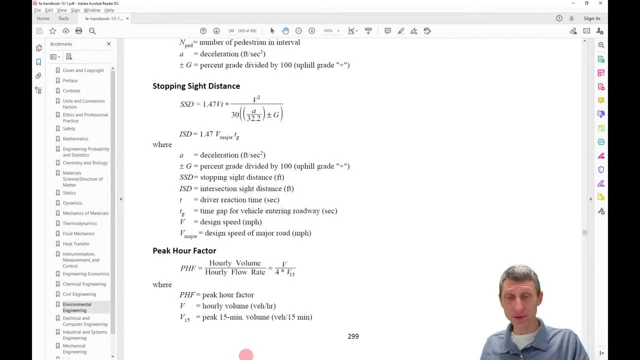 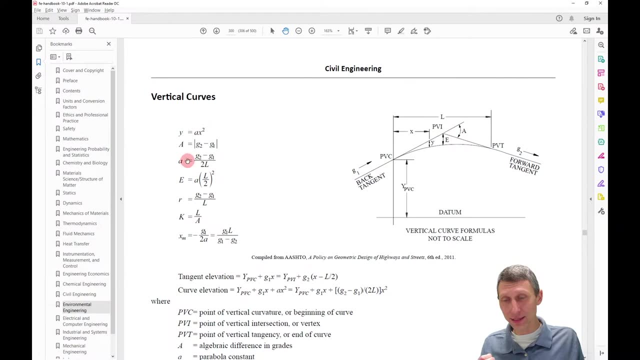 we have. we have certain pieces that we can deal with with curves. stopping sight distance gets thrown in kind of in a bunch of places, um, it could get thrown in with curves. we kind of need to know these different pieces here where we have our, our grades, um, and 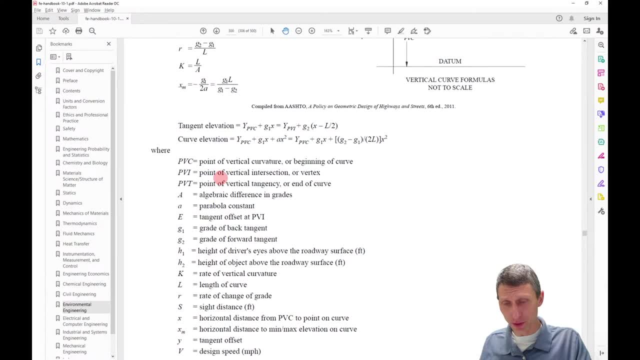 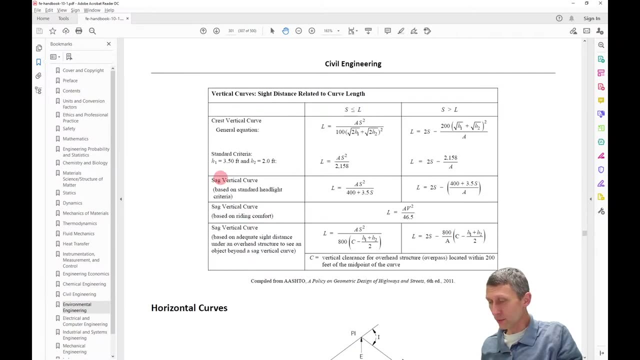 and um and how, how this, this works. so i i think i think we're good now. now i'm actually curious about one thing here. i and i want to just double check one thing: give me, give me two seconds um, because i want to make sure i don't screw you guys up too much, because i'm gonna. then i'll get comments and you know. 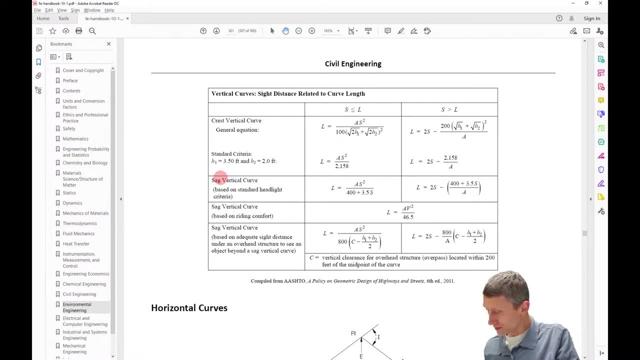 you guys all hate me, but that's okay if you hate me. as long as you pass the fb, i'm happy. and uh, hopefully i don't screw you up too much. um, let me just check one thing in here and uh, you know what? i'll have to check it later, so we'll come back to it. um, and it's okay. 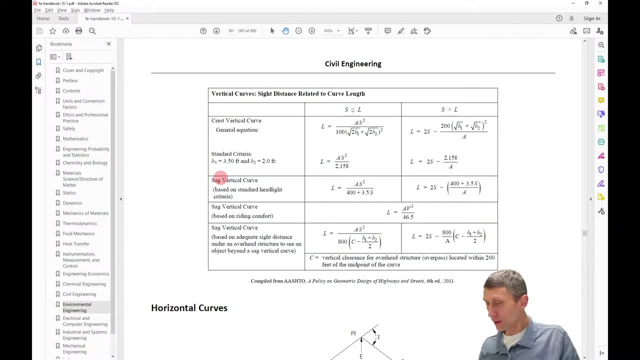 okay, let's, let's keep going. actually, give me two seconds. there's always this: you know this interesting thing when there's um down time for a second, because people are like what's going on? you know what. i'm also hoping that you guys will give us a story, for uh, the story, and i wanted to. 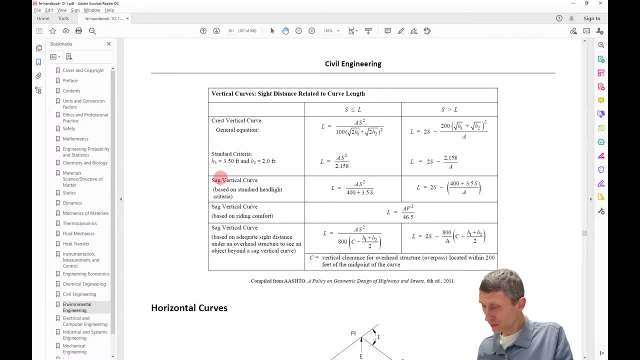 make sure. i talked about it earlier on and you know it's okay, we can make this work. but, yeah, i think i think we're good. okay, all right, let's keep going here and, um, i'm happy if you're happy. i think the only thing that i 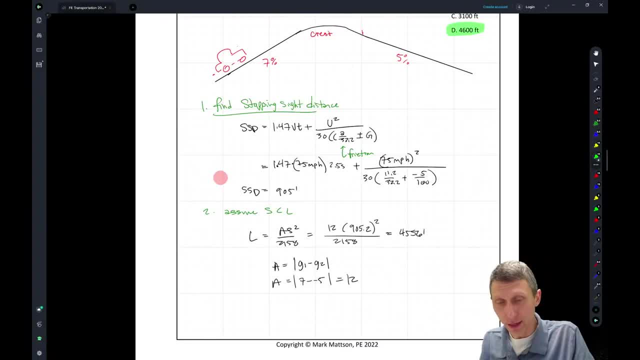 forgot to do here, um was to just double check that our assumption was correct. so s is less than l, and if s is less than l, let's double check this, right, because it so. so now let's check our assumption, right. that was: s is less than l we have. s was um. we would have. s was 905, that's. 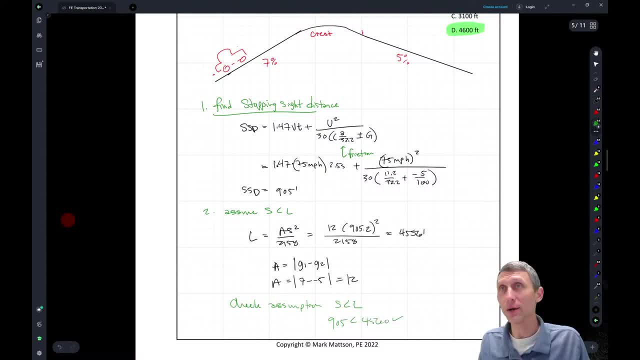 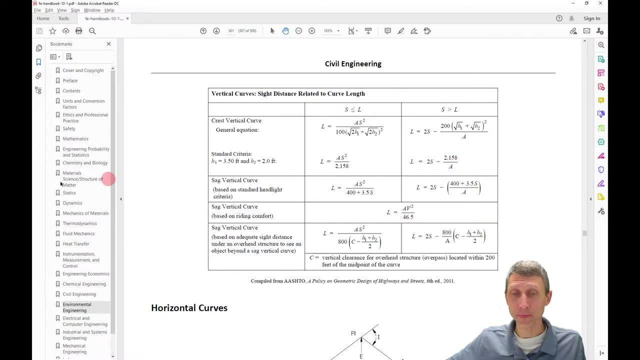 less than 40. you know 560. that checks out. if it doesn't check out, what do you have to do? you have to come in here and go to the second equation? okay, you have to go to the second equation, but then you don't have to check it because you already know what's going to happen. 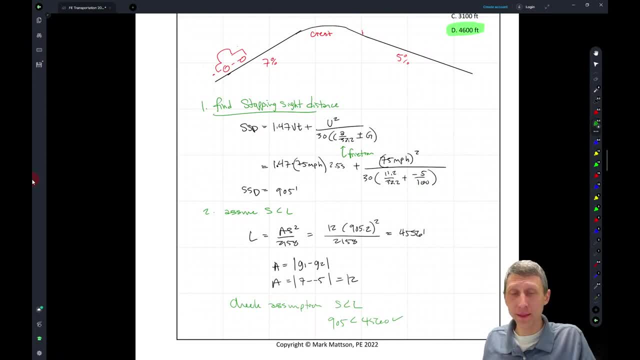 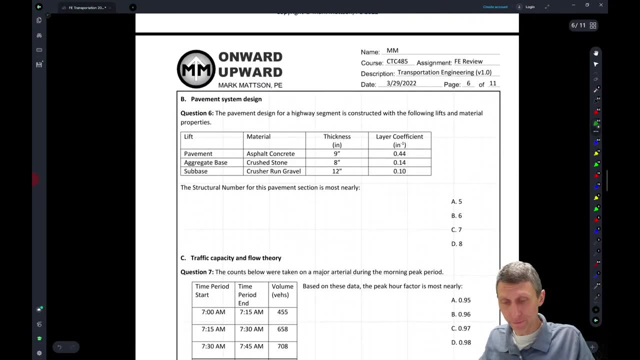 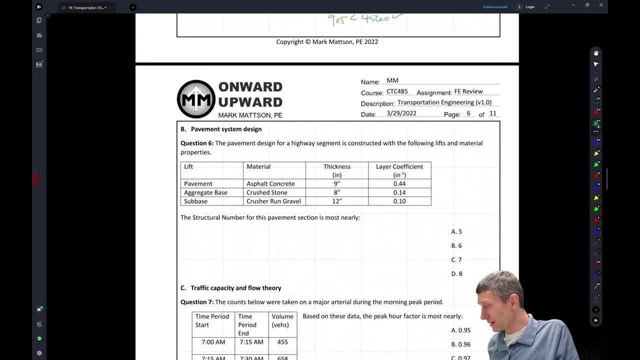 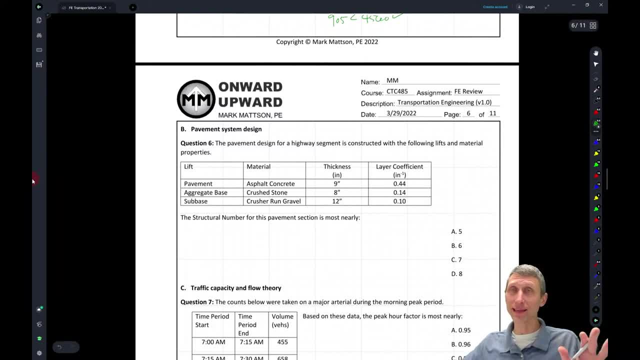 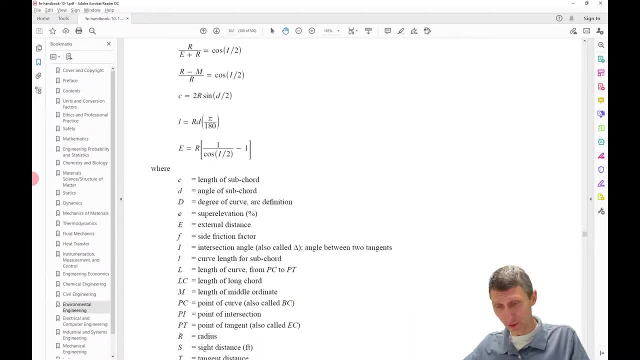 i'm pavement design. here there's not a ton, i think. i think if you get a pavement design question, it'll either be pretty straightforward in terms of um calculating like a structural design number or a thickness of a course. but as we look at the um, the reference handbook here, 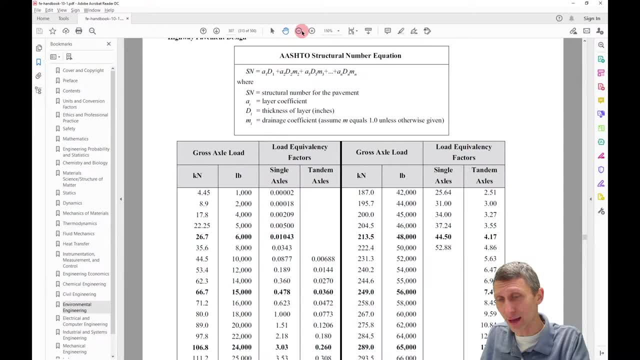 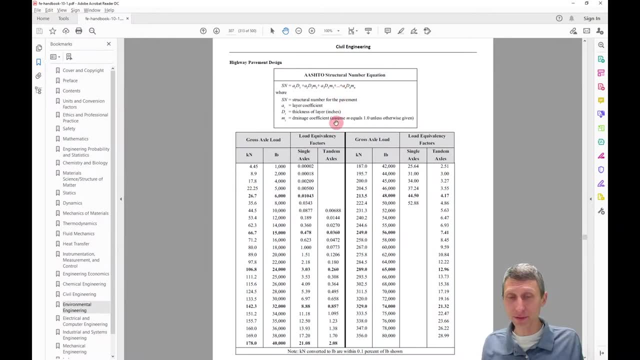 there's, there's this one page on like on highway pavement design, and it has structural number. so there's this one formula. i'll do a problem with this one formula. and then there's equivalent, you know load equivalency factors or equivalent single axis loads, and you could be asked for an equivalent load, the tandem axles, that's two axles per one. 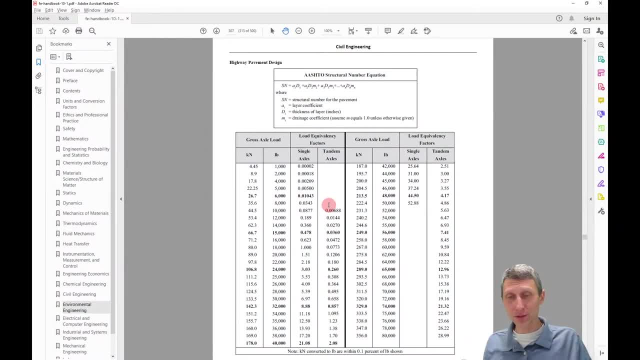 kind of thing. so it's like you could be asked to do some of that. but i mean, i just took a structural number one here. um, i think these might be some conceptual things as well, in terms of, like, maybe you're going to have: well, what, what goes into a pavement? well, there's the top course, right there's. 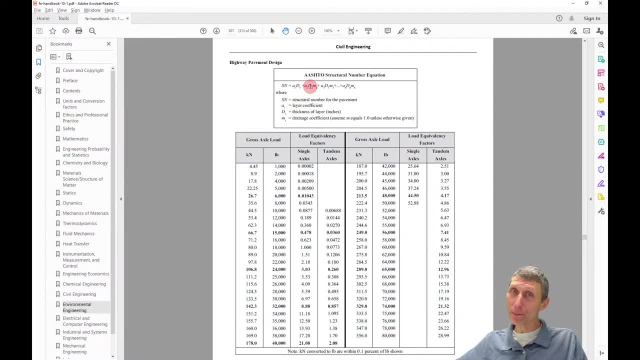 the, the binder course. there's a base course, there's a sub base course, there's a sub grade right and typically you're going to have a sub base course. there's a sub grade right and typically you're going to have a sub base course. there's a sub grade right and typically the sub grade is what's. 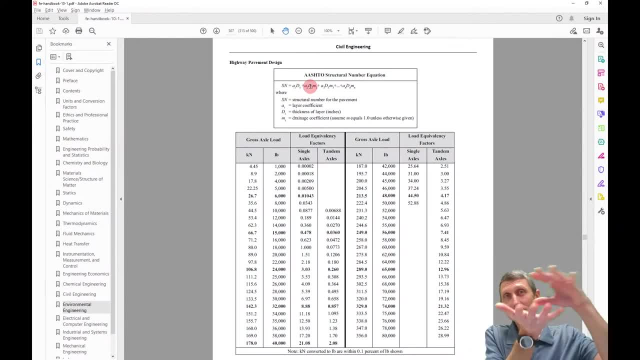 already there and then you start building it up with stone, and then you start building it up with coarse asphalt and then you get, you know, less coarse asphalt at the top right. so where do we, where do we go from there? i you know, i think this could be a conceptual question. it could 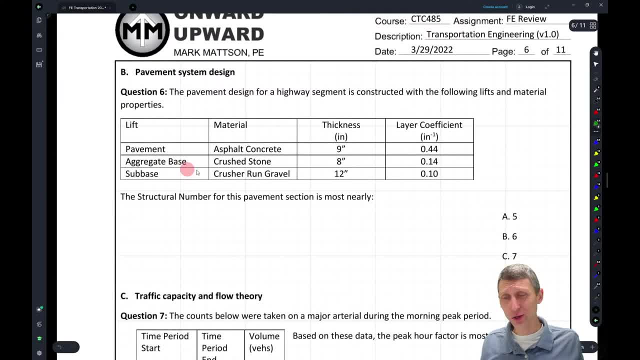 be something as easy as this, though, where you're given some, some courses and you're told to find a structural number, right. so if that's, if that's what it is, this is great, because this is kind of an easy, easy-ish question. but the structural number: you're told to find a structural number. 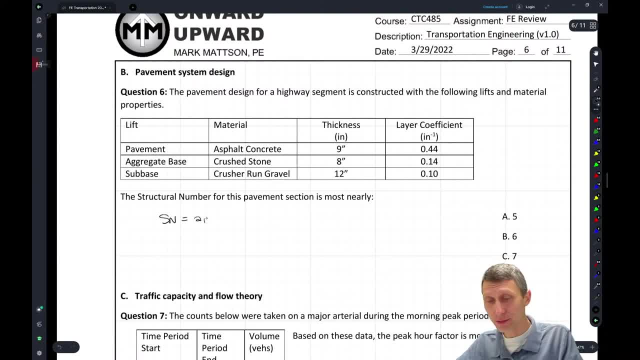 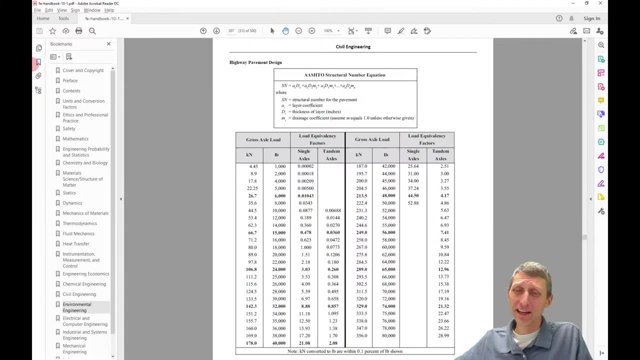 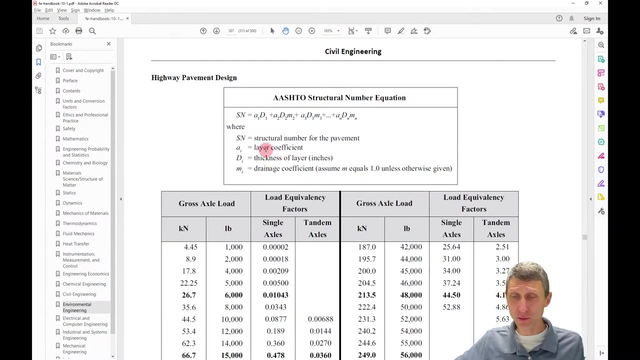 is just equal to a1 times d1, okay, plus a2 times d2, plus, you know, a3 times d3, and it would keep going if you had more layers. but, um, right, so this is just one of those formulas where it's not super crazy, it's not a super hard formula. you just have to know what the things the layer is and what the 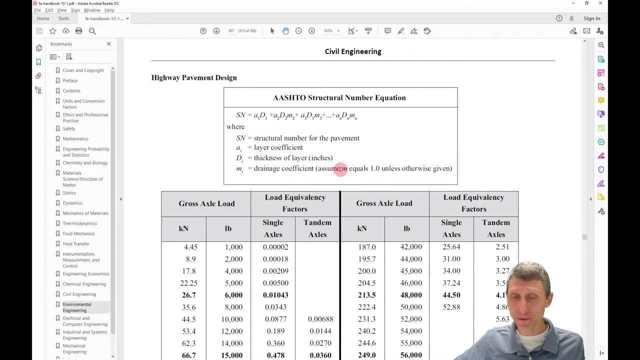 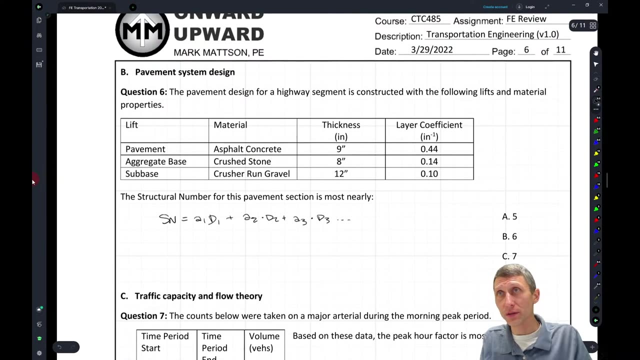 layer coefficient is now if there is a drainage coefficient. if it's not one, then you're going to throw that one in there as well. but basically we're just going to multiply a times d the layer coefficient, times the um, the thickness of the layer, and to get our structural number, so the, the. 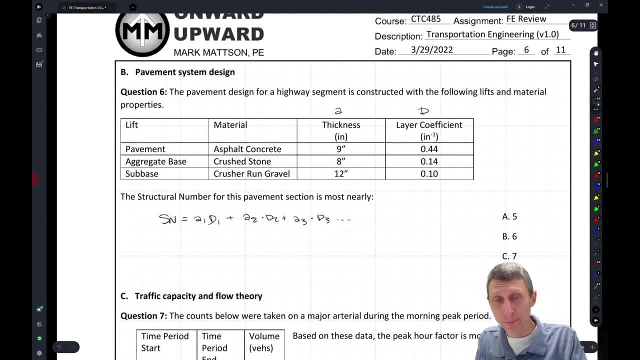 drainage coefficient. we're going to say this is d. we're going to say this is a. i'm just going to make another row over here. a times d, right, and if i, um, if i do those at nine times 0.44, that's about half a little bit less. i got 3.96. okay, um, eight times 0.14, that's pretty small. i can't. 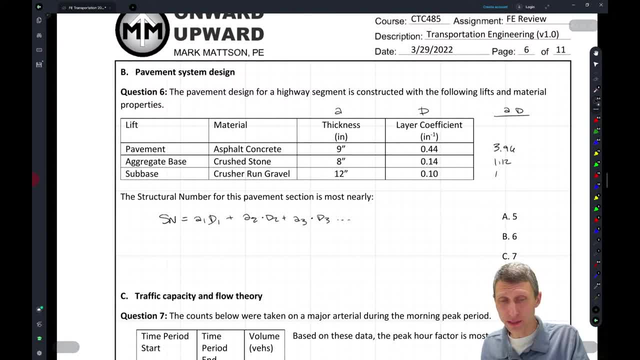 i got 1.12, um 12 times 0.1, that's just going to be 1.2. so really, where we end up is we get our structural numbers just the sum of this, you know if the sum of ad. sorry, i'll write my d? uh like the. 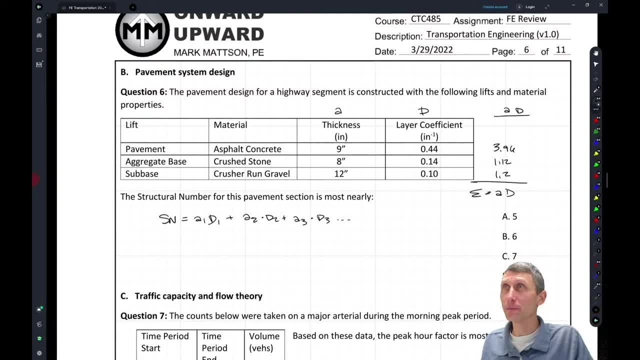 rest of them. but if we just sum that right, what we get here is the structural number equals. i think that works out to be about six. okay, so nothing too crazy. um, you, you know, i think it's like 6.28, right is the is the value that i ended up getting. um, and that's going to be most nearly, you know. 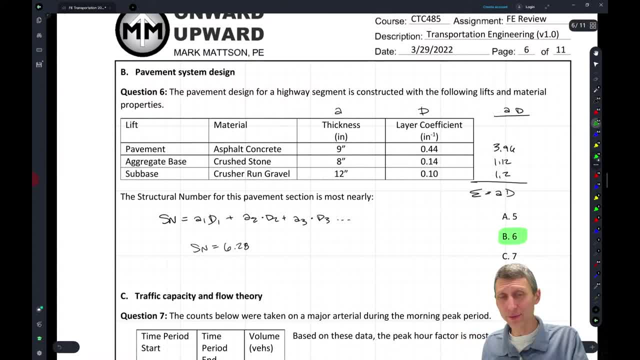 six, what? how else could you do this? um, you could be given, you know, if you're given, a structural number and you know you have to find, uh, you know, find the sub base depth or something like that. right, so they could switch this around on you, but nothing to i mean, i that equation is an equation. 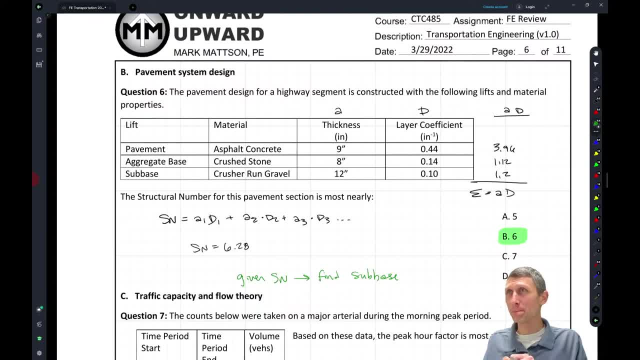 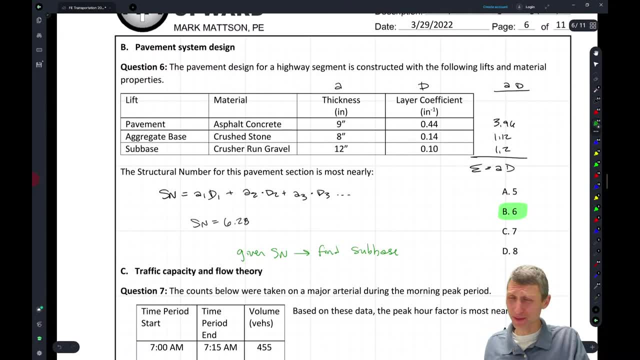 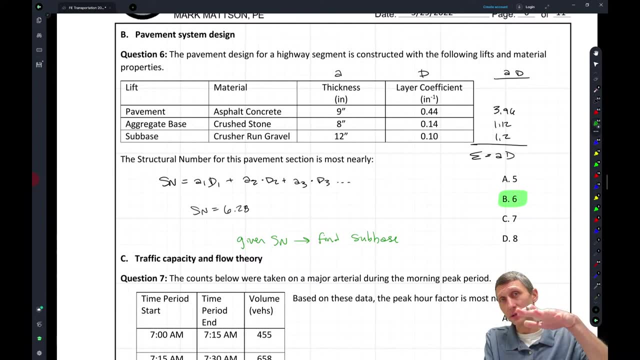 right, it's not. i don't think it's going to get super crazy in terms of what they're asking you for, okay, but i think this could lend itself more to possibly some concept questions like: what is the, the sub base versus subgrade? right, subgrade is all that material that's existing, it's all the soil and it's assumed to have a. 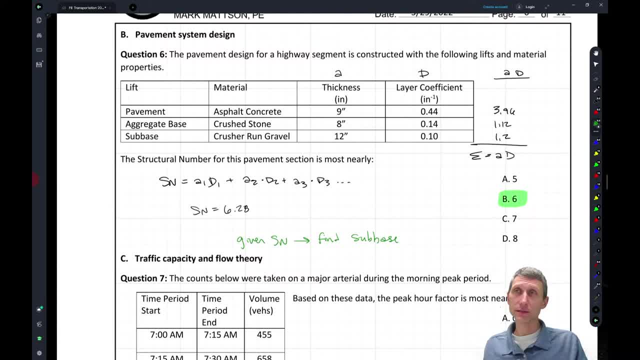 depth of infinity. so it's just, it's huge, right. it's just, it's earth, it's it's planet earth that you're on, um, obviously it affects the pavement to a certain degree, but here, um, we're looking at structural number just based on this asphalt. 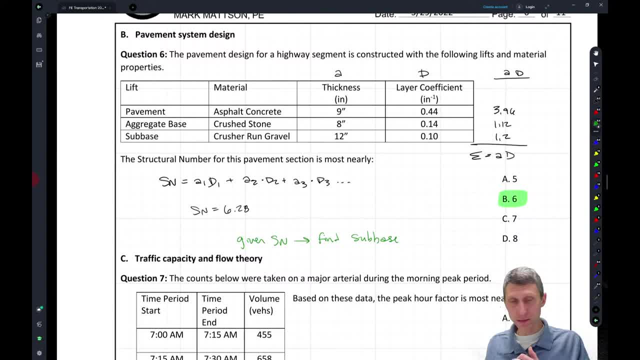 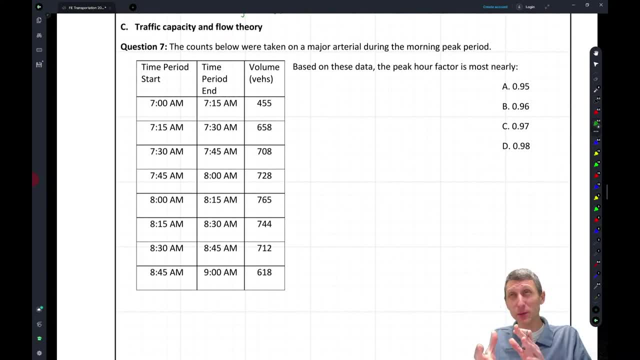 uh, the, the base, the sub base, um, those pieces, so, um. so let's keep going here, because i let's go to traffic capacity and flow theory, so so we kind of went through those curves kind of quickly. i wish i had more time to spend on just curves, uh, but there's a lot of, uh, there's a lot of, there's a. 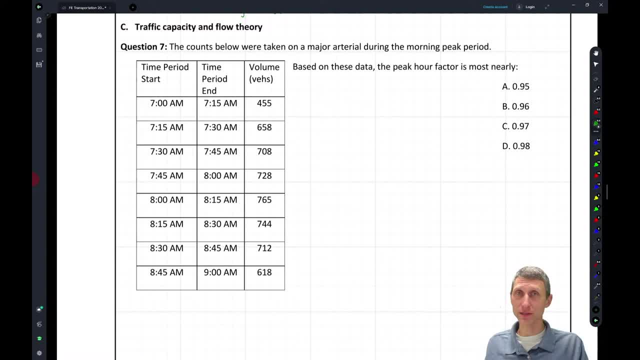 lot of questions. you can do with curves and it's just. you could rearrange those equations all sorts of different ways. but i think if you have some of those pieces down, like stopping site, so stopping site distance, you're good. i think the pavement if you kind of understand the basics of layers and drainage layers and 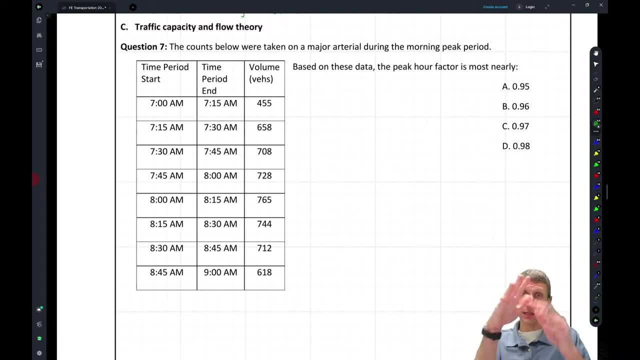 you know, getting things built up so you have some capacity to distribute the load down to the subgrade, that makes some sense too, and obviously if you have more, more load on it, you're going to want a bigger structural number as well, bigger, bigger capacity. and then we get into section c here. um, this is traffic capacity and flow theory. 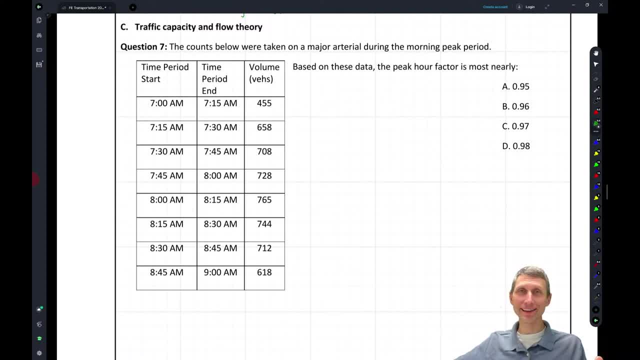 so i started out with just the first thing that you might be assigned to do is just the go count cars, right. so now maybe you're not manually sitting out there counting cars, maybe you're setting up counters, but sometimes i actually, early in my career, my boss told me: okay, go to this. 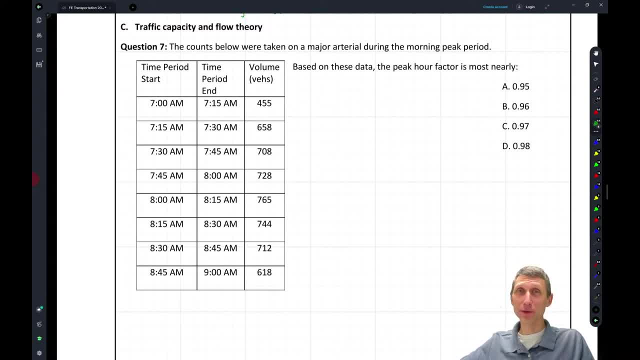 intersection count car through doing a traffic study. so i had to go out peak hour in the morning, peak hour in the afternoon. it wasn't like a super busy, it was just a- you know, a rural road, two lanes each way, nothing, nothing too crazy. but we were adding a big center on one side. we had to do a. 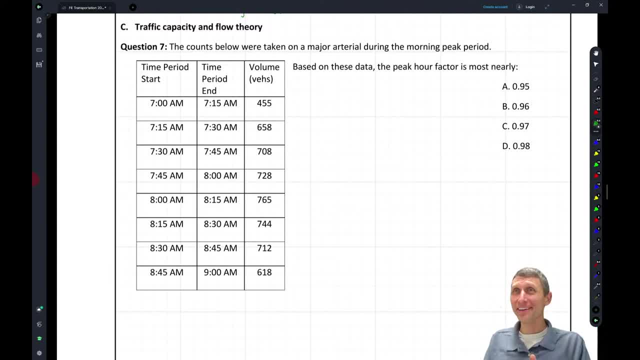 traffic study, my boss sent me out to go count cars, right. so you have a little tally sheets, you have counter that you're using to count and that's it right and granted, nowadays there's probably all digital ways to do everything but um, but still you end up with some data that that indicate the, the. 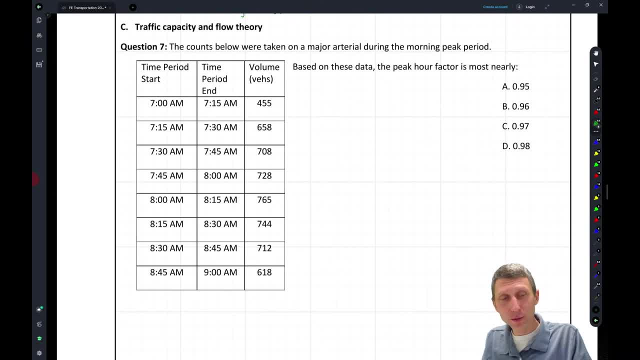 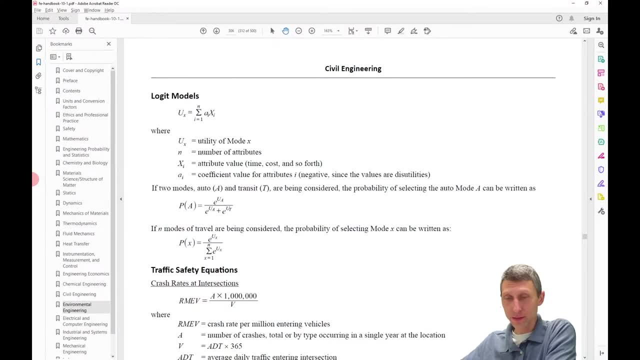 presence of certain number of vehicles. so when we're looking here, we're trying to find a peak hour factor and that's going to be something that's going to help us to design this, this, this facility, and if we come back here, uh, we can we see a phf there. that's peak hour factor, but i'm 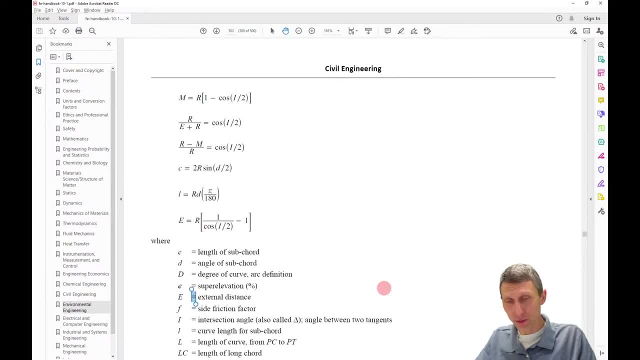 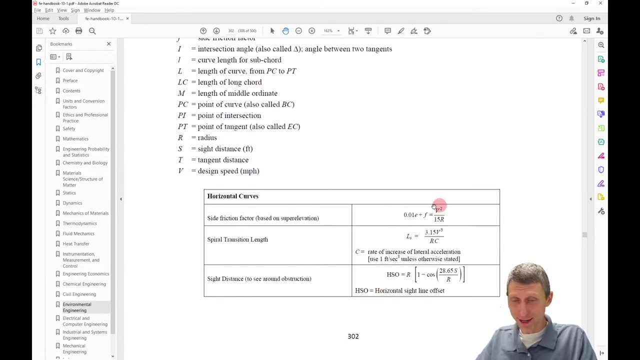 going to keep coming back a little bit further, i think, and actually now it's past horizontal curves. um, oh man, i didn't get into super elevation, but there's. there's not a lot going on here with spirals and super elevation, uh, but let's keep going here and let's look for that peak. 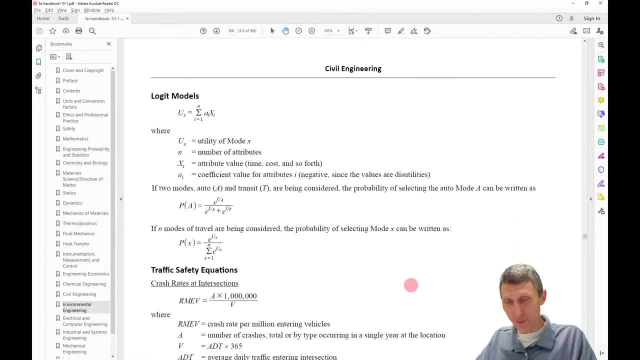 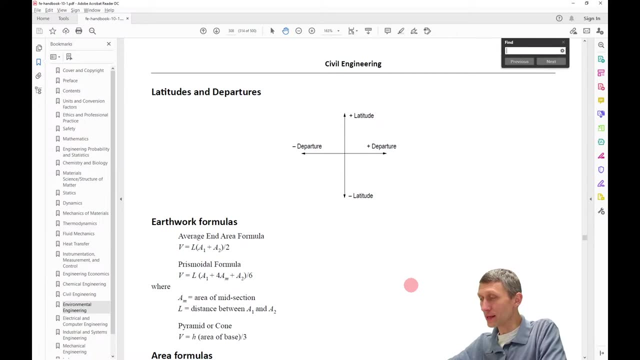 hour factor. where's our peak hour factor? there's. i know there's a formula in here somewhere and i'm probably missing it, and when you start missing things on the test, uh, that's where you're going to be able to do that. so i'm going to keep coming back a little bit further, i think. 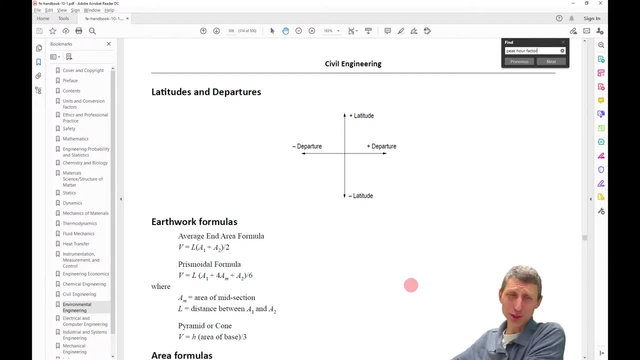 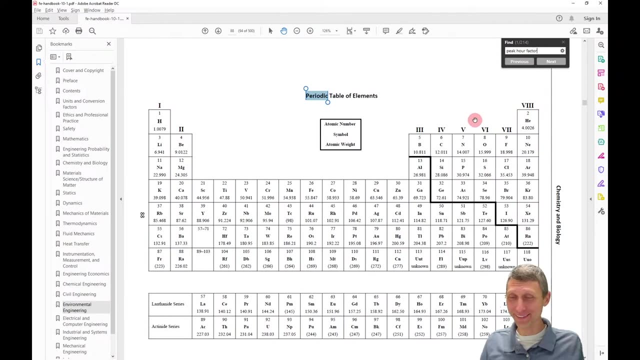 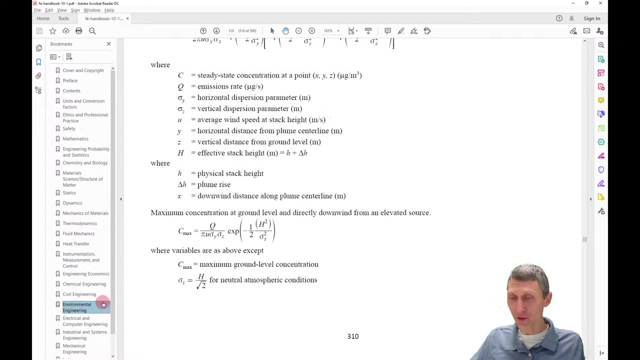 that's where, hopefully, the search comes in and you're able to find it right away or not. um, and sometimes adobe does this to me where it just kills me. it goes to periodic when i search peak hour factor. so i'm going to come back here, i'm going to zoom out. um, that's another. 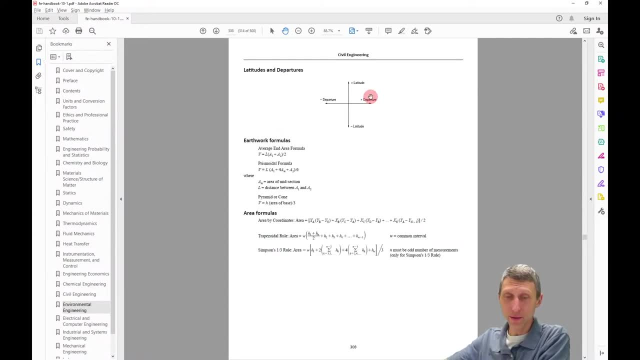 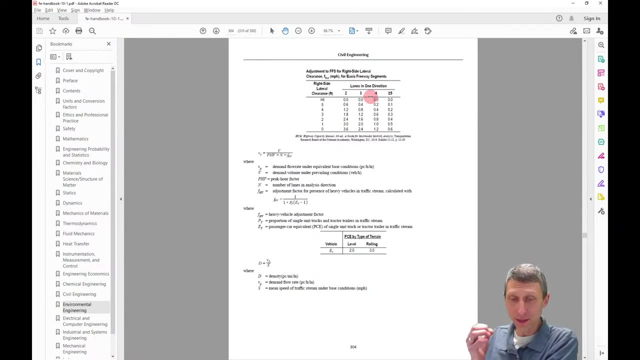 suggestion as you, as you're finding things. sometimes zooming out helps, because sometimes you miss what you're looking for on the page, um, when you're looking for this, right. so what is the peak hour factor? oh, it's right there and you might think like, but it doesn't tell it. but it does. we got to keep coming back. 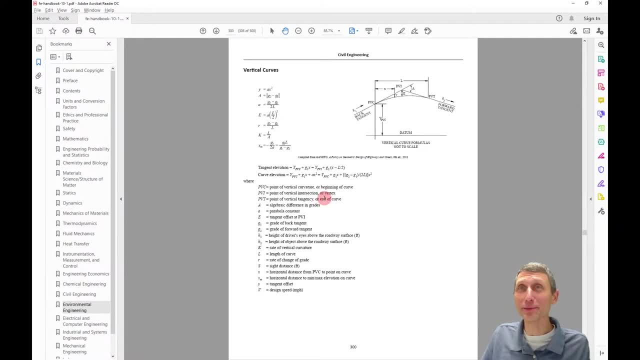 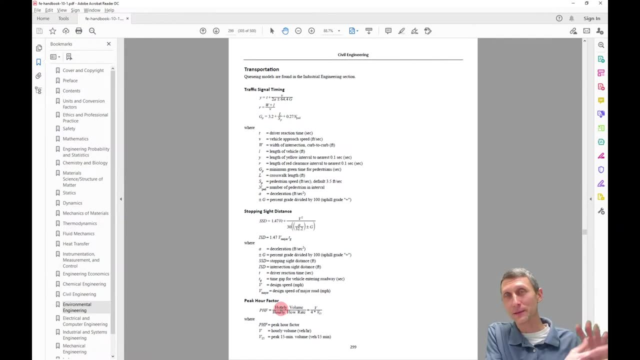 and it does show up here and maybe somebody could put it in the chat. it's it's in here, i think. oh, there it is, it's it's up here. so, even though we're in flow theory later on, we get this peak hour factor up here. so that's okay with the hourly volume divided by the hourly flow rate, okay, so. 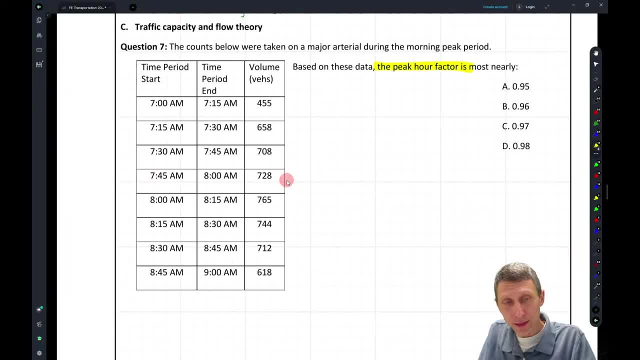 let's come back in and look at that. so we're going to say the peak hour factor. i'm just going to write it down here. the peak hour factor equals essentially v over 4 times v, 15.. so that's great and we got this thing going. 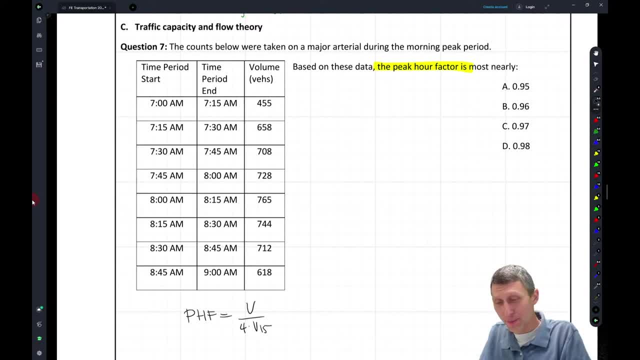 but it's. it's like: wait, wait, um, we have thanks, page 229. don't forget that. okay, um, sometimes actually it does help to remember relative pages, but but another good thing with the test is they don't jump you all over their place. normally you're in one section, you work through the page and you're. 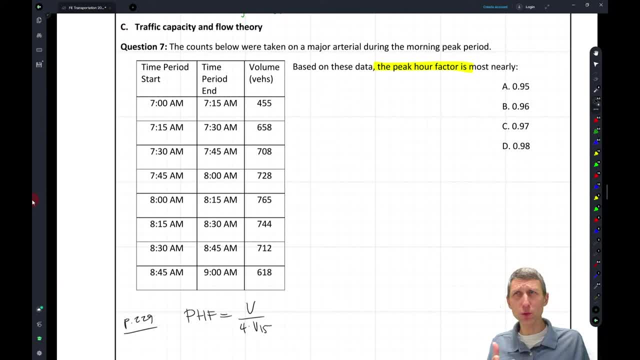 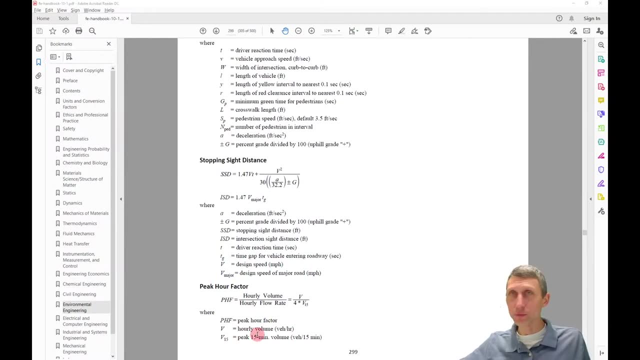 that section until you're done, until you're done. so we we have a bunch of 15 minute time intervals here, but what's our v? right? what v are we using? and that's where we can come back to the manual, the handbook, and think like, okay, we got this. we're looking at an hourly volume, so okay, okay, we got. 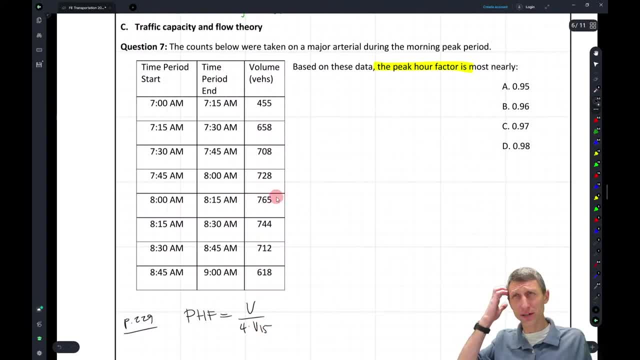 an hourly volume. we come back here. you scratch your head a little bit and maybe think like, well, what's the hourly volume? well, in this case there's actually a lot of hourly volumes, right? so in this case there's the first hour. okay, what's the hourly volume for that? so we can add up this, these, these four numbers, and 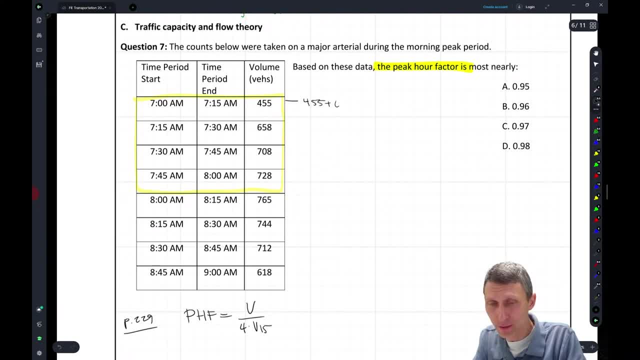 if we add up those four numbers- 455 plus 658 plus 708, you know, plus 728- what do we get? um, i got 2549. so that's the first hour. what do we do next? well, we come up here. i'm just going to get a different. 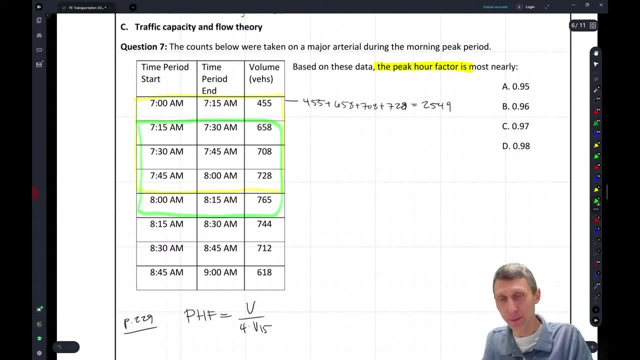 color here and i'm going to come here and i'm going to say, okay, that's the next hour. so, essentially, what i'm going to do is i'm going to subtract minus 455, but i'm going to add back in. what am i going to add in? i'm going to add in the 765.. so in when? 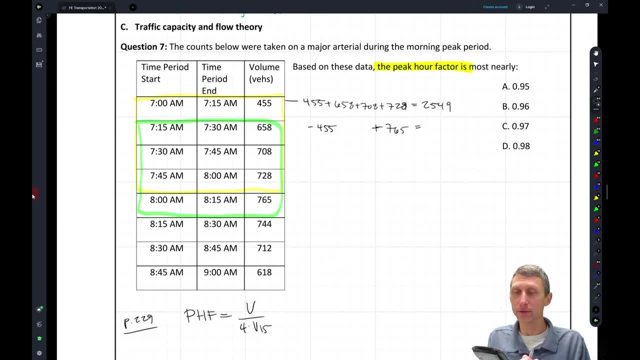 you're using your calculator sometimes, that's that's a more efficient way of doing it, right? you have a 25, 25 um 49 if i subtract off 455- because we're losing the 455 here- and then we're adding this 765, uh, we're gonna get like 28.59. okay, 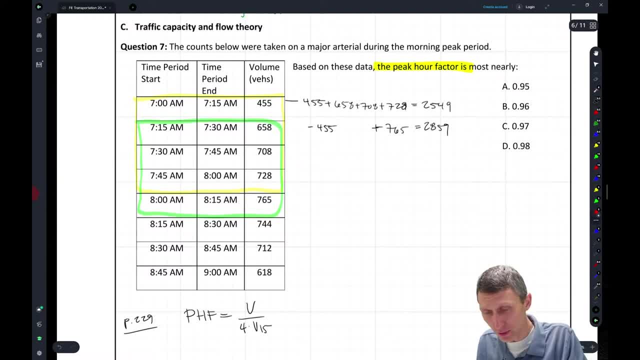 and basically we have to do that, we have to just keep going down. so we're going to keep coming down to this one. um, we're going to go down to, you know, this one, and then i ran out of colors here, so i'm just going to come back and use the same color here for the last hour. 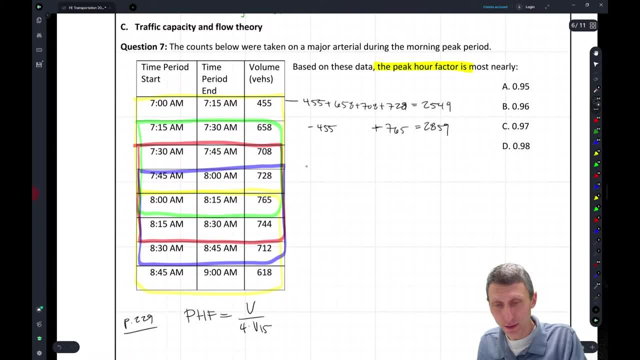 as well. but basically i'm just going to say, you know the if this is the green one, the red one's going to be, uh, what's the red one? i think, 29.45, the blue one's going to be um 29.49 and this last hour here is going to be uh, 28.39. so these are, these are a bunch of. 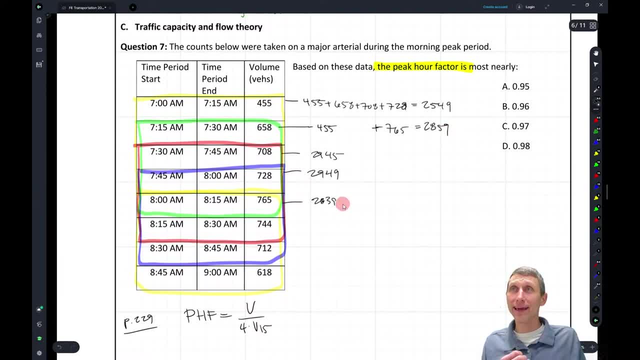 hourly volumes. now, right, so we have a bunch of hourly volumes and what we want to do is just take the biggest hourly volume. so the biggest hourly volume is going to be this 29.49. that's our largest hourly volume and what we want to do with that is we want to divide it by the peak 15 minute volume within. 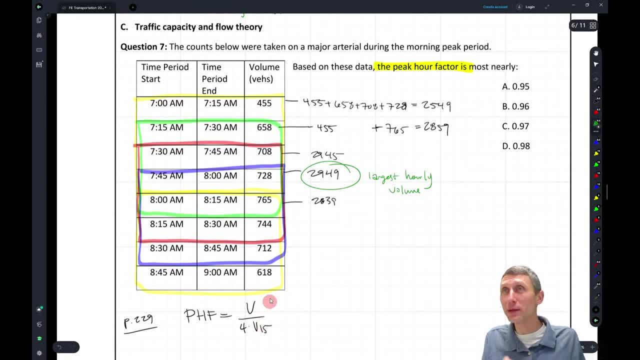 that volume right. so we've got this 29.49, that's this blue one and we're going to take the peak one inside of there and this is going to be our v15 and it's our peak 15 minute volume. and once we know that, the cool thing is we can just solve this equation. the equation isn't super. 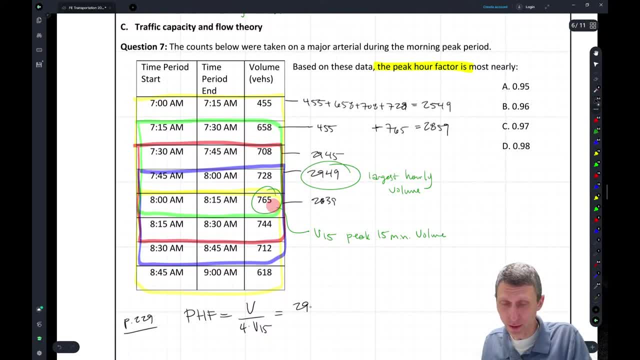 hard math, it's just 29.49. and then we just divide that by the peak 15 minute volume, 9 divided by 4 times 765. right, and what's this? this is the, basically, this is vehicles, right, per vehicles. so our units are gonna go, our units are gonna. 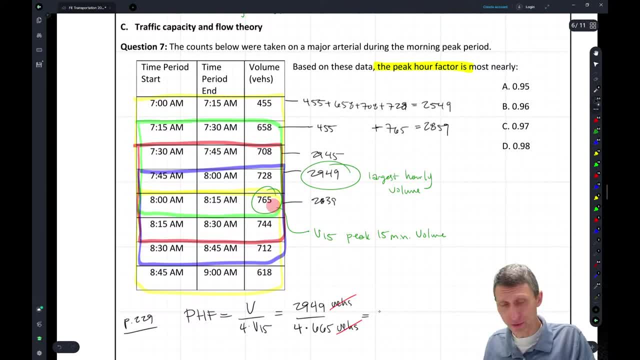 cancel out and we're gonna end up with about 0.96. okay, so that's gonna be. that's gonna be our answer, if I did the math right, I think. I think I I managed to get the math right on that one, okay, so I so let me just I'll check that so. 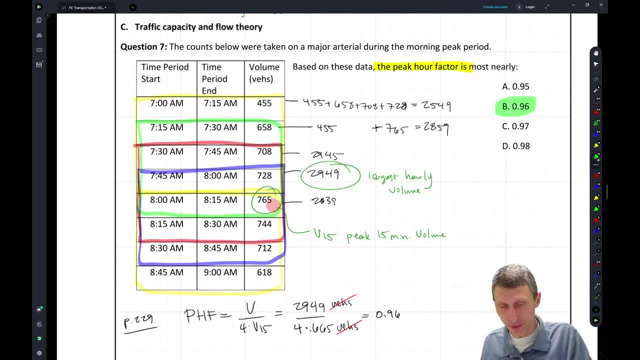 29, 49 divided by 4, divided by- I wrote it wrong. it helps to write things right as well. times 765, right, somebody's gonna put that in 765 up here- divided by 765, and I got the point. nine six three. okay, so I'm happy with. I'm happy with that. 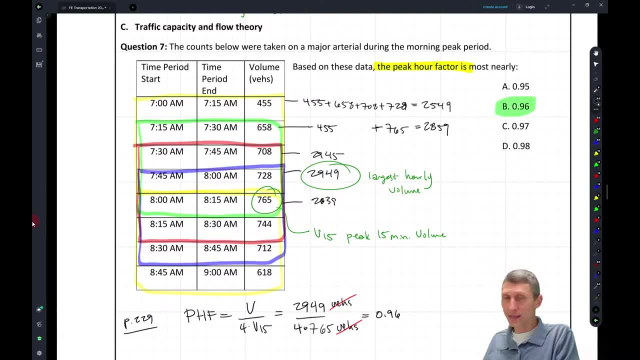 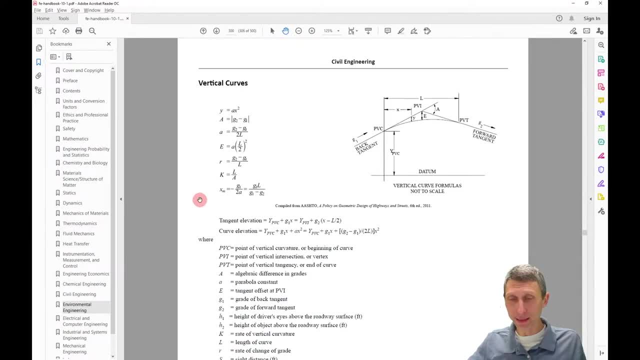 there's. so that's a peak hour factor. how do we use that? we use that in different ways. you'll see that show up. we'll get that actually a little bit later, but you do see that show up. once we get back into here. it's past curves again. we get past. 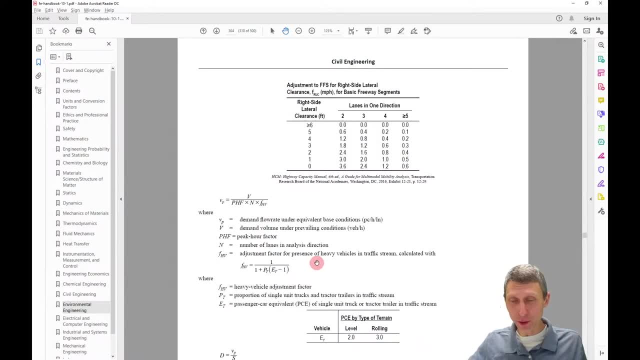 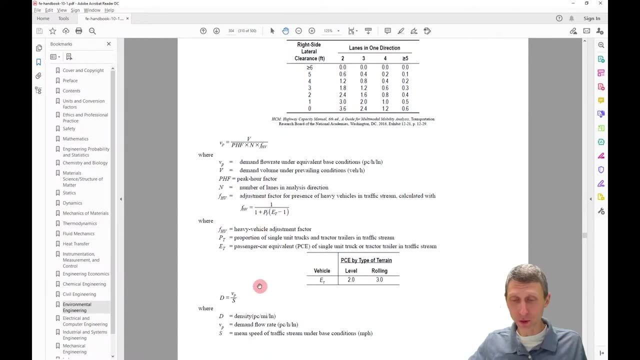 these curves. we get into some of our flows down here. but you know some of this demand flow rates. you're gonna use the peak hour factor, so we'll get into a question over that. we're gonna look at now. we're gonna look at some of this. 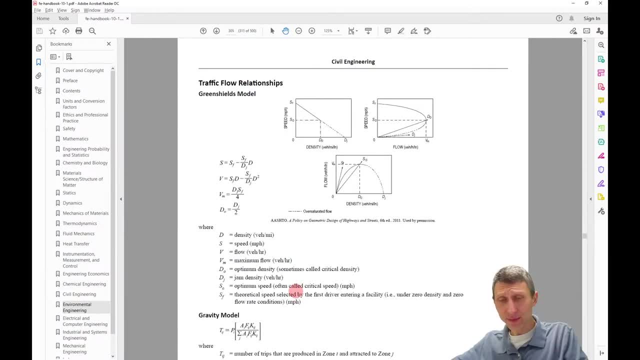 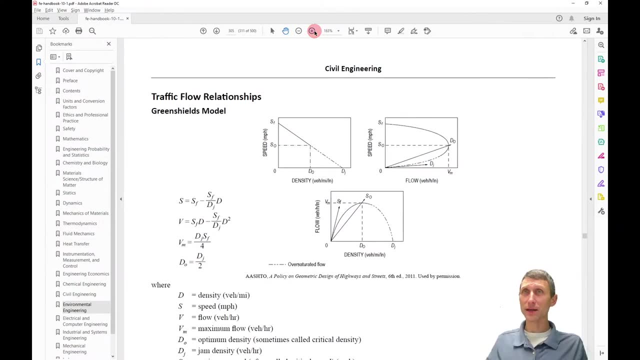 traffic capacity and flow theory, and this is a- uh, a green shields model. it's one of those models that gets taught, I think, in every traffic capacity analysis type of class, but the idea here is: you have some, you have some, um, some, some free flow speed, so if nobody else is on the road, 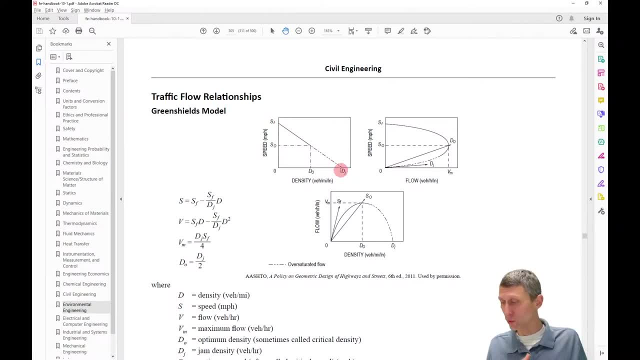 how fast are people gonna go? um, you have some jam density, so when is this? when are you going to just jam up the road? and then, somewhere in the middle, you have this optimum density. the idea here is like when you have, you know, when you have nobody else on the road, you have a low. 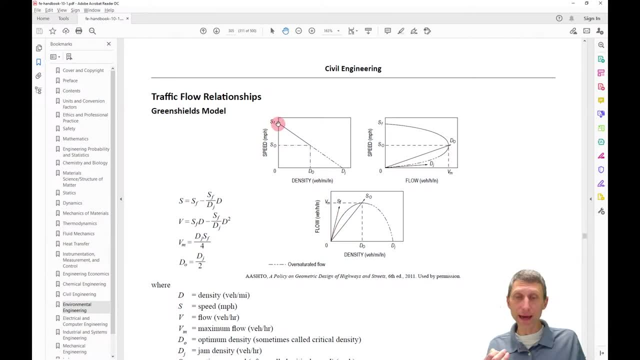 but it's not optimum. you know, you can get, you can fly, you can go fast- not that you guys would speed, but you can go fast. and then you have the point where everybody's there's such a traffic jam nobody can go anywhere. so that's not a good low right, but but somewhere there's that sweet spot. 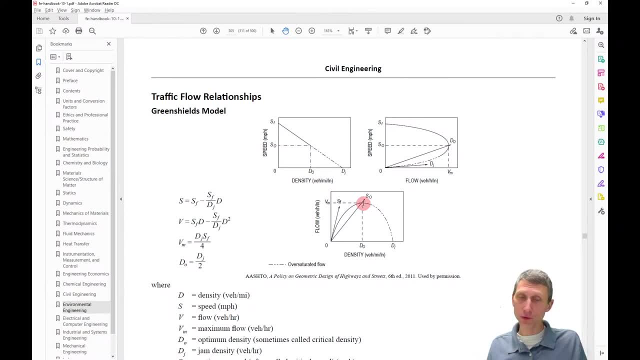 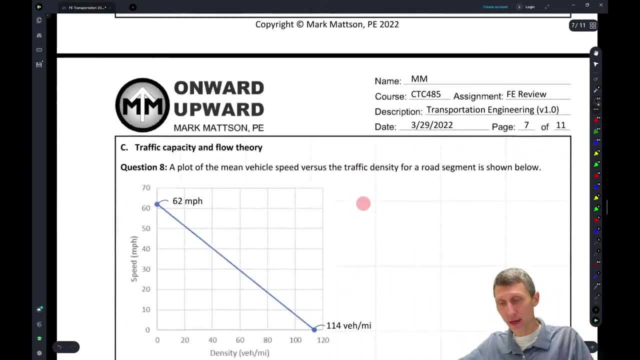 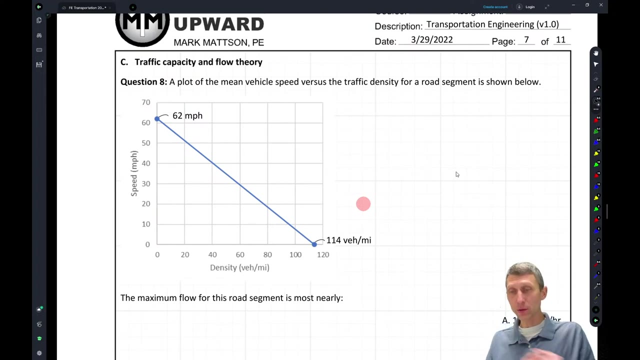 where you get the most vehicles possible through this, through this, this, uh, you know, through this, this roadway. so the idea here is we're given a relationship, um, in this next problem of the vehicle speed versus the traffic density for a road segment. right, so a vehicle speed. 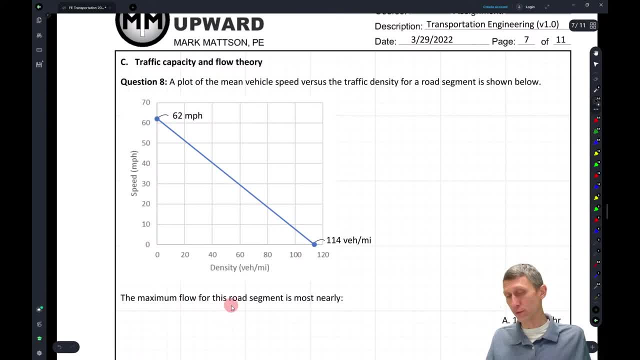 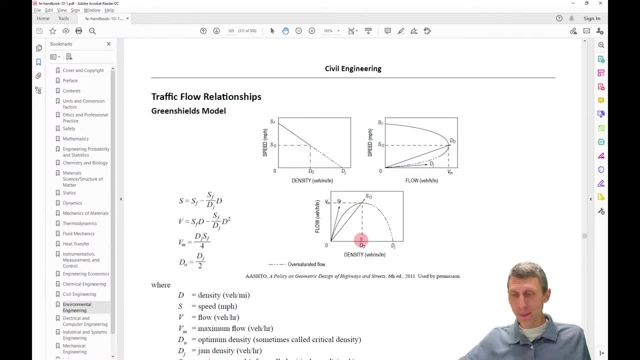 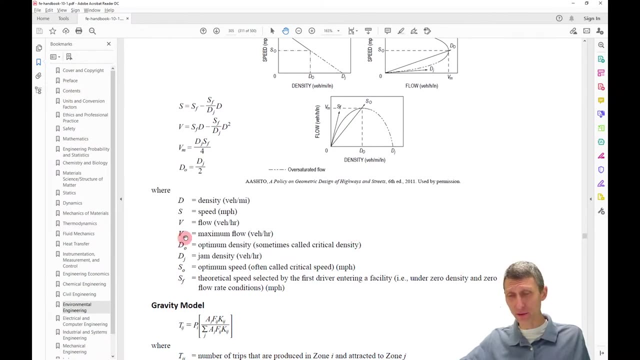 versus density and we want the maximum flow for this road segment. so what we know is we're going to go somewhere kind of between this model to this model. but the the cool thing is, here we're. we're also given an equation that that really calculates that for us. so either our maximum flow, 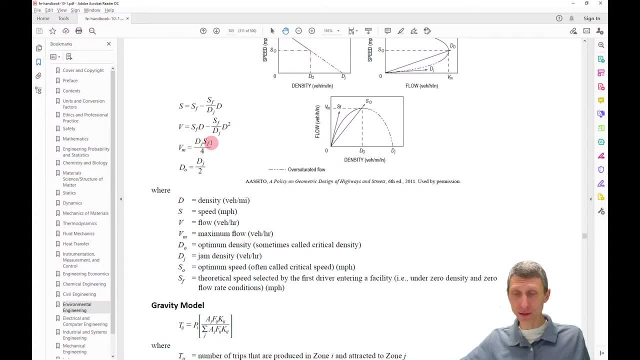 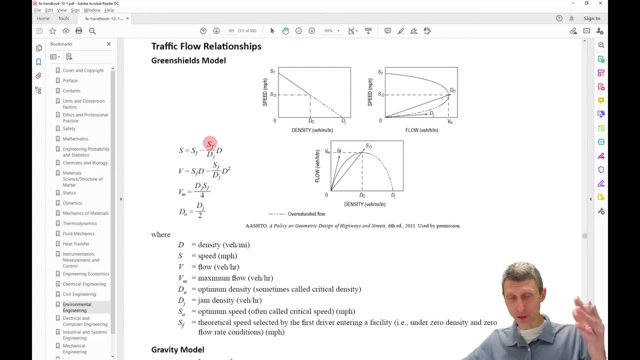 is going to be our jam density times, our, our free flow speed, or optimum speed. i should say um, or theoretical speed selected by the driver if nobody else is on the road. okay, um divided by four. so that's kind of like this, this optimum and optimum we can. 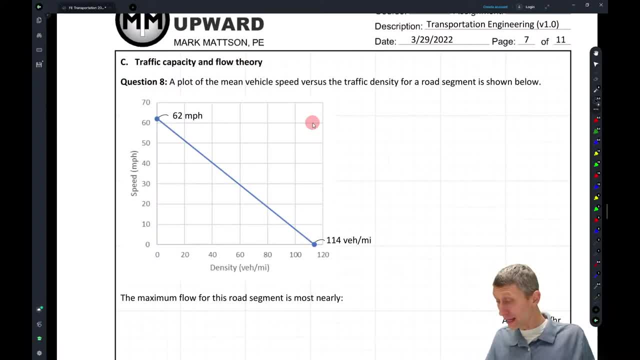 multiply those two together to get the same thing. so, um, that's just going to be right, that's just the formula here. but vm equals- uh, we have dj times sf over four. so what's this equal to? it's equal to 114 vehicles per mile times 62 miles per hour over four, and that's going to be 1767. 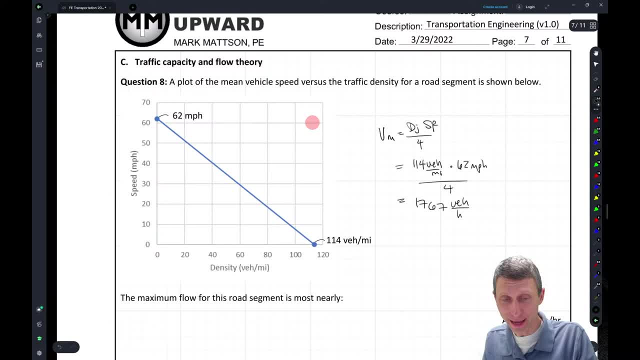 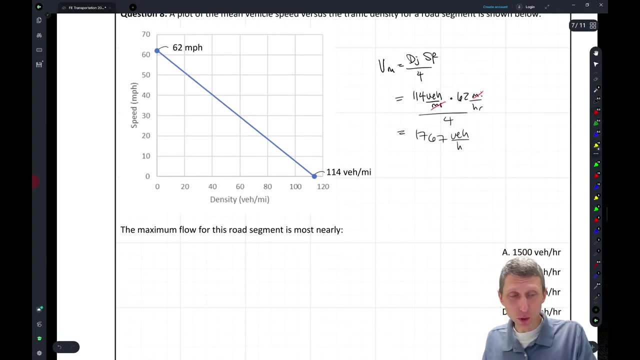 vehicles per hour and actually let me write these units out for a second: miles per hour. right, the units actually work out to the miles we get. we get rid of miles and we get to down to miles per hour. okay, and i don't know, i don't think that's going to work out for us, so we're going to have to. 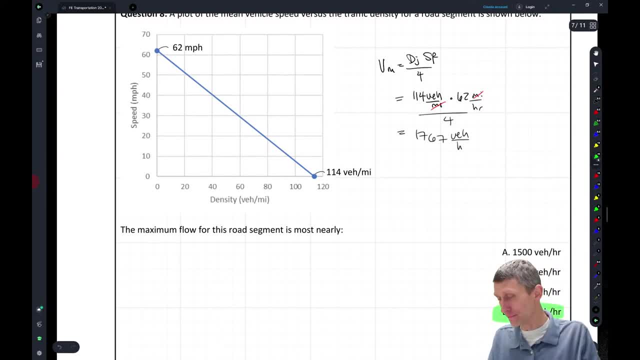 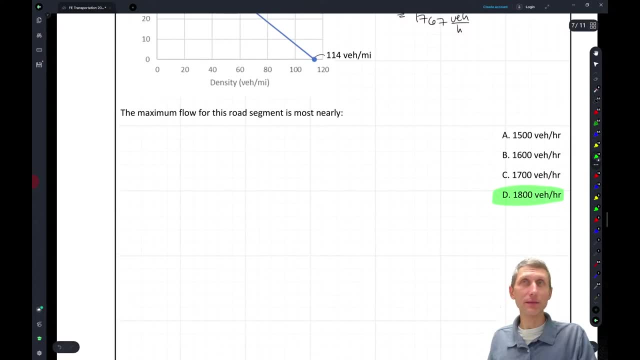 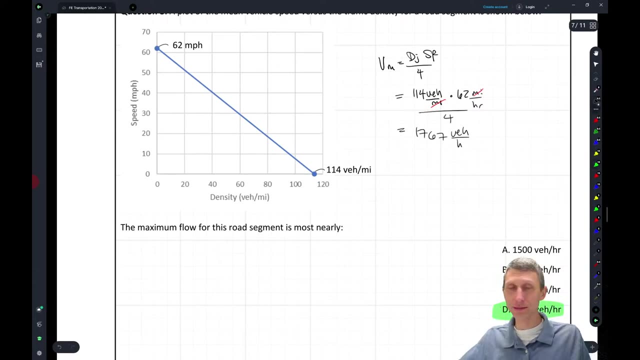 think about that, whether or not that's going to work out for this meinado tr a few days ago. we will respect on truth. that's probably going to help us a little bit further from what we were talking about, but so it's. an interesting thing is that this imagine, this idea here is these: 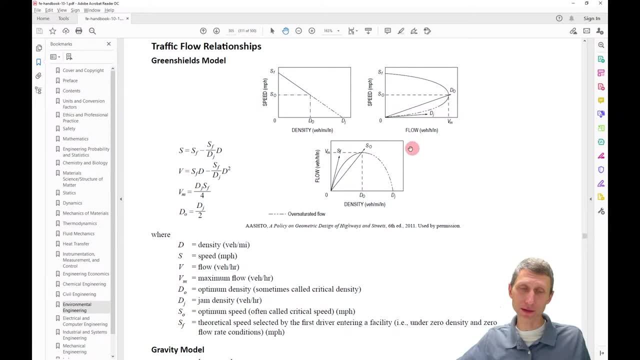 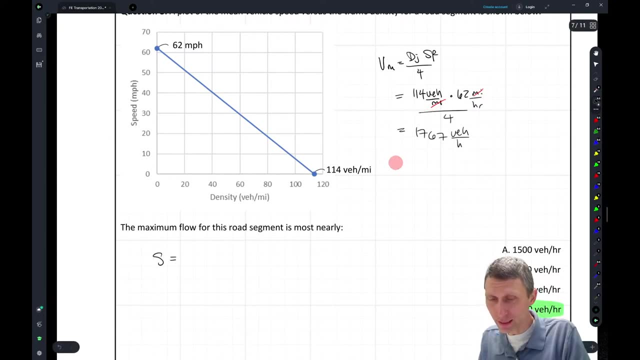 equations here are all interrelated okay these equations here interrelated and if i were to think about this i i know that the speed at any point this the speed this is how many miles per hour is an u plot then we put in the mountains. m � crafting requires several thousand kilometers 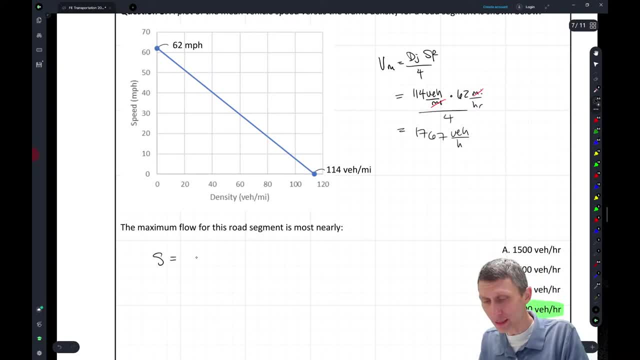 high p-of grade. you can't have homes yards between each other and y the whole Viher Development would judge the rangeuse by an u- infected that, in contrast to all the others, this is pretty complicated right line. i could find an equation for that. i could say: that's minus 62 over 114. that's the slope of. 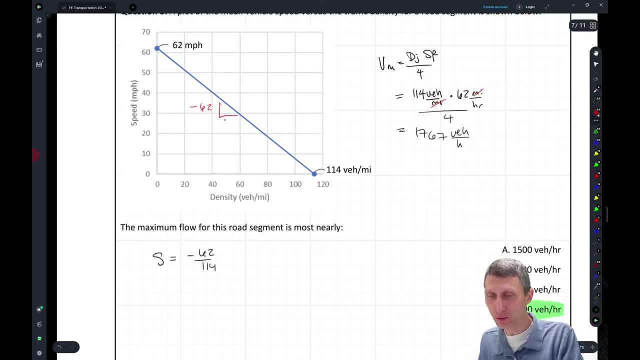 this line. right, that's the slope of this line as i come down: 62 and over 114, um times what, uh times my, my, my density, and then my, my y intercept is going to be 62. so that's my speed equation. okay, and what? what else do i know? i know my flow equation and this is where, like sometimes, it's. 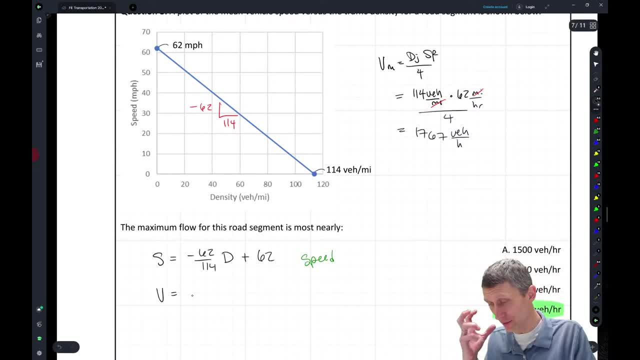 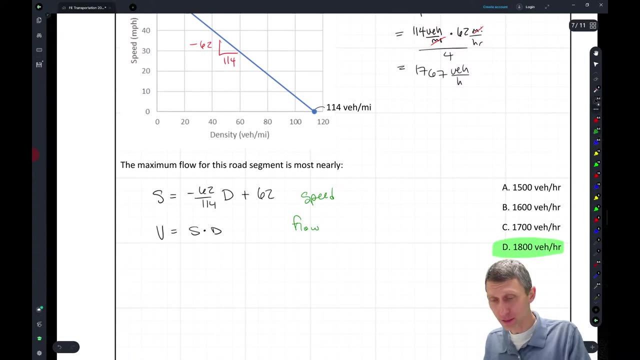 good to have this idea where these things are interrelated. um, you know how they're interrelated. flow equals speed, times, density. so if we know that we now have kind of we, we can, we can solve this as well. we can say: this is flow right. and again, if you want to punish yourself, go for it. 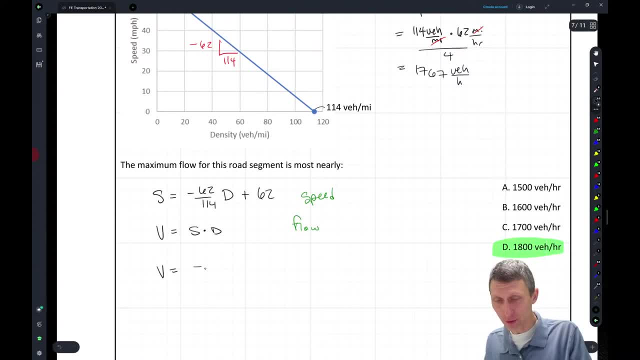 but here's b equals. what if we substitute s in here we have what? minus minus, minus 62 over 114, um d plus 62, you know um and then and then plus 62. did i get that right, or i think i'm? or no. times d, i'm sorry, i'm times z, so i'm just substituting in uh for s, so you could do this. 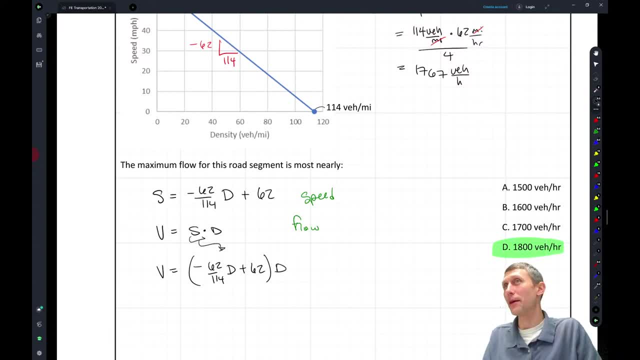 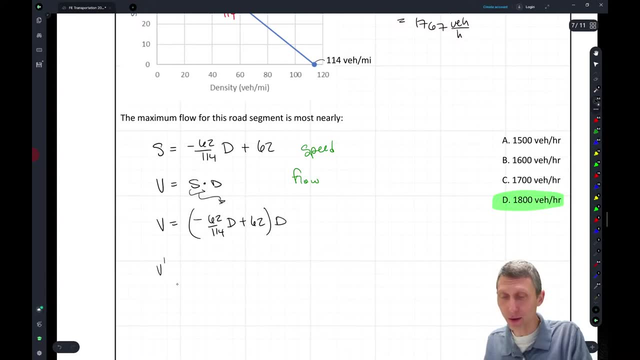 and you probably learned it this way in a transportation capacity analysis class, because this is one of those things that you should probably know, because then, what can you do? you can well. you can take b prime, you can take the derivative and you can solve. and when you solve, you get, like you know, minus 2 times 62. 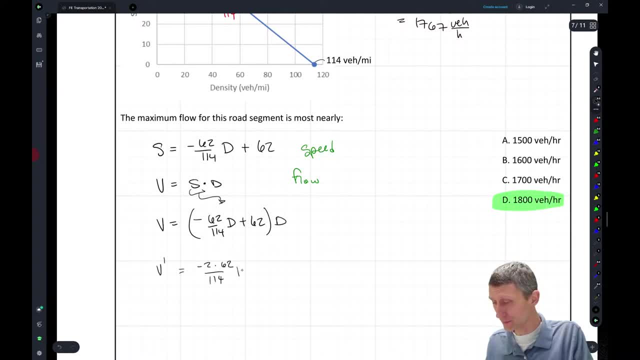 over 14, or 114 um d plus 62. so so we get this derivative. i skipped this step where i distributed the dn. okay, but basically, if we set this equal to zero, if we set this equal to zero, set, you know, equal to zero, we can also solve for. 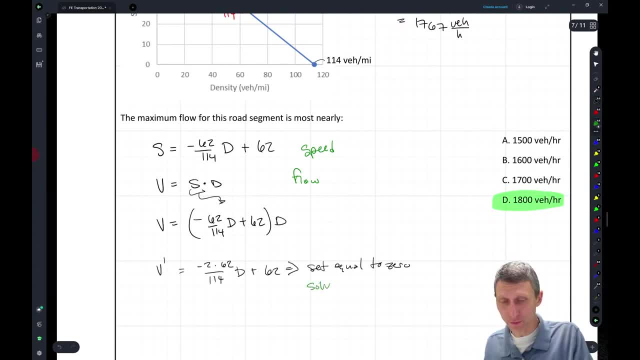 um, we can solve. we can solve for what are we solving for? well, this is a parabola right, so essentially we'd solve for that um, the location, the, the maximum density, or, i'm sorry, the optimum density i should call it. do like everybody else does in the handbook. 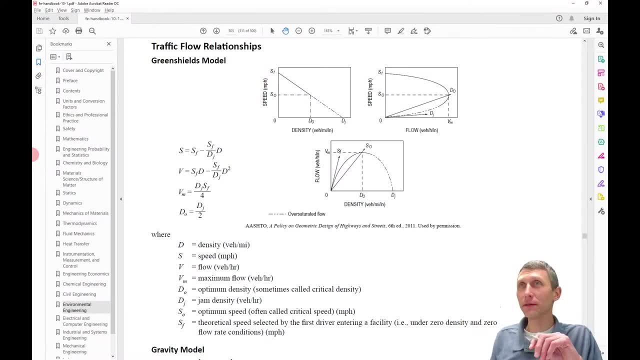 so i probably- i don't know the reason i'm going there- is just because, like, sometimes it's, it's it's worth understanding a little bit of the concepts, but that, like you know, this equation here is related to this equation here, right? so in understanding that idea that, um, just the basic, i 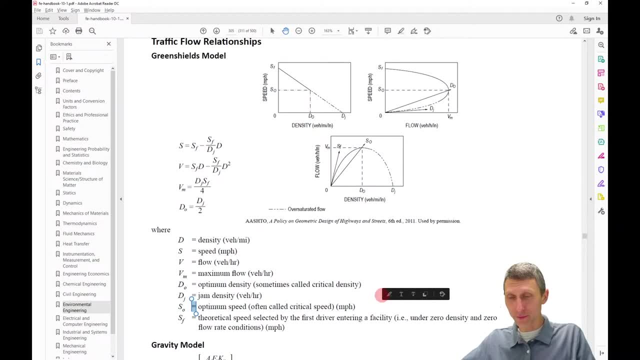 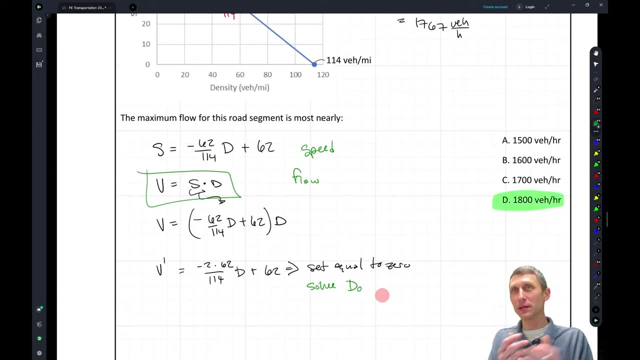 don't see this formula of of right of v equals um s times d. i don't see this basic formula in there. but this, this relationship, is one of those relationships i wanted to take just a couple minutes to like hit on and i i don't know if this calculus is just. 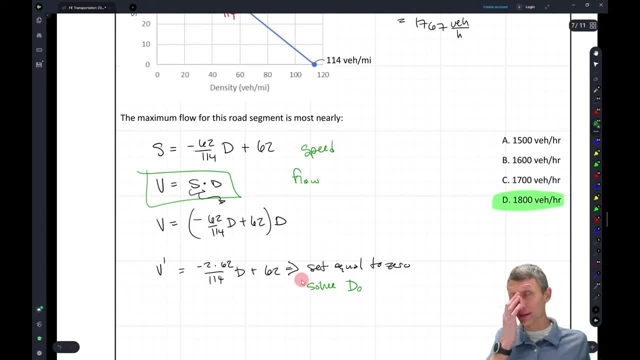 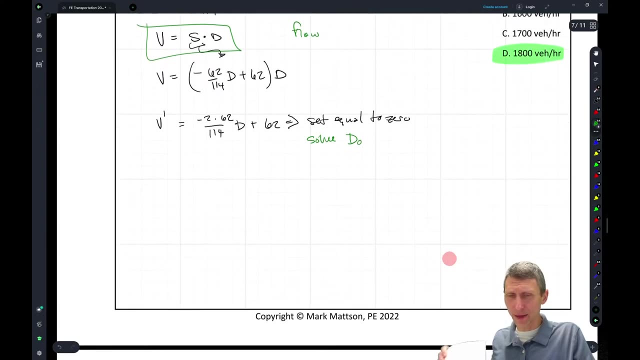 too annoying for you, just leave it and leave that to the math section and um and go. but you can do this the same way. you can solve for do you can substitute back in and solve for your flow rate. you'll get the same. you'll get the same thing, okay. so just another thing to kind of think about out. 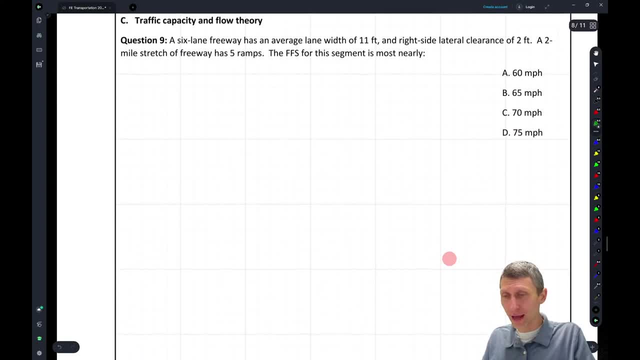 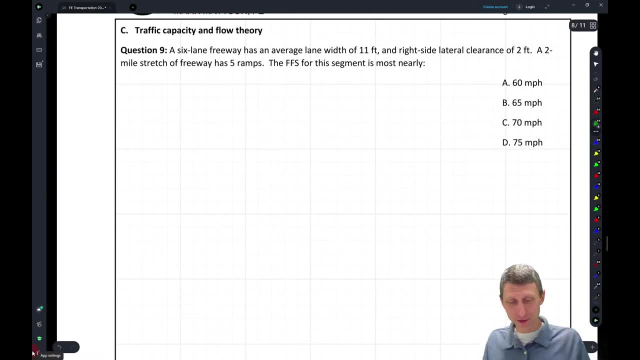 there, but let's keep going here and now we get into traffic capacity and this is where we get all those those multitude of of uh factors and empirical, you know, formulas and tables that we have to go look up, and the highway capacity manual manual is full of them. but here we have a six lane freeway, an average. 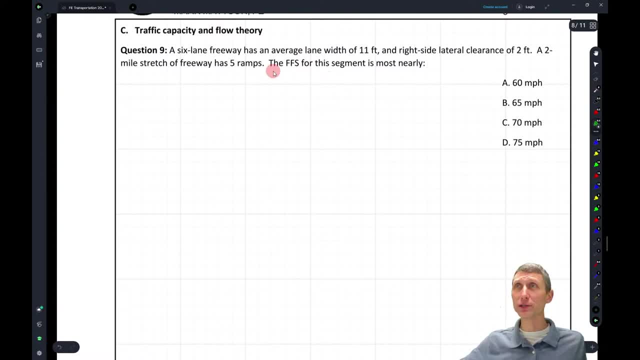 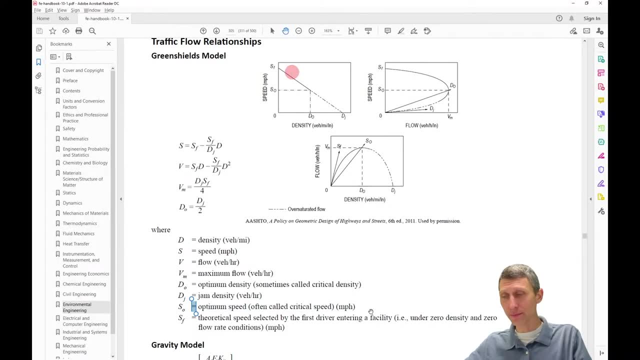 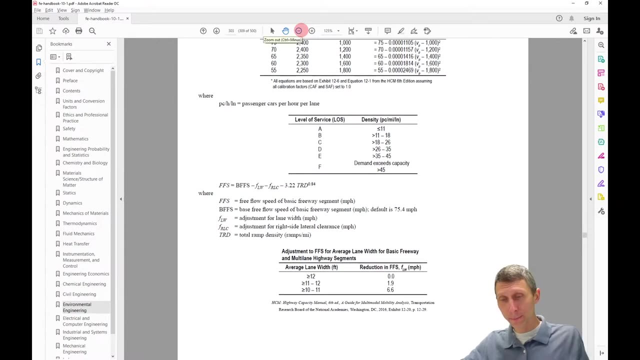 lane width, right side lateral clearance, a two mile stretch with five ramps. the free flow speed, the ffs free flow speed, is most nearly so. let's come back and come to the free flow speed here and let's find where that is. we have a free flow speed which is going to give us our base free flow. 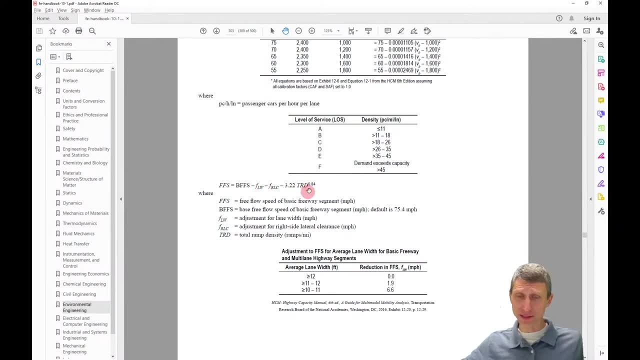 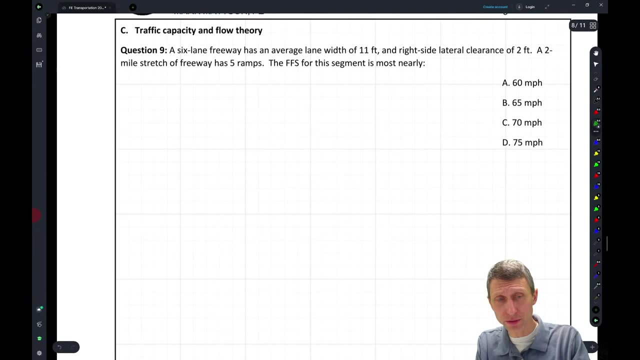 speed, um, the, the lane width, the right side, lateral clearance, all these things that we need, and let's use that to solve. so i'm going to come back and i'll write that in and we'll just keep going. so, uh, what do i have here? i have the free flow speed equals the base free flow speed minus the the lane. 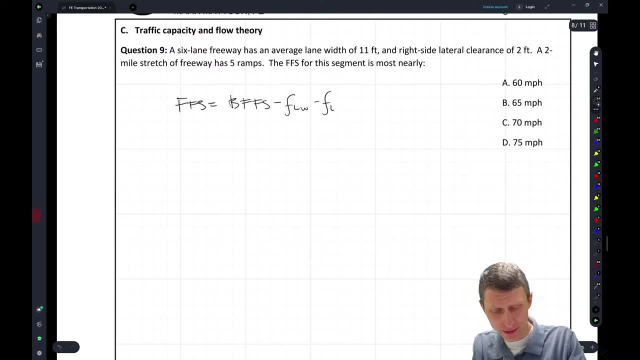 width adjustment minus the um. actually it's the right side lateral clearance. i want to always say the that doesn't matter the right side lateral clearance minus 3.22 times the total ramp density to the 0.84. and somebody spent a phd to just get that 0.84 um. you know number, but but this is where, okay, we have some of these. 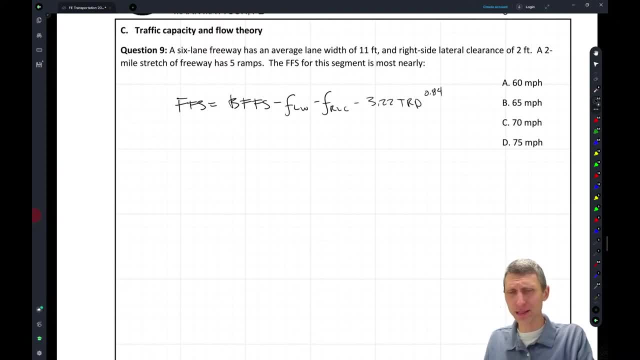 pieces we have. well, do we have some of these pieces? and you might think like, wait, we don't have some of these pieces. we don't have the base free flow speed. what is that, the base free flow speed? well, let's come back here. um, if a base free flow speed isn't given, 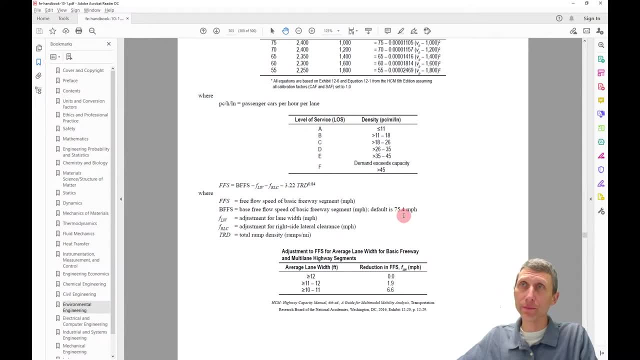 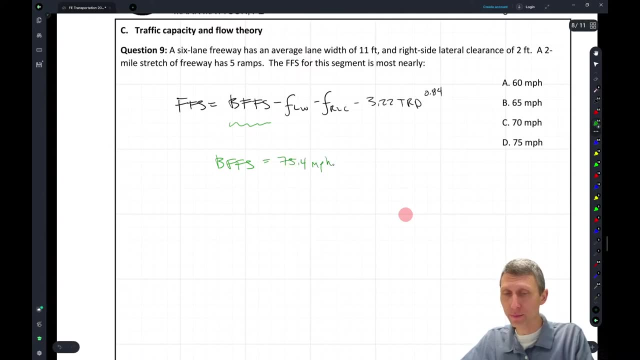 the default is 75.4 miles per hour, so we're going to use up 75.4, so we're going to say this equals 75.4 miles per hour. okay, that's where we start. let's look at this. flw- what's flw? 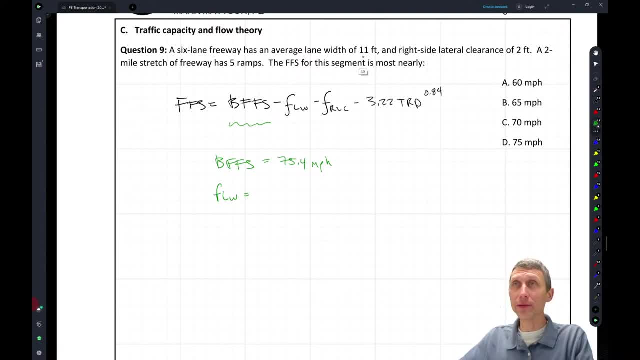 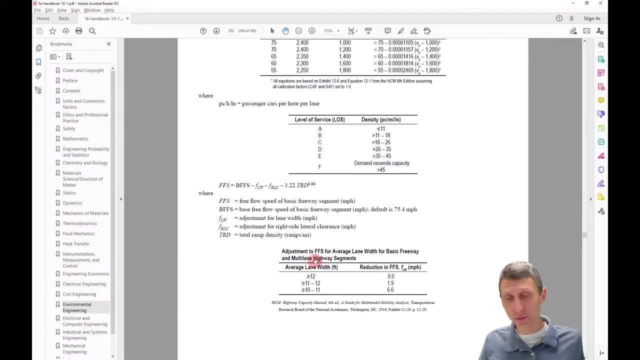 the lane width. our lane width is 11 feet up here. so let's come back and say: what do we have? we have an average lane width of 11 feet. so that's going to say we have a lane width 11 feet. that's greater than or equal to this. that's included in this lane width. so we're going to say that's going to say: 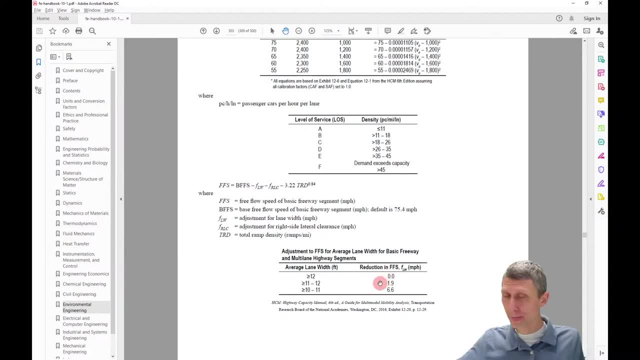 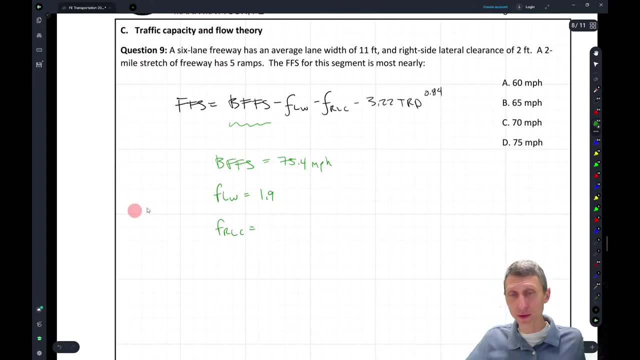 not in the bottom one, and we're going to come up with 1.9. so that's going to be 1.9. our right lateral clearance is going to be: what do we have? we have two feet, so let's look at our two feet. we 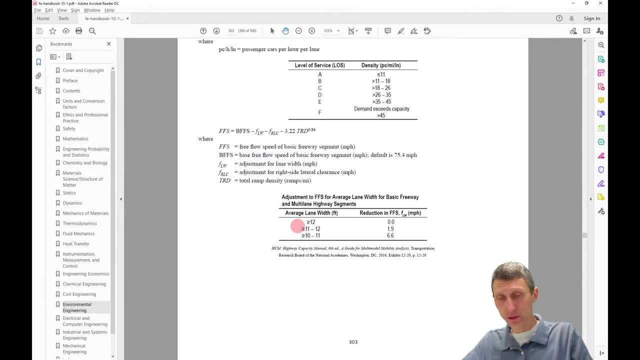 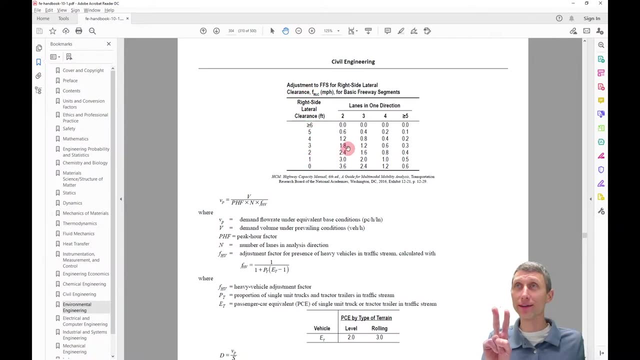 got to go to a new table here. so what's our new table? well, we have a right side lateral clearance of two feet. there's six lane highway. so do we go to three or greater than five? what do you think so? so this is where six lane highway- yeah man, i wish this actually does tell us that lanes in one direction. 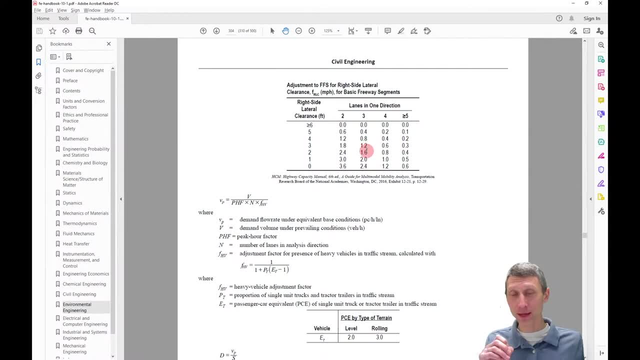 is three, so six lane highway is going to have three lanes in in one direction. uh yeah, basically it's it's the, the shoulder, so so we've got two side lateral clearance. um, we got 1.6 here for our fl or frlc, so i got that right: 1.6. okay, this is 1.6, and 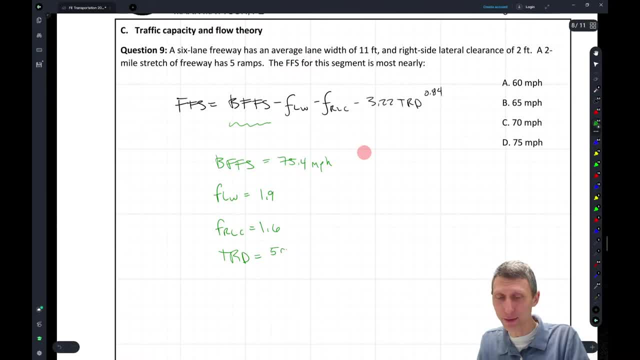 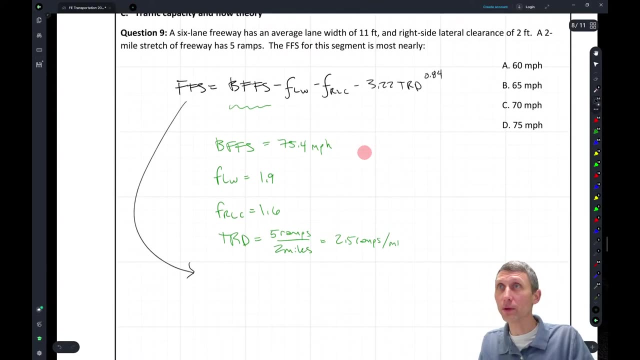 and now one area that has a lot of do some Dianegt total ramp density. what do we have? we're told that we have five ramps per two miles. so what's that? that's gonna be 2.5 ramps per mile, and the cool thing is now we 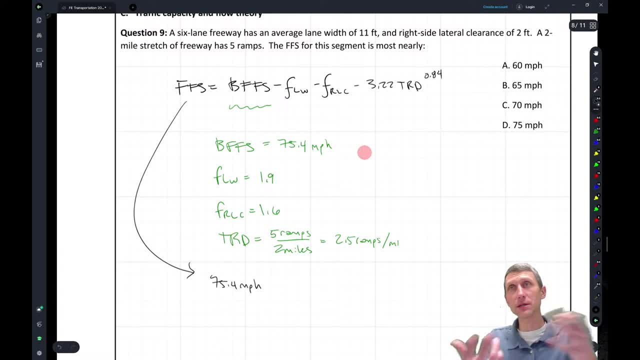 just plug and chug down here. um, what are we gonna get? we're gonna get the base free flow speed, which was 75.4 miles per hour, and then we're just gonna start subtracting off of that. so, And, Matt, I don't know if your question's to me or just other people, but in terms of delayed, I'm not sure. 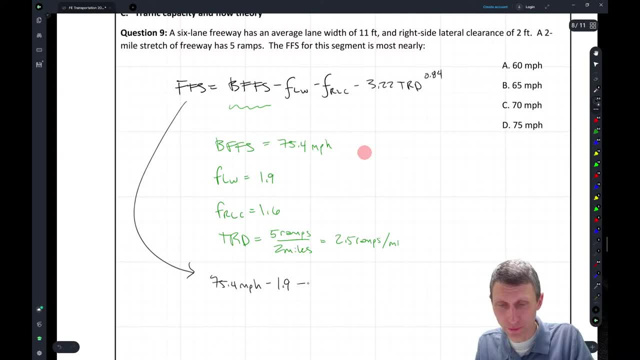 So what do we have? We have 1.9 minus the 1.6 minus. what do we have? We have 3.22 times our 2.5 to the 0.84.. And so I'm going to get a free flow speed down here. 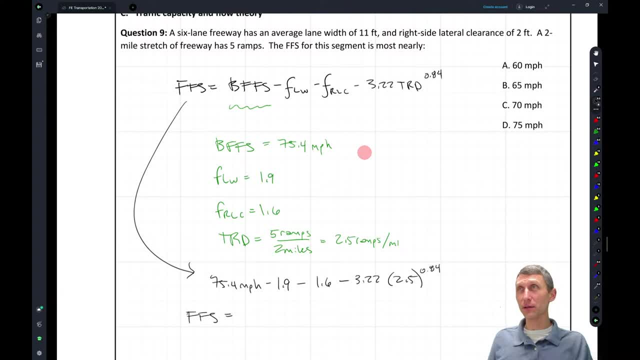 When I plug all this in, I think it works out to be pretty close to 65 miles an hour. So 75.4 minus 1.9, minus 1.6, minus 3.22 to the power of 0.84.. 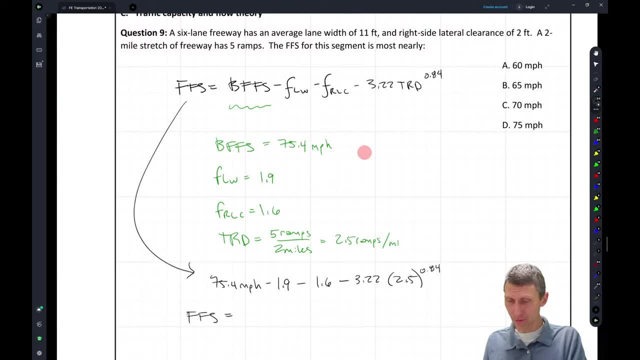 Yeah, or did I cheer something up? Oh, 3.22, I put it in wrong. So 3.22 times 2.5 to the power of 0.84. And I get about 64.95 miles per hour. 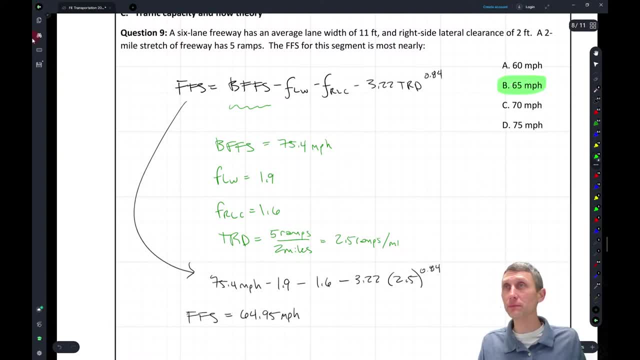 So I'm going to go with 65.. Okay, So, Matt, I'm not sure if you're still having issues with this, Delays, or not, but hopefully this is working and we're still going here. So it's been a long night and kind of a rough technical night. 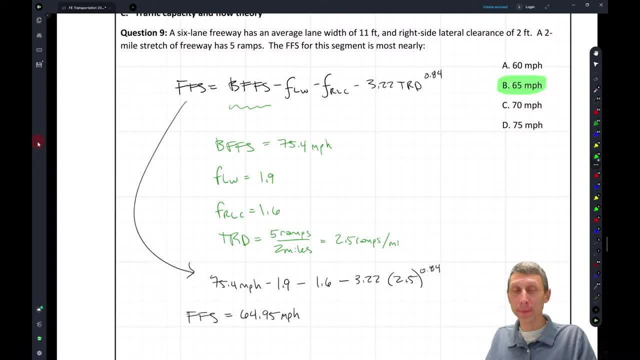 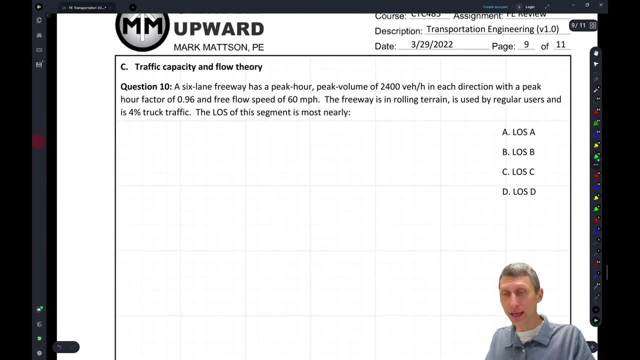 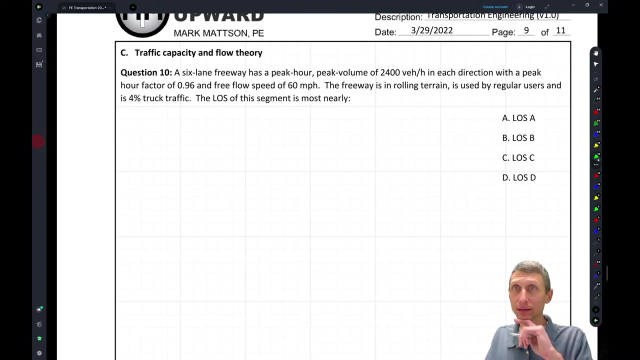 but hopefully it's still working for you out there. So let's keep going here. This next question is probably one of the harder questions I'll throw on here. It gets a lot of pieces in where we're going, So 30 seconds behind. 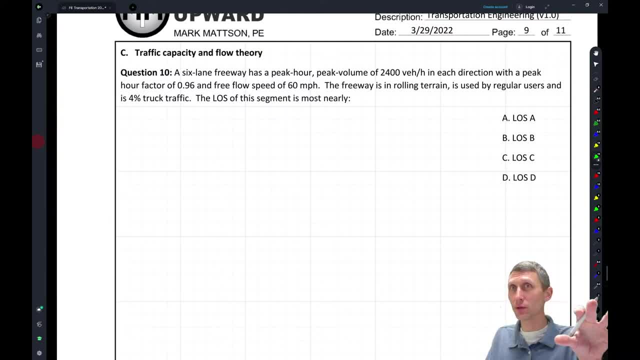 Actually there is a little bit of a delay. So the way that the stream works is, I think YouTube buffers me for a little bit And then sometimes I don't see it right away, So there's a little bit of a buffer going in there. 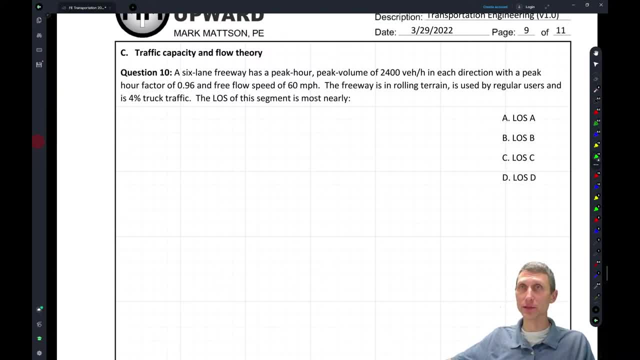 But no, just keep asking questions and I will respond to them as soon as I see them. So I keep looking up to try to make sure I'm following this, because it's just me. I mean, I don't have a team of people supporting me. 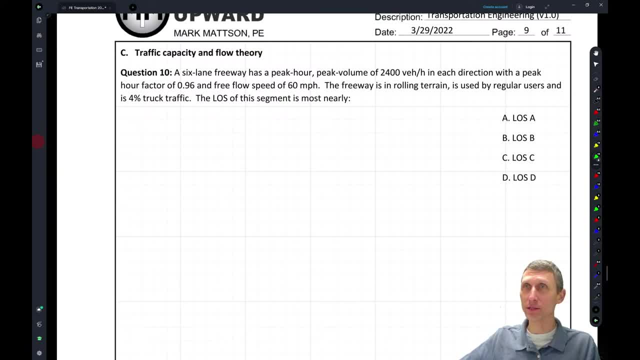 It's just me trying to navigate this, But I do appreciate the questions, So. So let's keep going. here We have a six lane freeway, peak hour volume: 24 vehicles per hour in each direction. If you got a factor point nine six, I'm going to keep going with these sales right now. 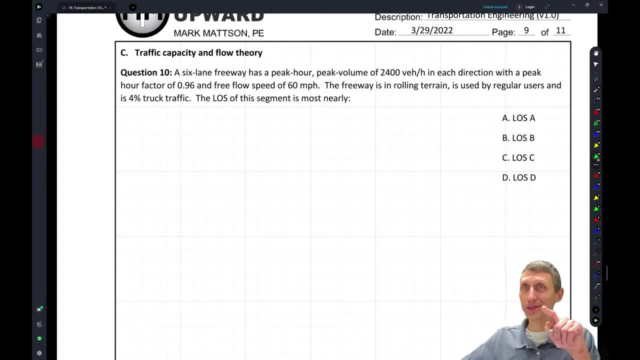 I'm not going to come back to that chart at this point, So sorry. maybe I'll throw another video out there for that at another point, But we're we're pushing time here, So let's just keep going at this point. But the e-sales: you basically look at each of the axles and what they give you and you add them all up. 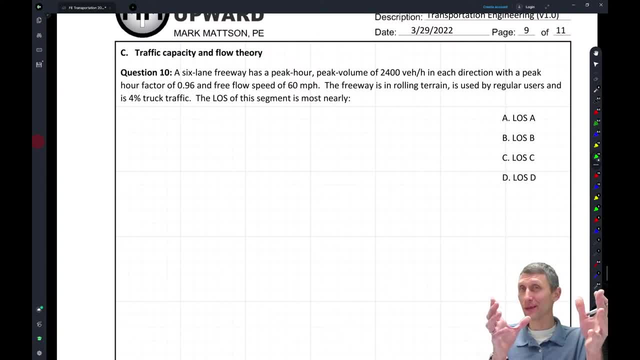 to to go And then you get an equivalent load. So so, just jumping, I guess, from this question for a second, those e-sales you're looking at. if you're told so many pounds per this axle, so many pounds for this axle, so many pounds for this axle, you're going to the chart. 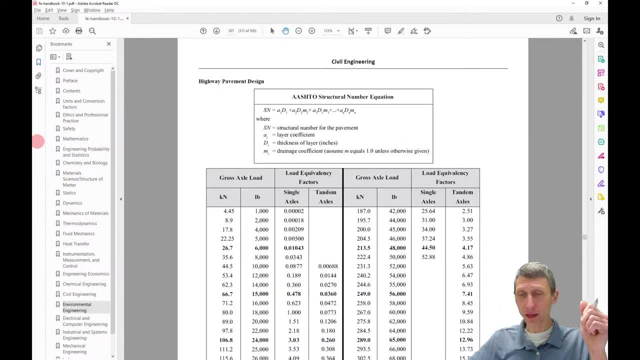 You know what. Let's just go there, Why not? You're going to the chart and you're saying: you know we have so many pounds for the front axle, you know maybe so many pounds for a tandem axle somewhere, And we're adding those pieces up. 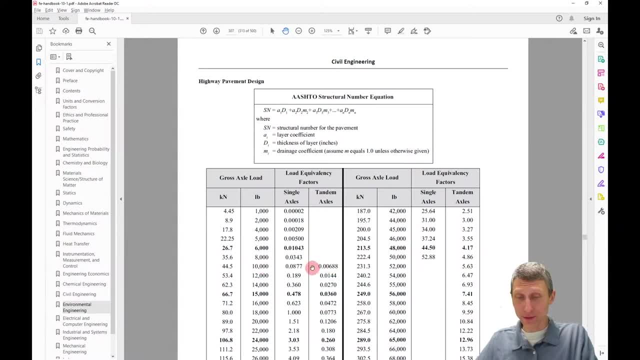 So we're going to add up. you know, if we would 10,000 pound single axle, you got 0.0877. or you know, 6,000 pound single axle, We got 0.01043.. 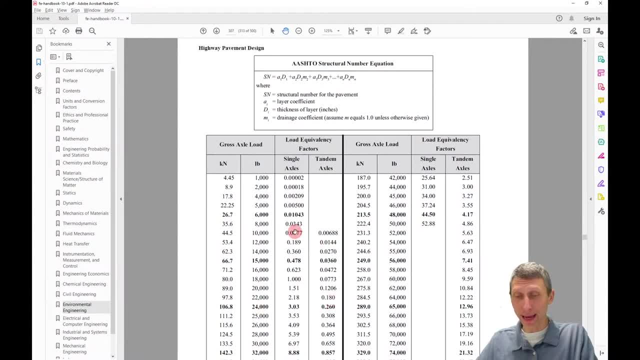 And then let's say we have a 24,000 pound tandem axle. We're going to add those pieces, add those numbers up, And that's going to give us essentially an equivalent, equivalent load. So that's like the three second version. 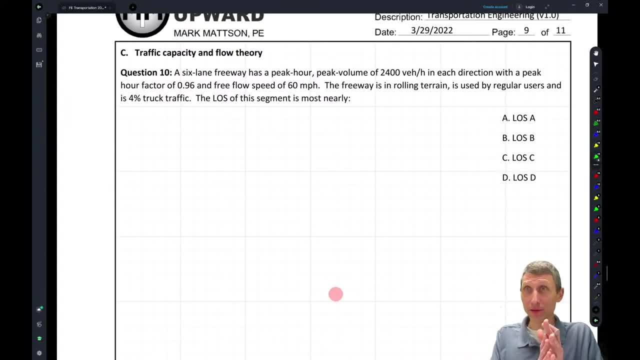 But let's keep coming here and keep going, So maybe I can get another video up with with a question with that as well. And so what do we got here? We got a six lane freeway. peak hour, peak volume: 24 hours. vehicles per hour, peak hour factor: right. 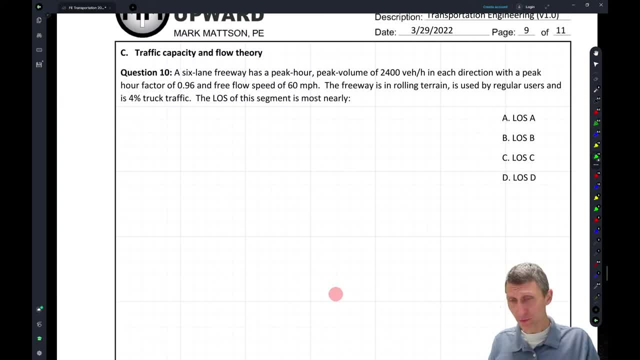 That's what we just found earlier in the session here. Preflow speed is 60 miles an hour, The freeway is in rolling terrain used by regular users and it's 4% truck traffic. What's the level of service? So level of service? we did see a table for that in here. 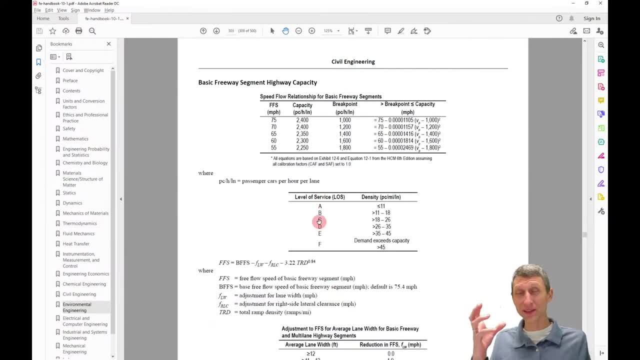 Level of service, What typically it's good to kind of know, but this is kind of the rating of the road, Like how, How people experience it and how much they, how, how happy they are. right, I mean, some people are happy because C's get degrees and then, honestly, C's pass the FV. 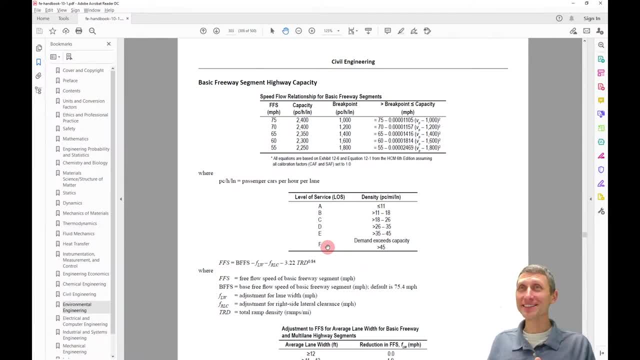 So if you can get 70% on the FV, you're doing great. So I don't know, There's not like a magic number, I don't have any like magic insight here, But typically if you can hit that range you're pretty good. 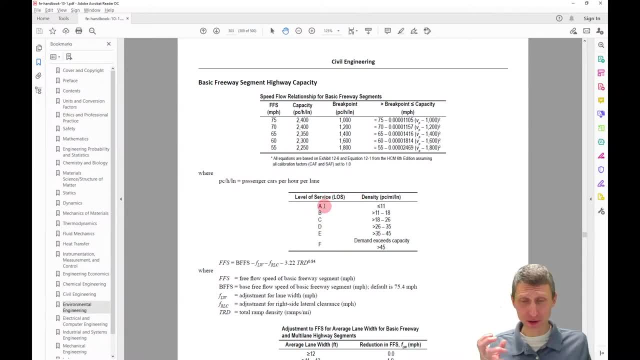 So where you are here, I mean typically, if you're an A, you're great, You got no problems. B's and C's are pretty typical. Sometimes D's And congested areas is easier as well. So what we're looking for is: what density do we have here? 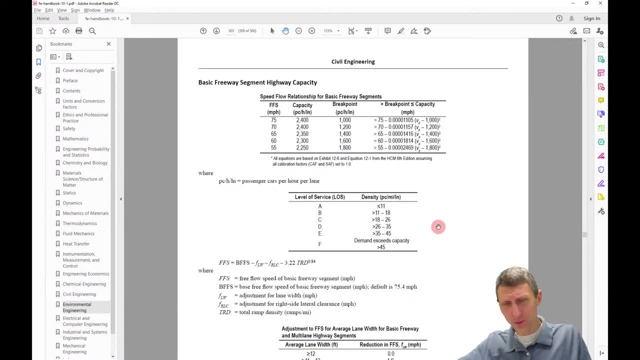 Okay, so let's keep coming here And but we have a density, We have a free flow speed, We have capacities. I mean, is that where we're going? No, because this just gives us the break point for kind of this, this, this density on here. 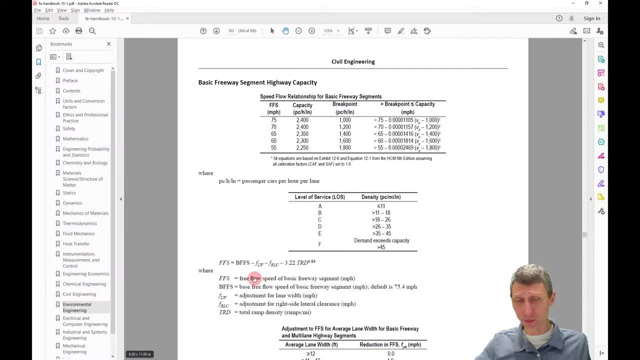 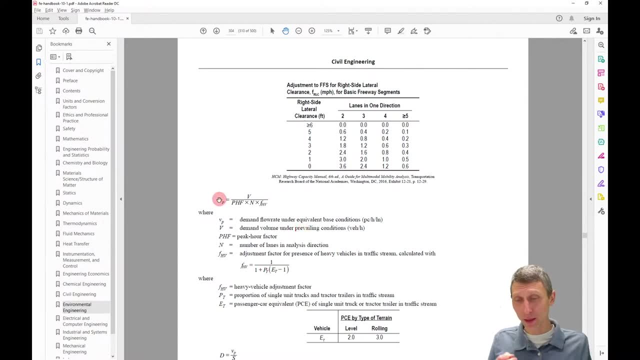 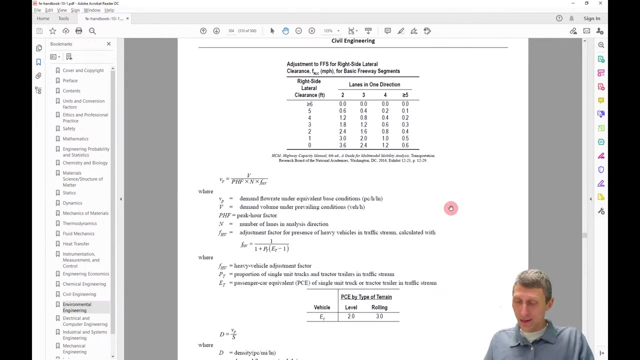 So let's just keep going as well, because we're told some other information. We have this equation, but we have to find the right equation. We also have this information about heavy Truck traffic. We have our demand flow rate here. We've got a bunch of things going on that's going to. that's essentially what we need to solve for. 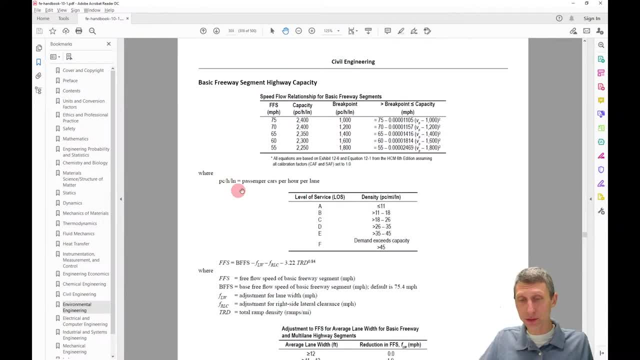 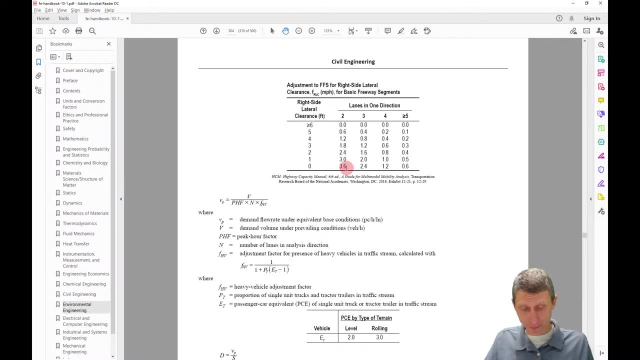 So we need to solve for this demand flow rate in order to come back to our level of service and figure out where we are. So let's, let's keep going through that. So we want to find that demand flow rate and then we want to find our density. 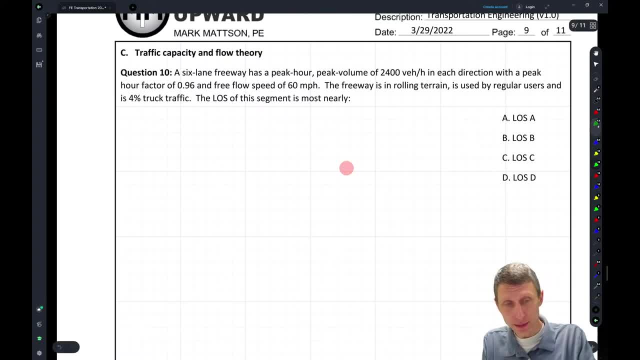 So I'm going to come back here. I'm going to say, let's, let's start with, let's just start with that demand flow rate. OK, the demand flow rate is equal to this little piece of piece times V, or sorry, equals V, over the peak hour factor times and times FHV. 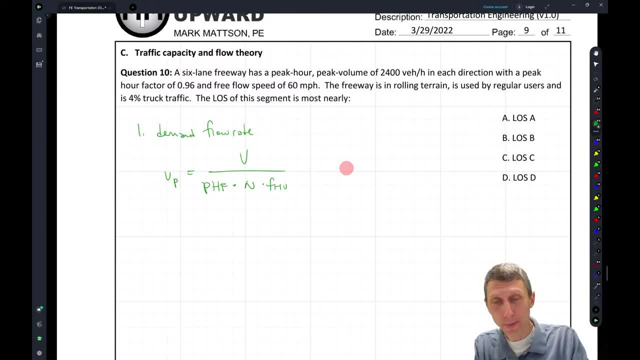 So we have some of these pieces right. We know we're told that the V Here is 2400 vehicles per hour. We're told that this is we were told the peak hour factor is 0.96.. OK, we have a free flow speed of 60 miles an hour. 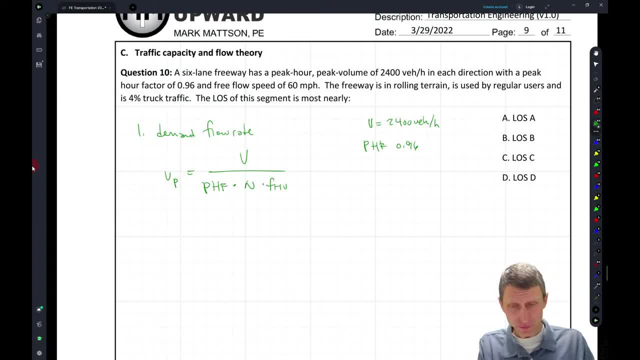 We'll get there eventually. And then what else do we have? We're told some other pieces like we have this six lane freeway, So we're going to say N equals. again, we need to know how many are where. we're going to this. 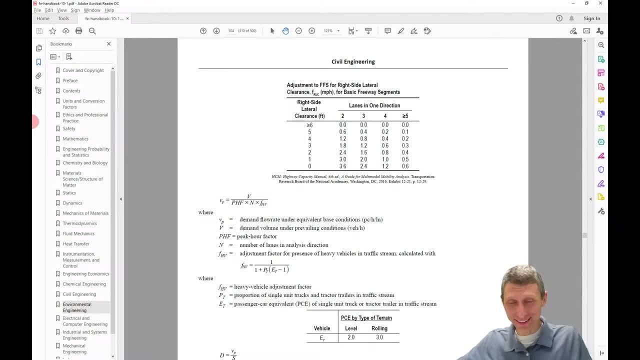 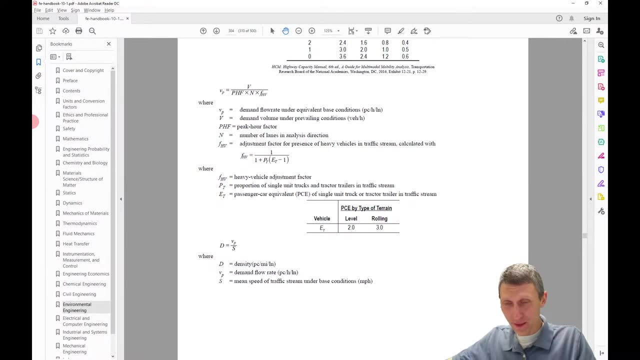 Um, Yeah, I think. yeah, there's certain places in the world that I think always have an F level of service, but what do we have here? We have a peak hour factor with, and the number of lanes in the analysis direction. 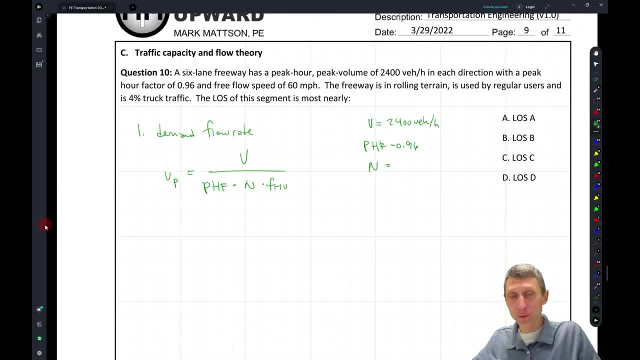 So we're just looking for one direction here. So we're going to come back, We're going to look at one direction. We're going to see three lanes in one direction. OK, this FHV we don't have, but we have to go solve that. 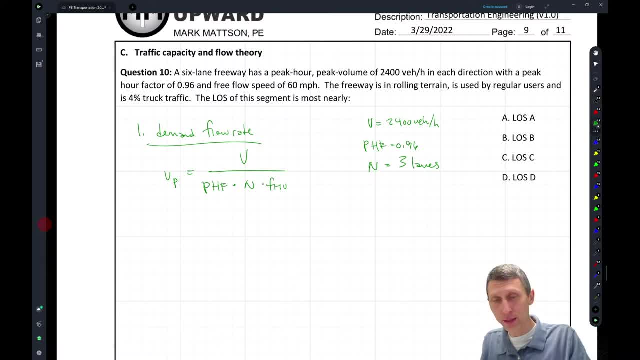 So, Before We can solve for this flow rate, we need to solve for, you know, solve for FHV. So maybe I should really call this number one. But what's our what's, what's our FHV, Our FHV? here is another formula. 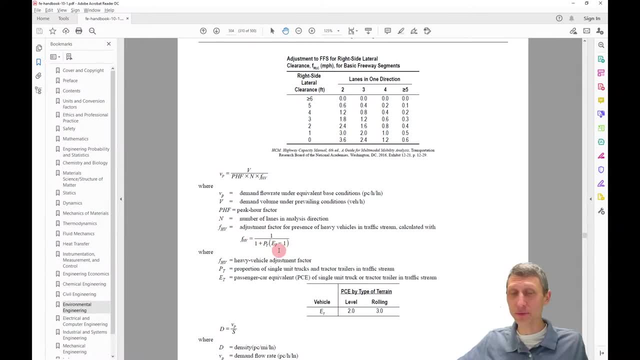 So again, I tried to fit a lot packing a lot, into these problems. But we have this other formula where we're having this: this PT, their portion of trucks, and ET, the type of train, So three. So we know that the percentage of 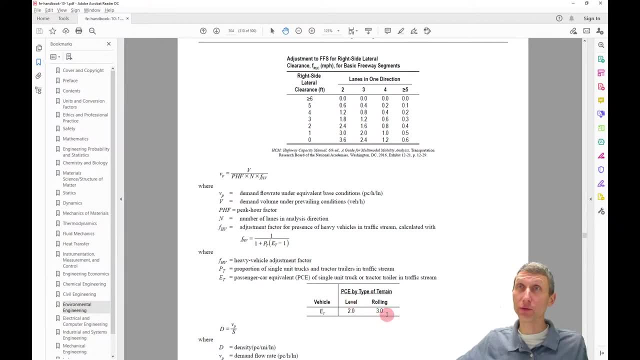 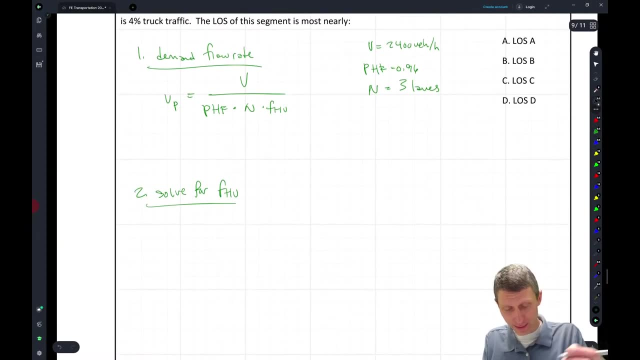 Trucks was, I think, four percent in the rolling train is going to be this: this three here. So let's come back and find that, But let's write that formula down here first. So I'm going to take this formula and I'm going to say the FHV. 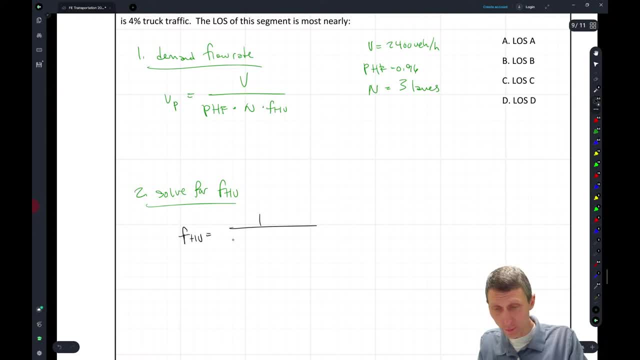 The heavy vehicle adjustment factor is going to be one over one plus PT times what ET And minus one. So this is going to be one over one plus zero point zero four. So that's our, Our truck traffic times. three minus one is going to be that three is the ET. 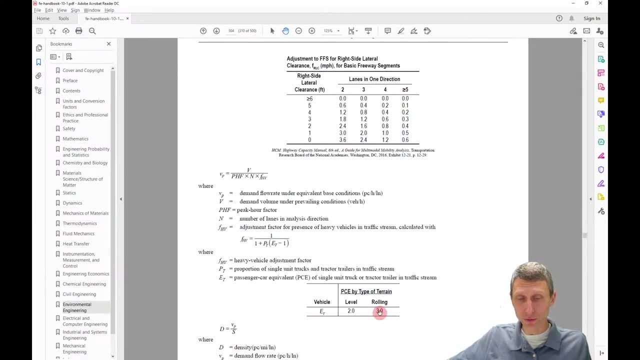 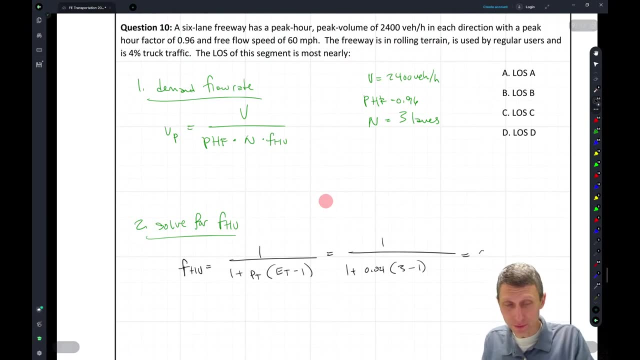 So if you remember that, since we're enrolling terrain, we're going to use this three point zero And that's going to give us a value or a heavy vehicle adjustment factor of zero point nine to six. OK, and then we're going to come back up here. 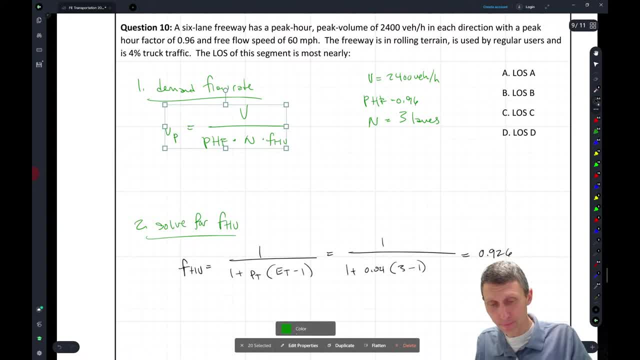 I'm just going to change this for a second, Because I like to do my my equations in black here. So so now we can solve for this as well. So now we know that we have twenty four hundred vehicles per hour- OK, divided by zero point nine six times three lanes. 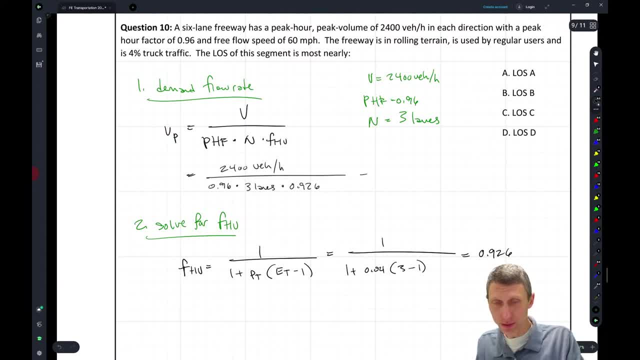 And times zero, point nine to six. so this demand flow rate Works out to twenty four hundred divided by point nine, six Divided by three divided by point nine to six, And I got like right about nine hundred. And let's look at the units. 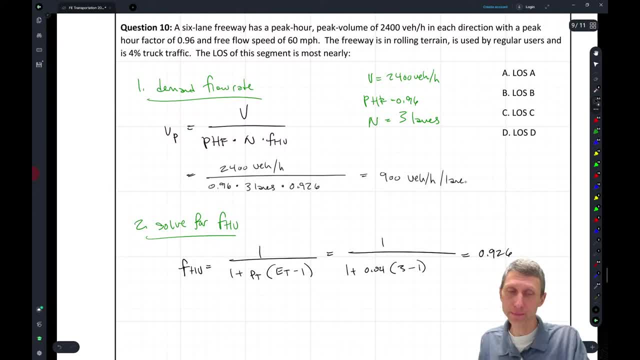 What we get here is vehicles per hour per lane. OK, so our units stay with this: vehicles per hour per lane, And that's our unit. So in a perfect world, we just come back to our flow, our level of service chart. 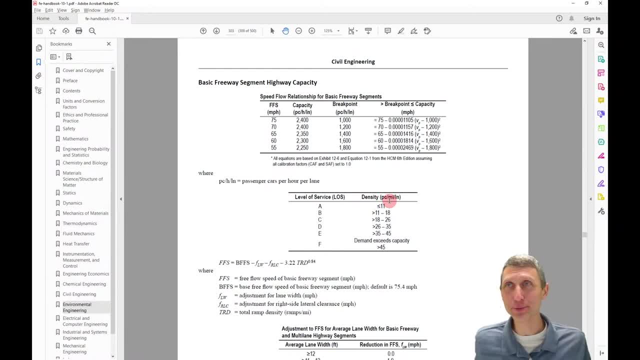 We come in here with passenger vehicles per hour per lane, But what you see here is we have units problems, right, We have passenger cars per mile per lane. Oh, what do we do? We can't just use nine hundred, and nine hundred doesn't make sense. OK, 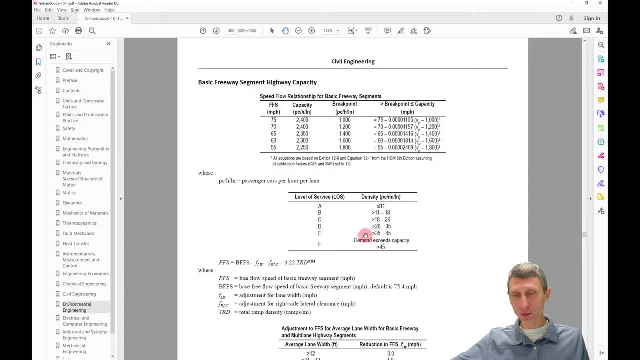 That doesn't work here, But what we do see here is we have this, this idea here where we can come up with our level of service, and specifically what we're going to do here is we're going to, we're going to find the density. 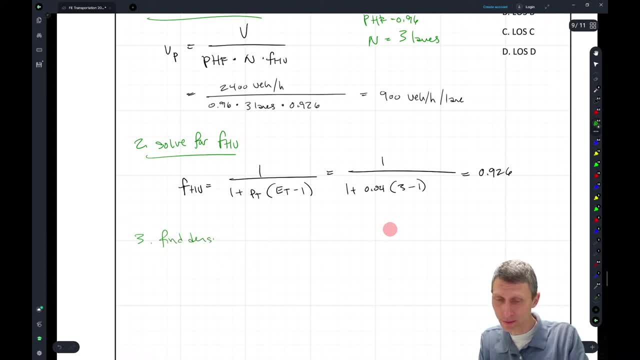 But we're going to find our density. We're going to find our density. How are we going to find it? Remember what we said the last time: the density. this density equals what density equals? the flow rate divided by the speed, or really, the way we did it the last time, was the flow rate. 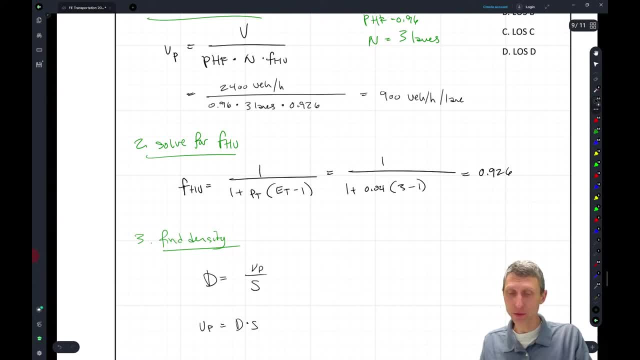 What we said the last time is: the flow rate equals the density times the speed. So we're going to rearrange that up here. But that's one of those basic formulas like Q equals AV, and when you're looking at fluids, like Q equals AV, right, this is kind of a similar idea. 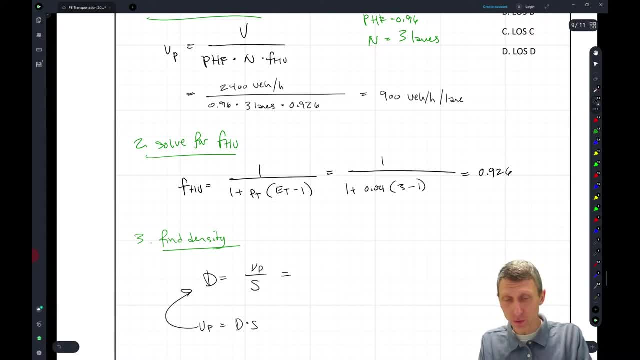 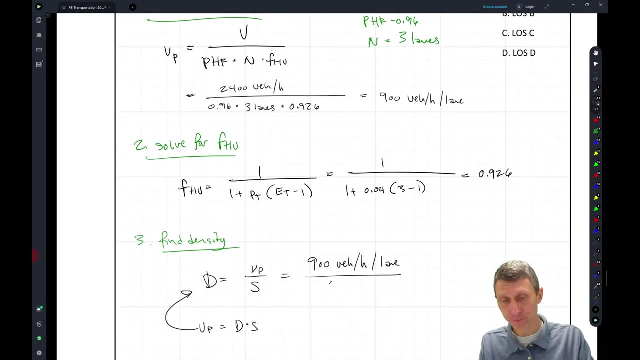 This density equals flow rate divided by the speed. So what do we get here? We have nine hundred vehicles per hour per lane divided by our speed. And what's our speed? That's where we get our free flow speed up here of 60 miles per hour. 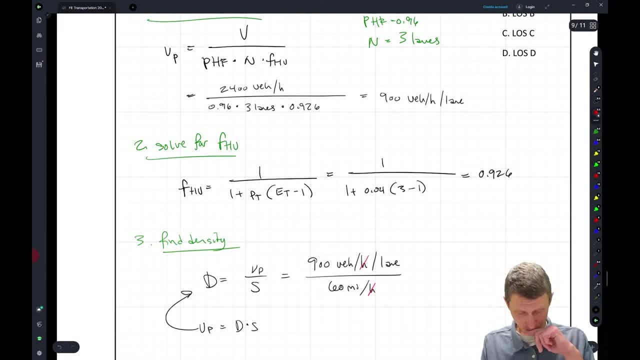 So the good news is our hours drop out, OK, And what else do we get? We get when we solve this. now we get 900. over 60 is going to give us about 15 vehicles per mile per lane. OK, And that's a number now we can use, because that's what we were looking for. 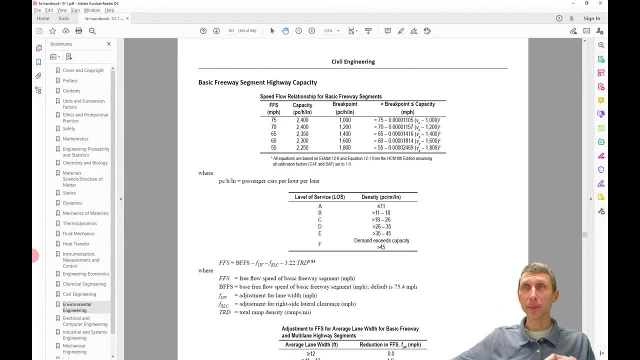 We're looking for this density, but we had to go to flow rate first to get there, So is this problem really going to be on there? Probably a little bit complicated, But honestly, I wanted to get some of these concepts in there, especially that the relationship. 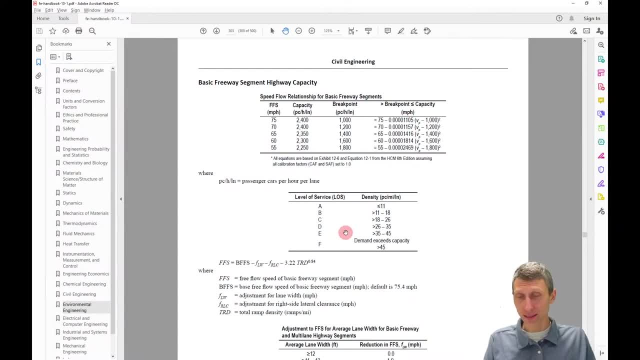 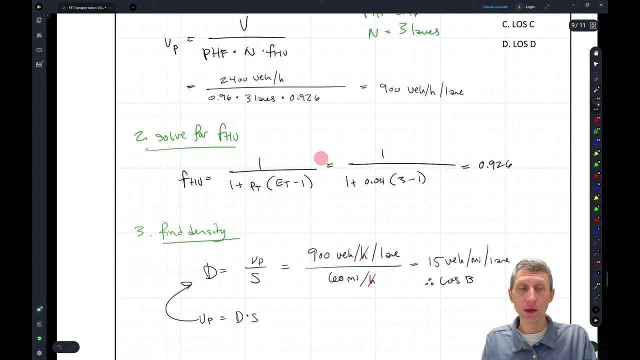 between flow speed and density, just to hit on that just again. Right, But that's where we get into this 15. We're solidly in a level of service, a level of service B. OK. So you know, therefore, LOSB, and we can circle that one. 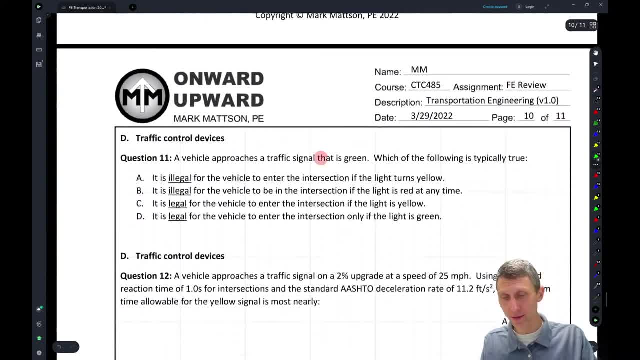 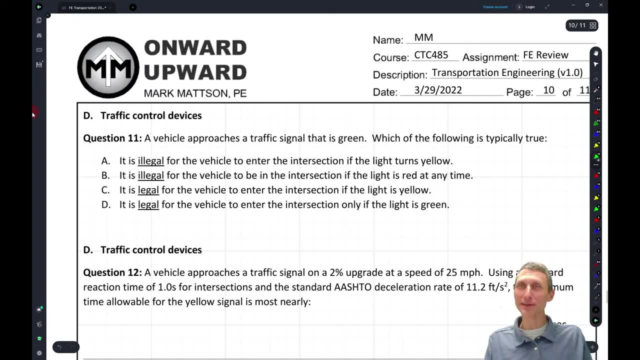 OK, well, let's keep going here, and this is one of my favorite questions, not really, but sort of: A vehicle approaches a traffic signal that is green, which is the following is typically true: The one of the reasons I love, I love this question is it's. it's one of those questions. 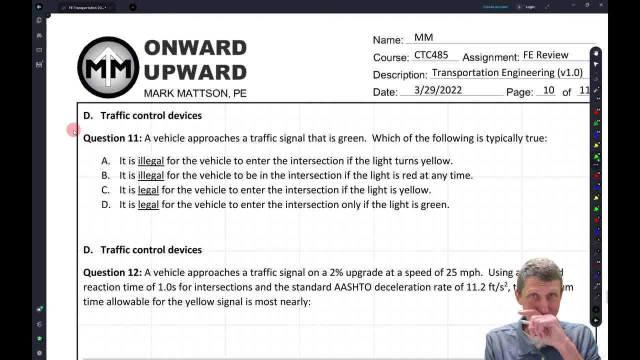 that I ask how many of you have driver's licenses, You all raise your hand and I say: how many of you know the answer to this question, And there's a little bit of scratching your head going on. I think I'm like, ah, what is it when you approach a traffic signal that is green? 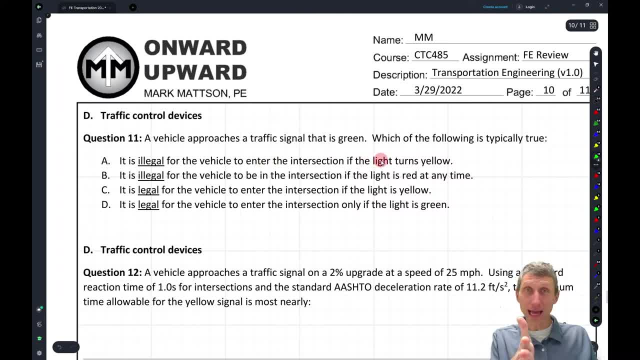 Is it OK to enter the intersection if the light turns yellow? So if it's yellow, is it OK to enter the intersection. Is that illegal or legal? OK, So is it legal or illegal? Is it illegal to be in the intersection if the light is red? ever. 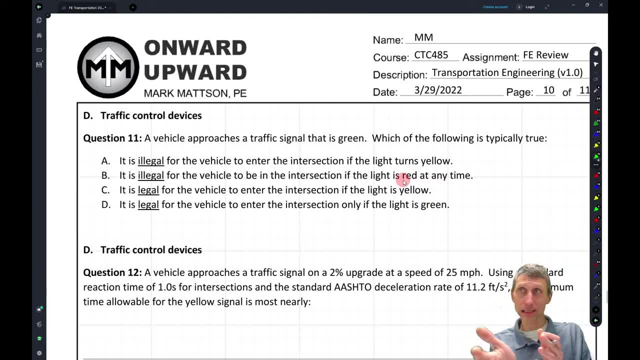 OK, so maybe you can enter it when it's yellow, but can you be in it when it's yellow? Is it legal for the vehicle to enter the intersection if the light is yellow? So it is legal. So it's either illegal or legal. 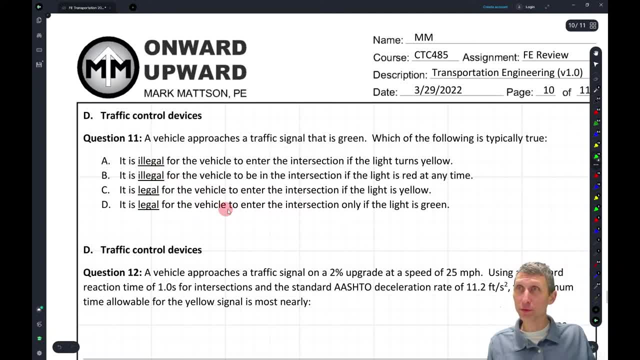 Which one's true, We've got to pick. And then is it legal for the vehicle to enter the intersection only if the light is green, So you can't go in if it's yellow. So there's. there's some of these kind of repeats here. 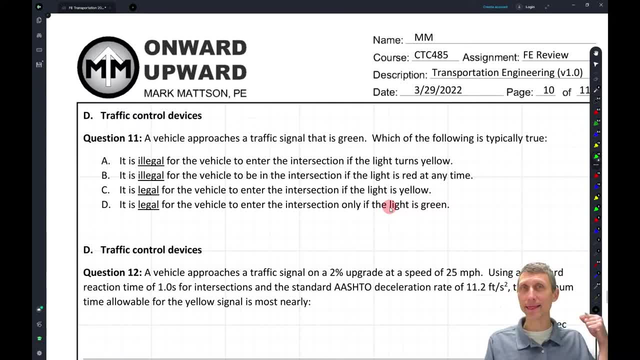 The wording is a little funny. I was going to just put in: what do you do when you see a red light? Hit the gas. But that's not good advice, So I didn't want to put that in there. I just thought it was funny because it's true. 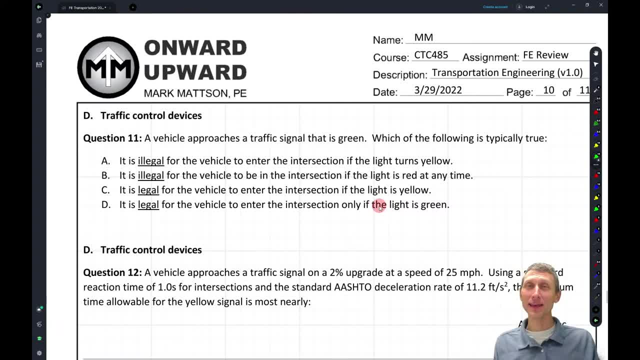 Many times. what do you do with the red light? Maybe not you, Maybe the person next to you that's telling you you're number one with only one finger? You know there are people that do that in the car. I would not ever recommend that. 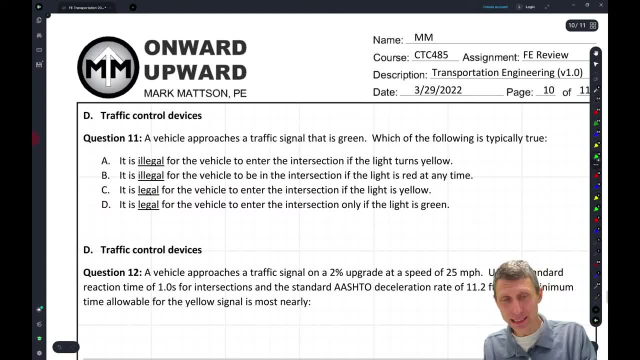 But the idea here is: I'm going to say that this, this, this C is typically true. So, typically, what would go well now? So what, typically, what are we doing Typically when you see the yellow light should be long enough so that, if you, if you're, if, 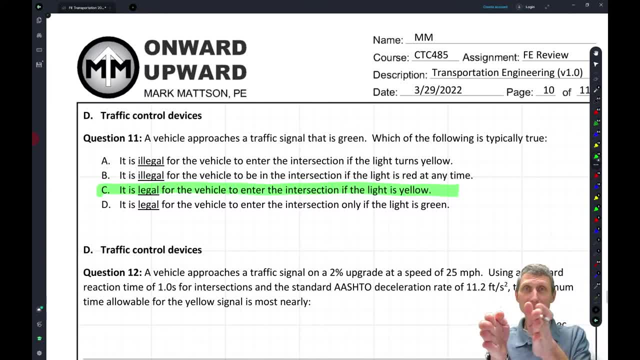 it's green. you see the yellow light. you're far enough away, You have enough time to stop before you hit the intersection- The yellow light should be timed long enough for that- And if you're before that, if you're past that point of no return kind of point where 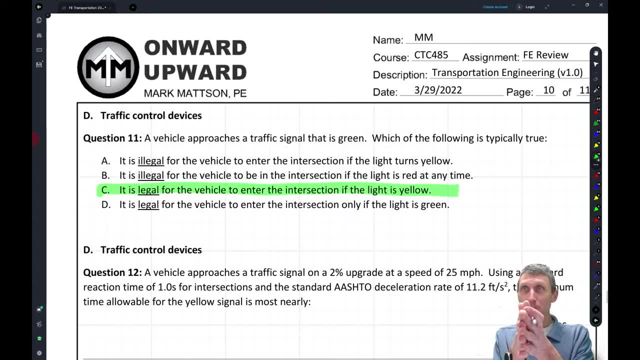 like: well, it's yellow. If you're before that intersection, right then, you should have enough time to get through the intersection. But let me ask you this question: So is so, isn't B true, Matt? that's a good question. 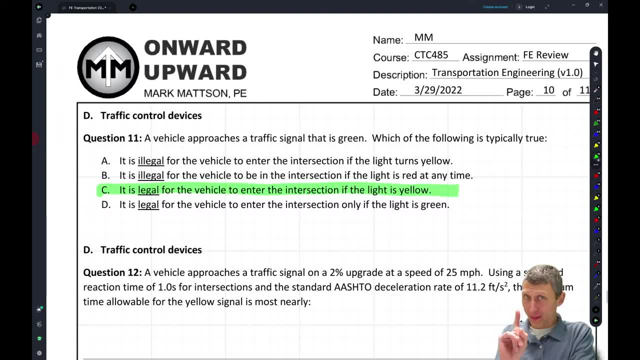 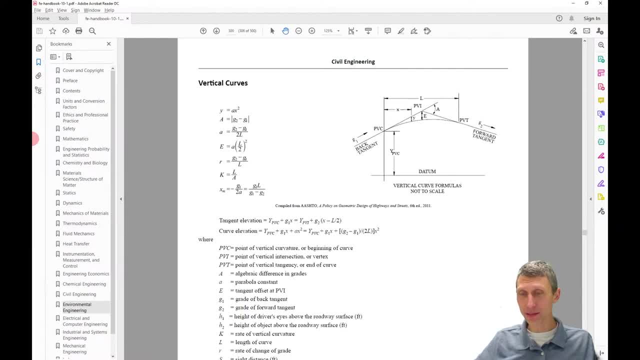 Isn't B true? Oh, why is B false? B is false because in when we get into our signal timing in here, let's come back to signal timing. Do you see what? this, not that one? Where is it? Do you see what this is? 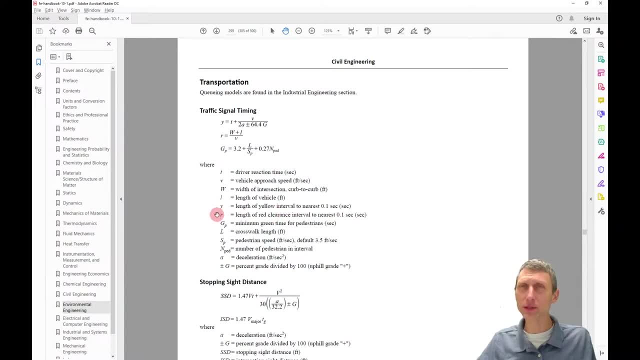 This is our. That's our the length of red clearance interval. What's the red clearance interval? The red clearance interval is when the intersection is red on every single side right To allow cars that entered when it was yellow to pass through. So there's going to be a red signal time. So, like typically your yellow times in two to three second range, typically there's a one second all red time to give those cars that entered when it was yellow a chance to get out of the intersection before. 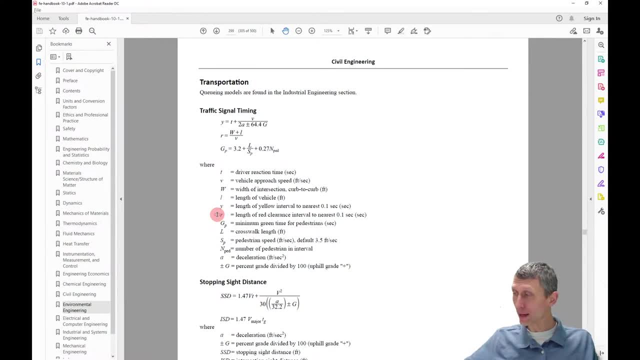 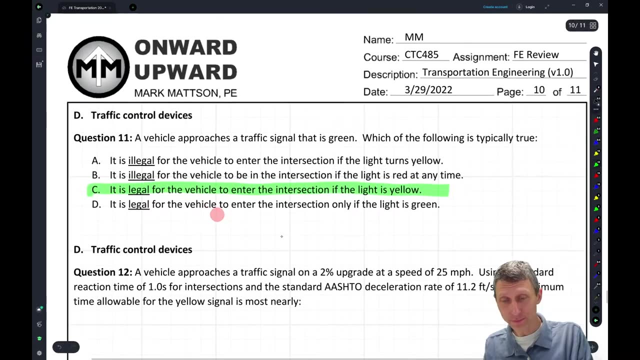 Yeah, And the other lights turn green. So that's why B is false. Like typically, it's like you, let's say you know you're driving along, you know you're driving along here and you enter the, you know it, the, you know you're, you're at. 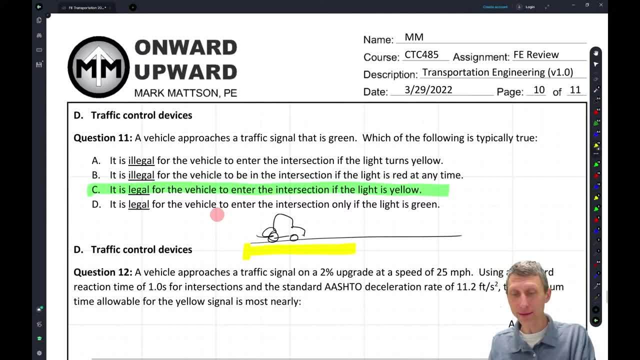 this point in the light turns yellow. Well, if you're already at, well, actually that makes no sense. Let's, let's try it, Let's try to draw this a little bit better. So, if you're, if you're driving along and you know it's green, green, green, green green. 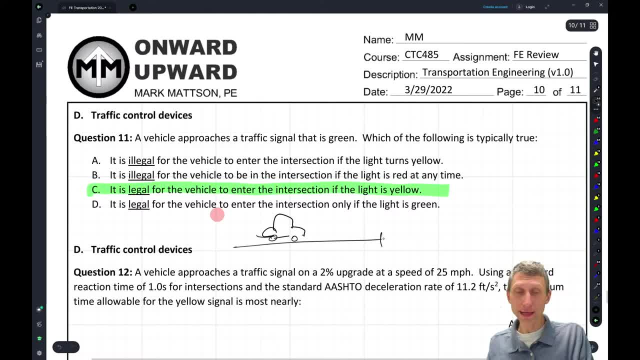 green And you're like right next to the intersection and it turns yellow, but yellow keeps going until you reach this point, right, And then it turns all red for until, essentially, you leave the intersection. So there it's. it's meant to be kind of this idea where, if you're driving, I mean let's. 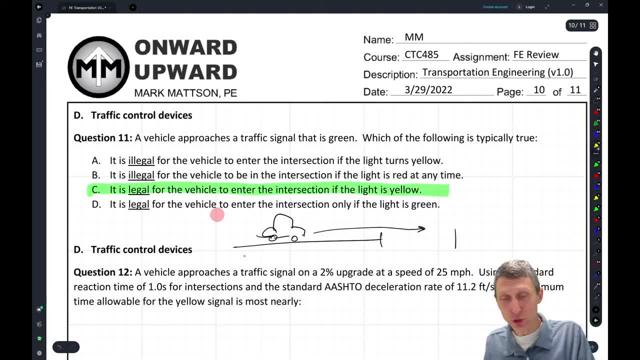 let's push this back a little bit. Let's say that you're driving and you're super, super close to the intersection And as soon as you hit the intersection It goes to red. In theory, you should have enough time to get through that intersection and back out. 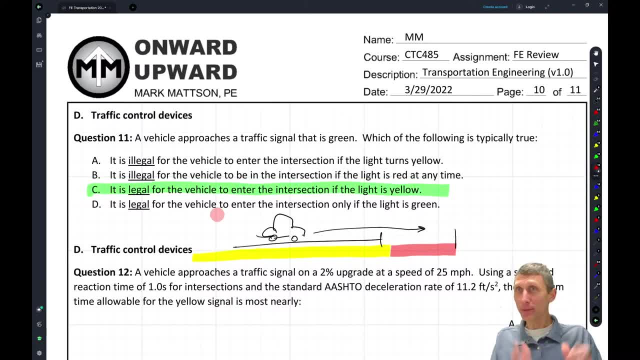 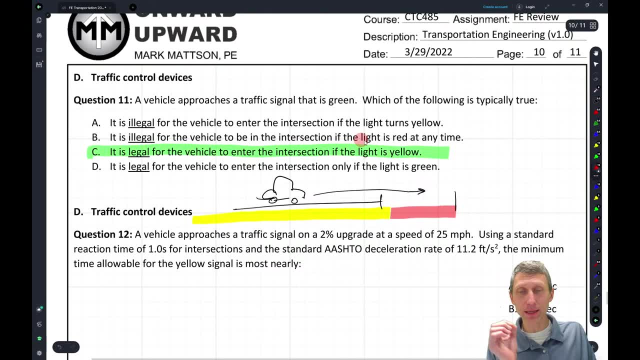 and still be legal. I probably didn't explain that wonderfully, but I tried, So typically I'd say it's legal to enter the intersection of it's yellow It's. it is legal to be in it because there's that all red clearance time. 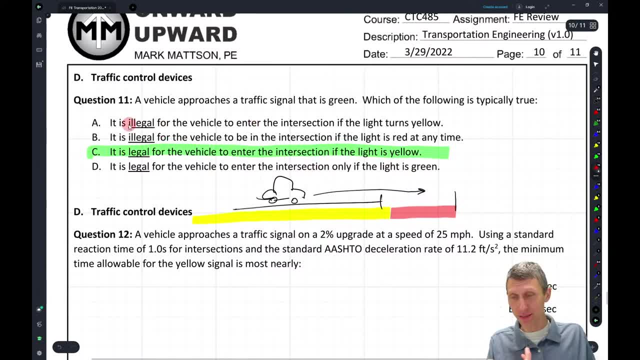 You can enter it if it's yellow, So that one doesn't make sense. And this one, this is kind of like a repeat of D, So it's like these are, these are kind of the same, I don't know. 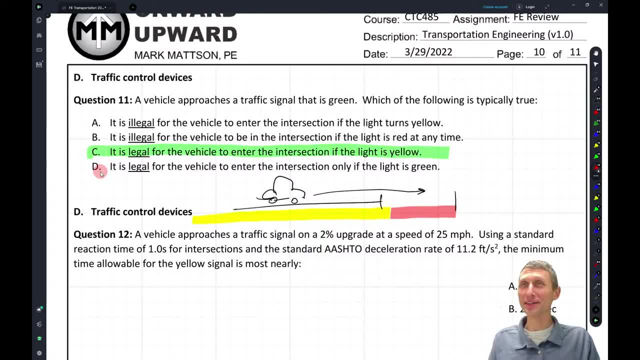 I can't explain it to a trooper. You know, I I did have a conversation with a trooper once where I got pulled over. there's a new roundabout put in and I, sort of like, went up to it and I I saw this trooper come. 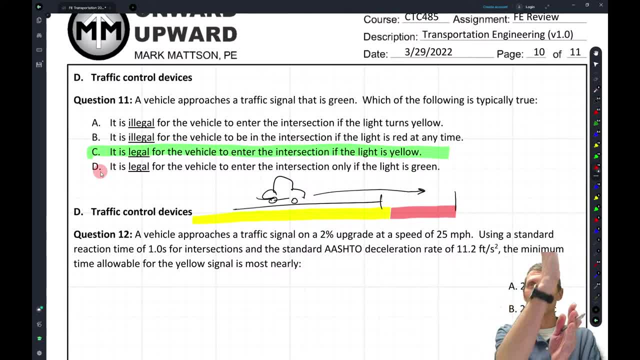 in. I actually saw a police officer, He's coming. He was coming around and I thought he was going to continue around it, So I started to nose out a little bit, but then, then I think he, he, he started to turn. 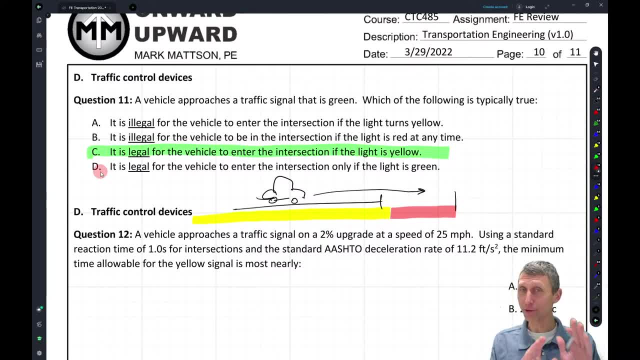 So I stopped. I just 100% legitimately stopped. I never entered the, I never actually entered the roundabout, I just stopped. But then he stopped And then he waved me forward and then I went forward and then he followed me and pulled. 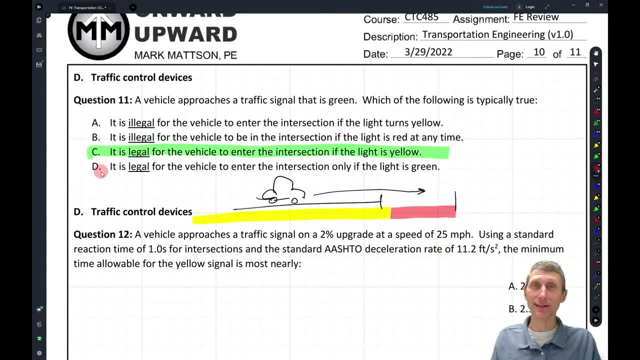 me over And I was like he's like you realize you're supposed to yield at an intersection. I said I did yield, I actually stopped And then he let me go, which I was surprised I was. my wife was like Mark, don't contradict, don't contradict, don't contradict the trooper. 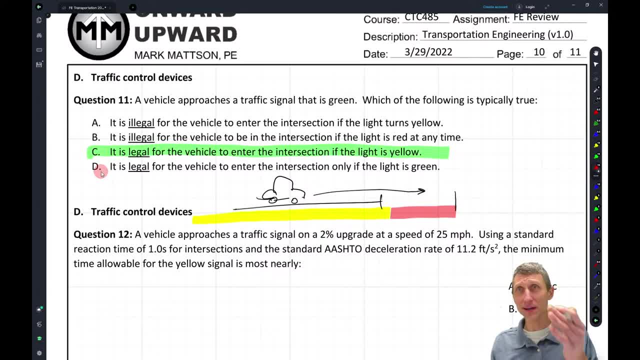 But you know I was like I did stop So. so, Austin, if you want to download, there's a link to my website. There's, there's some you can. you can get these videos. There are the, the, the, the, the paper copies as well, if you want to download these to. 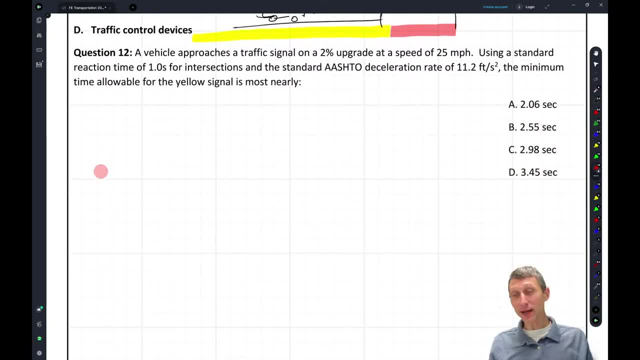 follow along. Okay, Let's keep going. So, as we talk about this, we do have yellow, yellow stopping times, And that's one of the ones. I mean. maybe you'll get a red time, maybe we'll get a yellow. 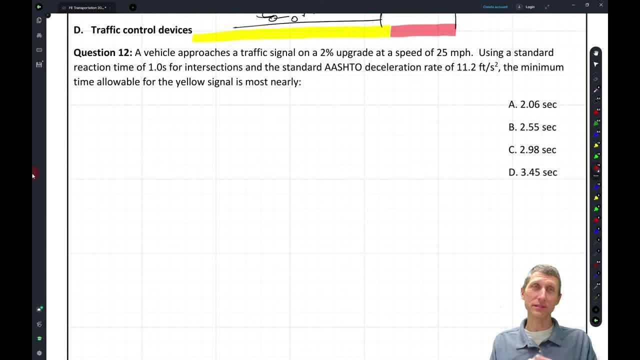 time I honestly the green and like proportioning ratios is going to be. that's a more complicated problem. I, you know, when I taught this class, I went through and I we went through that process. It's a little bit more complicated and proportionate and you need a lot more information. but 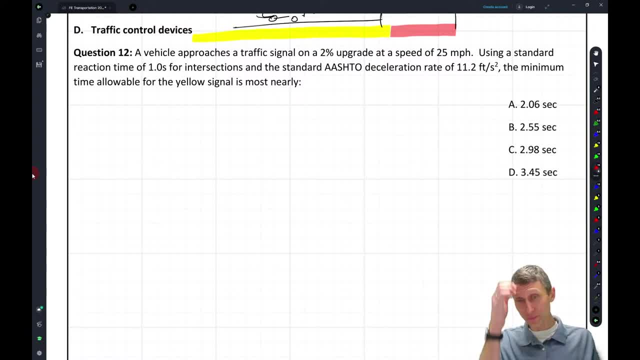 something like yellow stopping, yellow time is is doable, And the interesting thing is yellow just uses the stopping site distance, but it's it's in its own way and it's in its own units. So let's come back to this. but we have a vehicle approach to traffic signal: 2% upgrades. 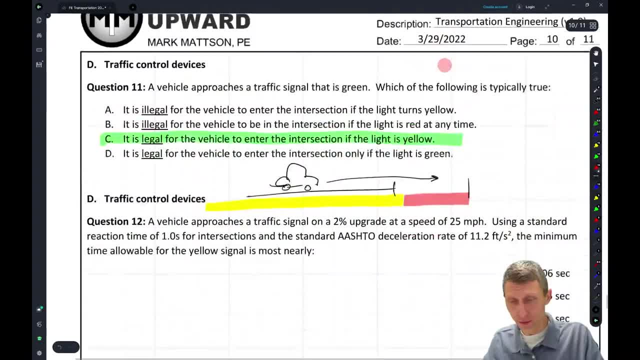 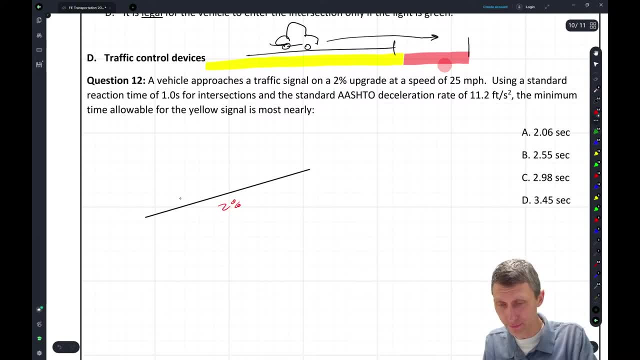 to be the 25 miles an hour. So where'd that go? So we have a 2% upgrade and what else? 2%, Yeah, So we're traveling at 25 miles an hour. And what is the yellow time in here? 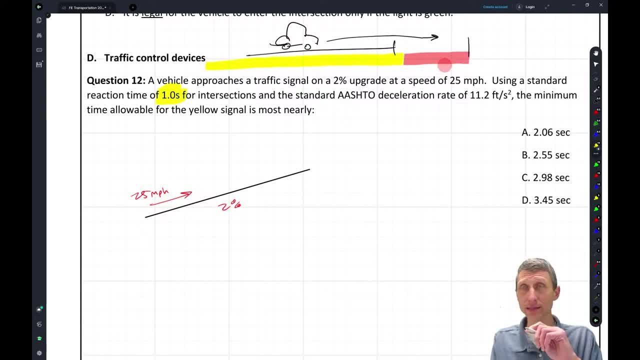 You'll notice that we have a reaction time instead of, like the stopping site distance for a vertical curve where it's an unknown object that kind of enters in to the intersection. here You're kind of expecting it. So the the reaction times, typically less acceleration. we're still using that 11.2,. 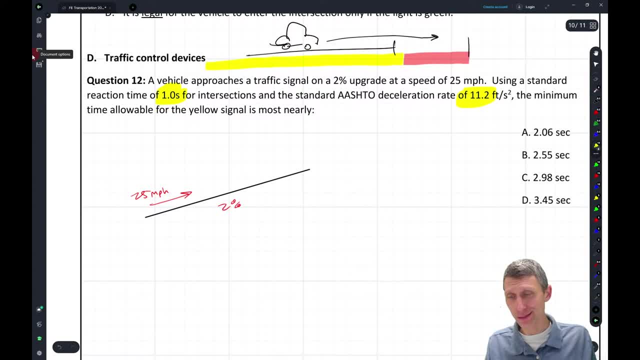 like we did for our stopping site distance And what is the what's the minimum time to allow A car to stop safely. So, in other words, this car is driving along and you know what's the minimum time that this car can stop. essentially, 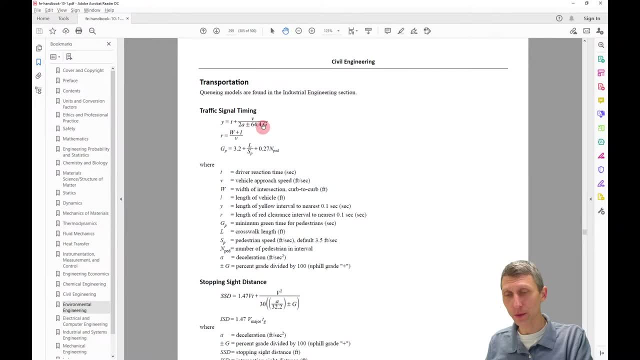 So what we're going to do is it's- it's essentially this, this formula up here, which is essentially the same thing as this, but it's a little bit different and it's like: this is a time. Why is it time? 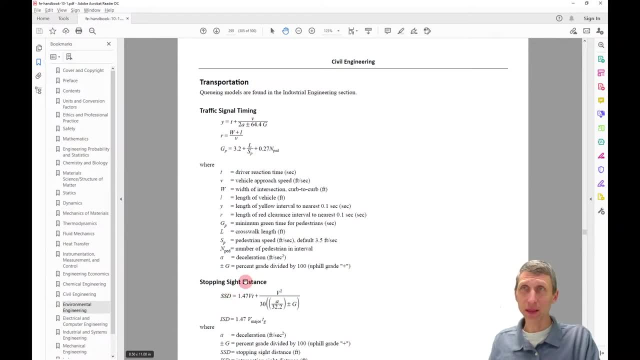 Right, This is a time where this is a length, but they, they both kind of work off the same principles and they're, they're very, very, very similar. When we get through this, Yeah, When we get through this, it's just, it's, it's. it's interesting here because the variables 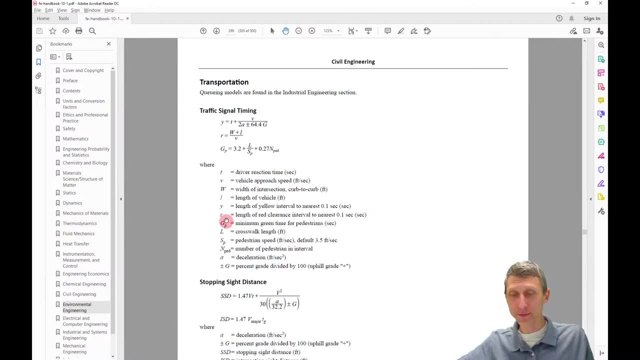 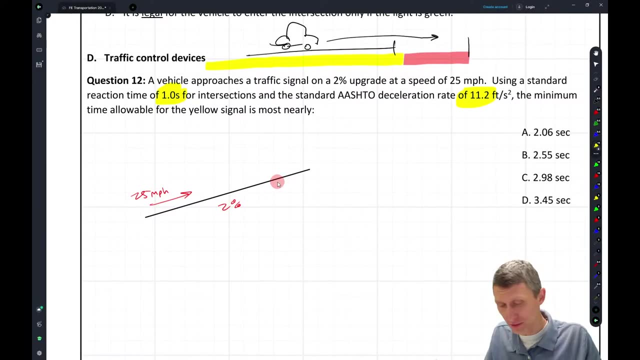 are different. here We have V in miles an hour, here we have little V in feet per second. So the units on these are just: oh man, they're, they're, they're killer. So let me just write down that formula and we will, we'll, we'll, we'll, figure it out. 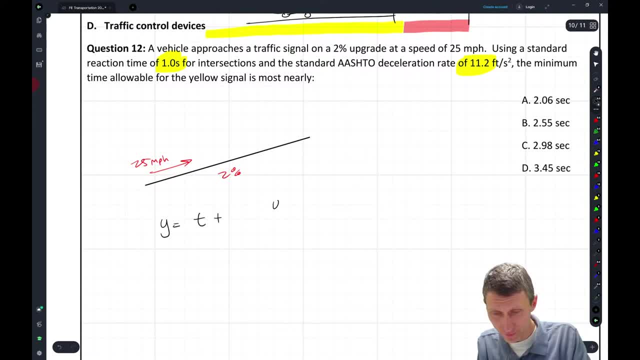 So Y equals T plus, you know, V- I'm going to do a little V there- divided by two, a plus or minus, 64.4 times G, and and then we're you gotta remember, this is the speed, This is the speed, you know. approach speed is in feet per second. 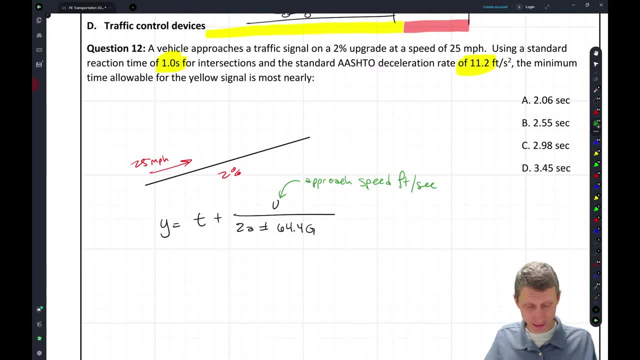 Okay, Oh man, it's just it's, it's, it's, it is what it is. So let's go through here and find out what those things are. So Y equals T, this is a one second. that's the driver perception reaction time. 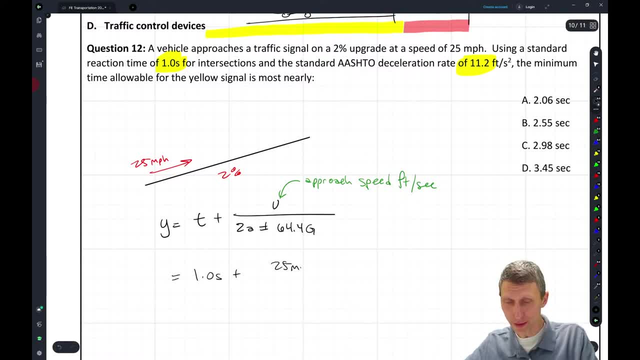 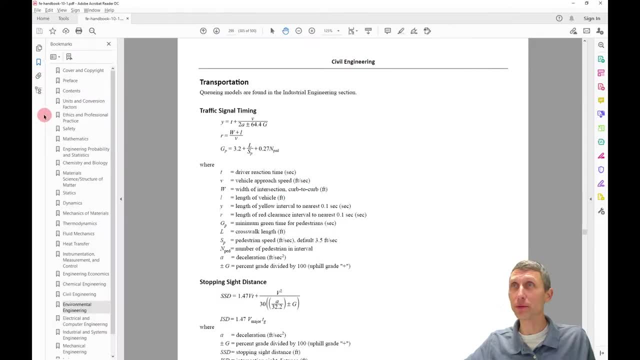 Okay, We're going to add in what's our speed? 25 miles per hour. Okay, And I need to convert that And and you might remember- I don't know if anybody remembers, but this 1.47 is that- 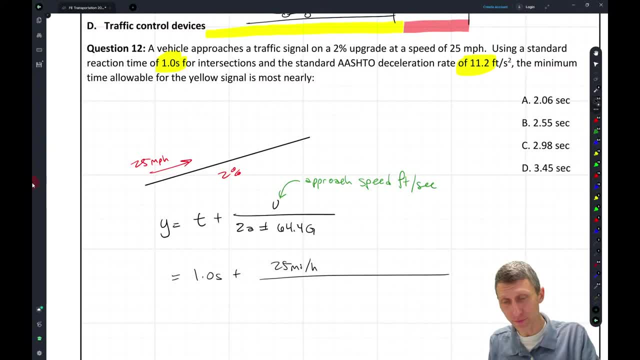 conversion. Okay, That 1.47 is conversion from miles an hour to feet per second. How do we get there? Well, we say: there's, for every one hour there's 3,600 seconds, And for every one mile there's 5,280 feet. 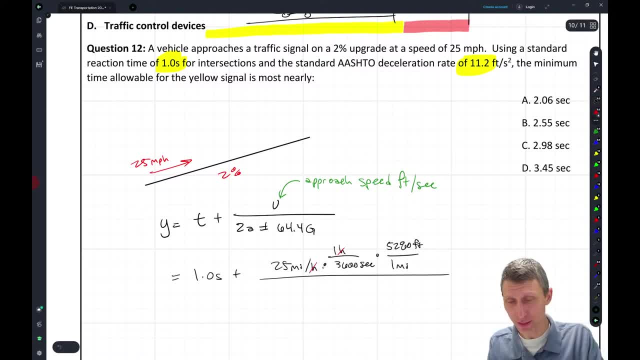 So those are some of those conversions that are good to just remember, because our hours cancel out, our miles cancel out And if you take that 520, somebody, you can check it if you want to. but 520 divided by 3,600, that should equal 1.47.. 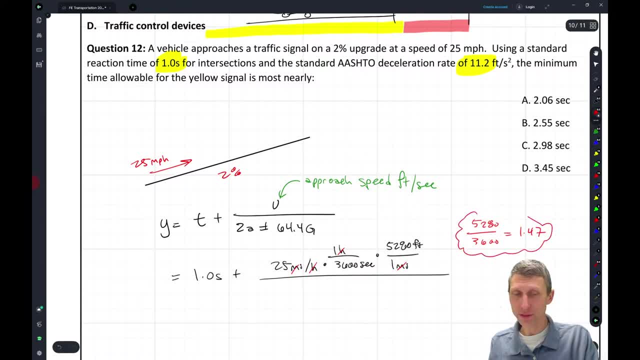 So that's where that conversion comes from. right, That's that conversion. And then we need to divide by what? two times our 11.2 feet per second, squared, plus or minus our 60.2.. 64.4,. well, in this case let's just do a plus, because we know it's an, it's an upgrade. 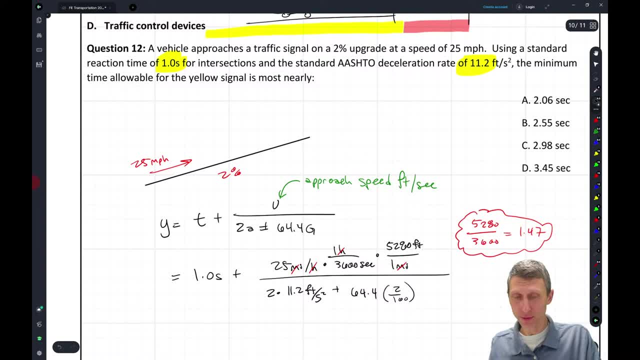 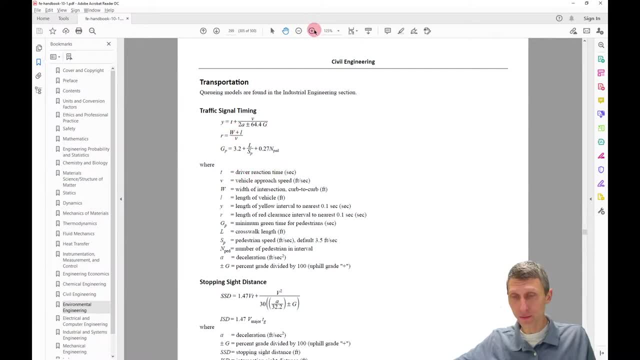 and we're going to say our grade is two over 100.. Okay, So let's just go back and check our units. Our T here is going to be time in seconds. Okay, What else Our A is going to be to tell us our deceleration in feet per second squared? 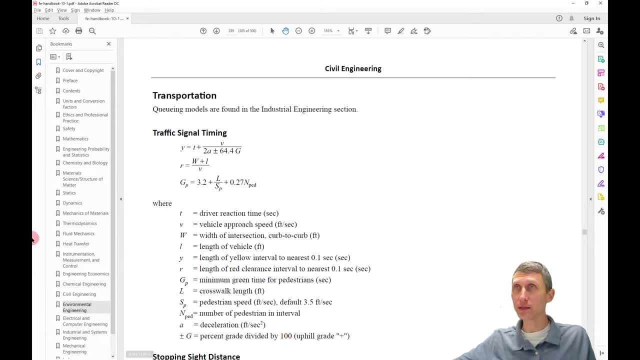 Our G is our percent grade divided by that 100 again. So that's, that's nice to know. So so we have this. this is good. I mean, here we have minimum green time for pedestrians, We have a red time. 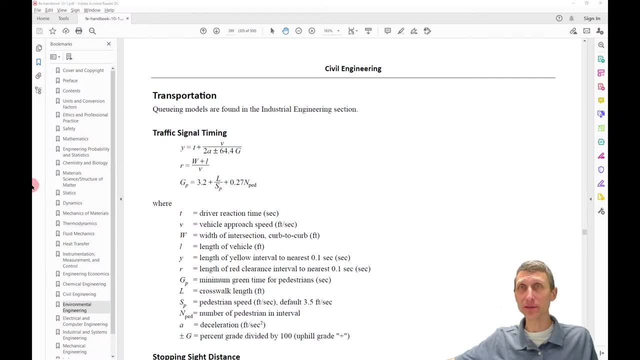 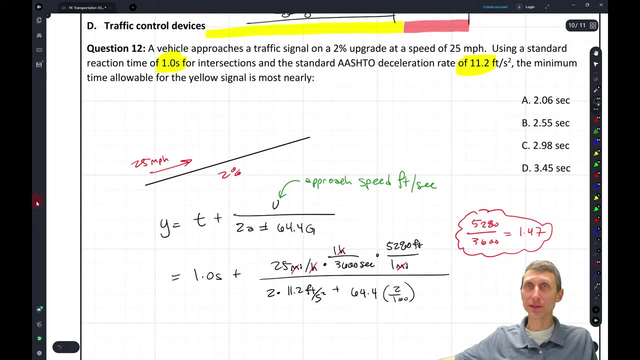 You could be asked any of those I just picked why? because the units are kind of kind of interesting. Why is deceleration positive? Because it is. I mean, that's a good question. I wish I had a better answer. serious, I wish I had a better answer. but yeah, it's, it's. 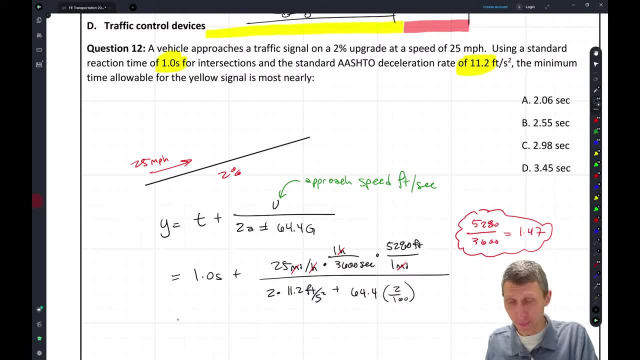 it's. it is what it is. That's the deceleration rate. Okay, So when we plug all this in, though, what do we get? We get one plus 25 times 5280, over 3,600 divided by two, divided by 11.2, actually 90 parentheses. 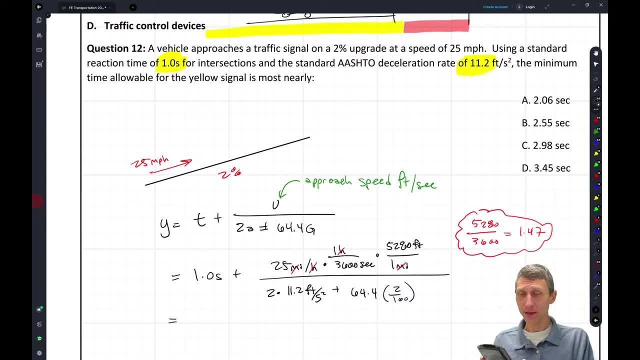 in there. So it's worth trying these with your calculator, not just to check me and to tell me when I'm wrong, which I am wrong. You know everybody's wrong at times. That's why we have people check our work. 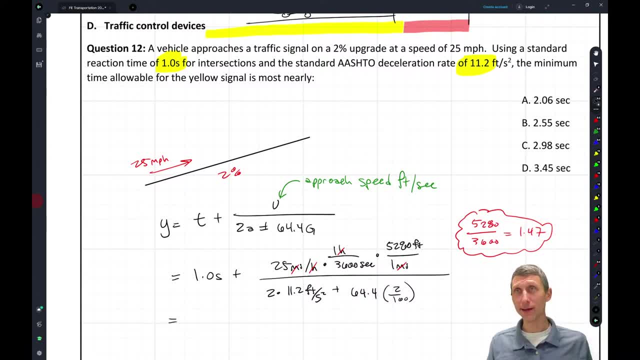 That's why we double check our work, That's why I do these ahead of time And you know, try to double check my work. But when you put all this in, I think you get about 2.55 seconds to which somebody is. 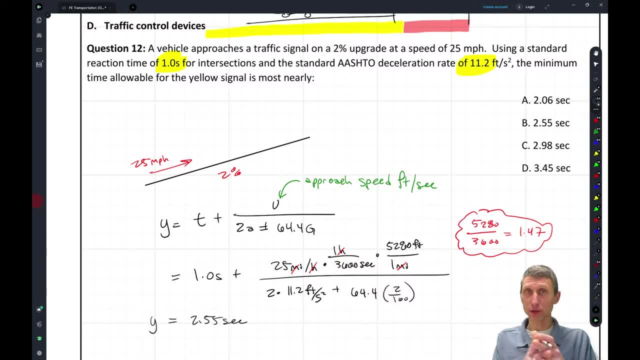 now going to. every time you stop at an intersection, you're the first person you're going to see around the corner and sort of see that yellow light and you're going to count one 1,000, two 1,000,, three, 1,000, then you're going to don't hit the gas yet because there's 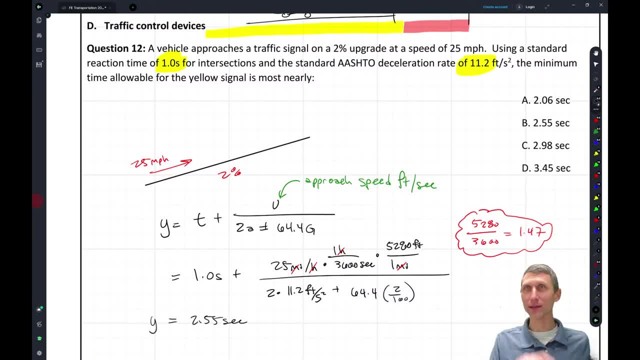 that one second of all red, Okay, So typically it's. it's typically not three to four second range before the light turns green. I know, maybe I'm maybe I'm just the one that does that, but it looks like it counts in. 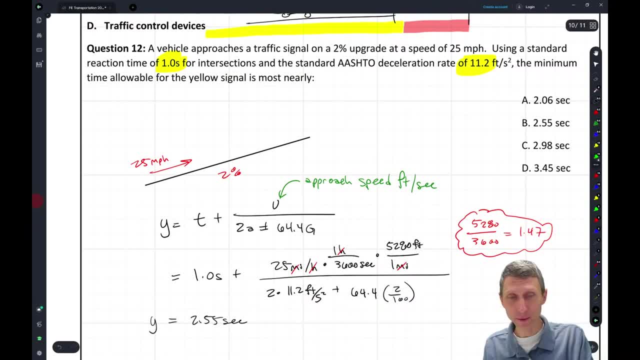 my mind Like how long is this going to take till I can go again? Okay, But that's where we end up with about 2.55 seconds. Normally that would be rounded to three. Okay, So typical, typical, you know, typical, typical times. 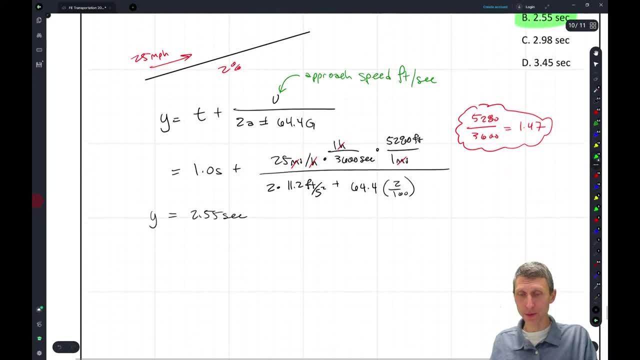 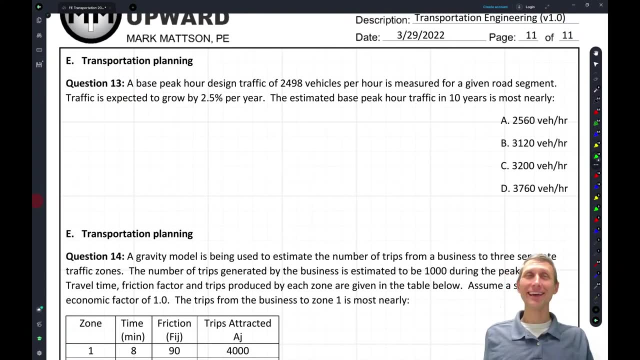 Okay, So let's keep going. Transportation planning: This is one of those ones where I was looking at transportation planning And I think I mentioned this earlier in the stream, but maybe that part got cut out, I can't remember I was. I was looking at the transportation planning section and the transportation planning. 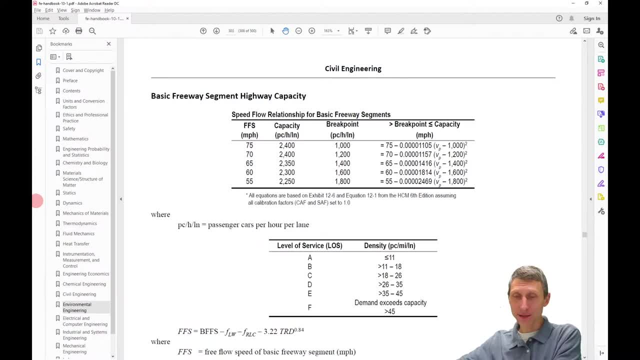 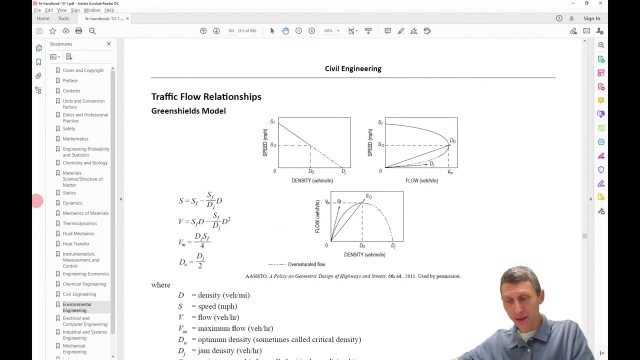 section in the handbook is interesting. It's there's a, there's a lot of stuff in here And honestly, actually, let's just, let's just well, yeah, let's go there, Let's go to transportation planning. There's a lot of stuff in here. 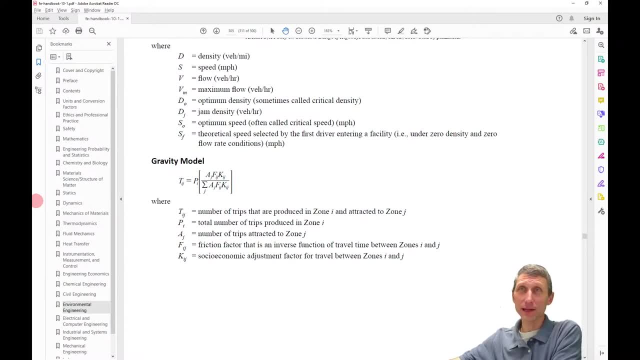 There's a gravity model and that can get pretty complicated, especially if you get more than one zone. If you get like two or three zones, it can get pretty complicated. And then the real world: there's a lot more than three zones so that that model can get. 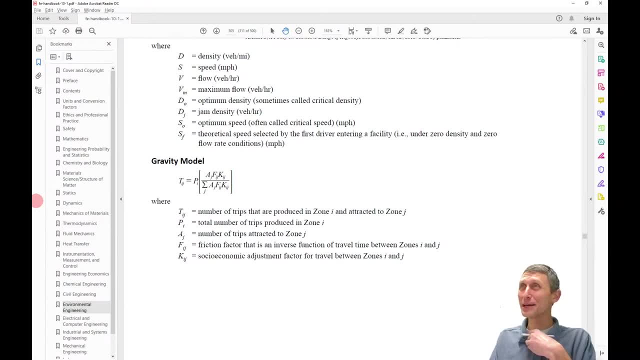 pretty complicated. We're going to do a basic example. And the reason we're going to do a basic example is because I think I mentioned the last time I did a transportation review. I said like, yeah, the gravity models are just kind of. 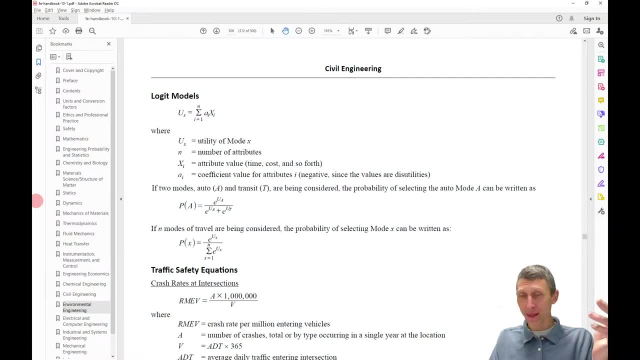 complicated, So it's a logit or logit model, depending on how you say it. You know they're pretty complicated, but they can be broken down into simpler questions. I just I picked gravity partly because that student came back and said: Madison, there's. 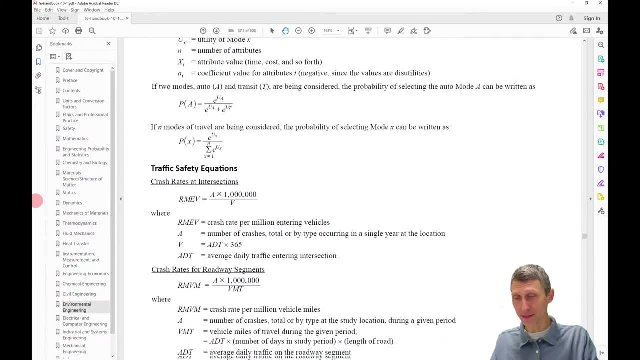 a gravity model question And I was like, okay, I'm going to do a gravity model test. So we're going to do a gravity model. I don't know if this is the same type of question that he saw, but it's just the kind of a basic. 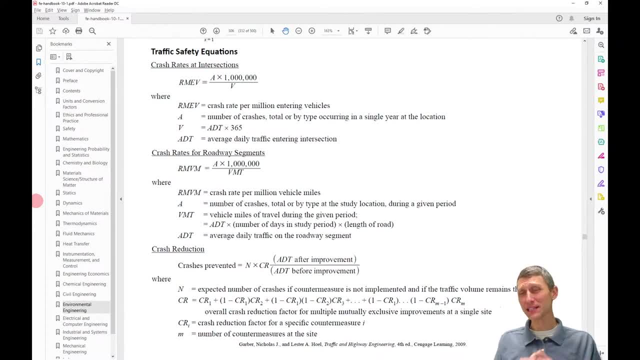 question to figure out how to use this. And then there are also these traffic safety equations. and these traffic safety equations there are a lot of plug and chug. I mean this is: this is kind of like the structural number equations, You know it's it's kind of looking at like, with safety, how can we, you know, have what? 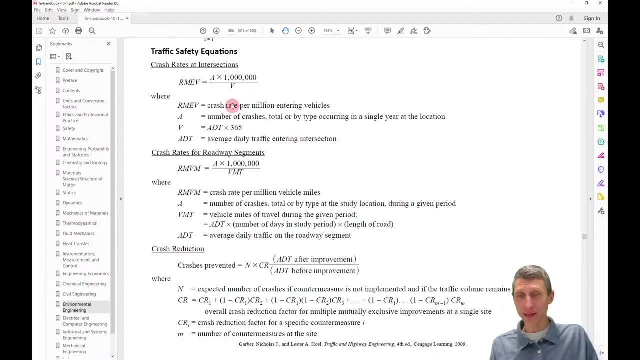 what are the crash rates? So we look at the number of crashes times a million, Right, So this is a million, and we're looking at average daily traffic times 365.. So we're looking at our total volume here. So we're looking at kind of this crash rate. 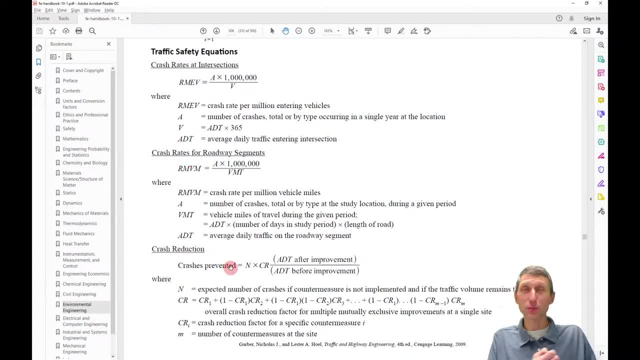 We're looking at crash rates for roadway segments, We're looking at crashes prevented. So maybe you say: well, okay, we're going to, we're going to do something and we're assuming that's going to. you know, reduce bias, reduce the crashes by a certain amount. 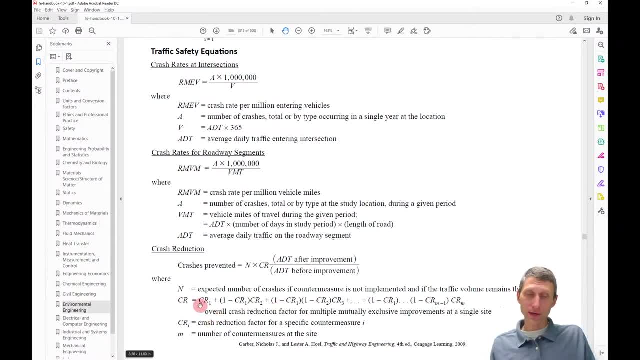 We'll get in there, And if you have more than one countermeasure, That's you- You're going to have to do it at the same time. I think that's another thing I wanted to introduce at a. you know, typically if you're doing, 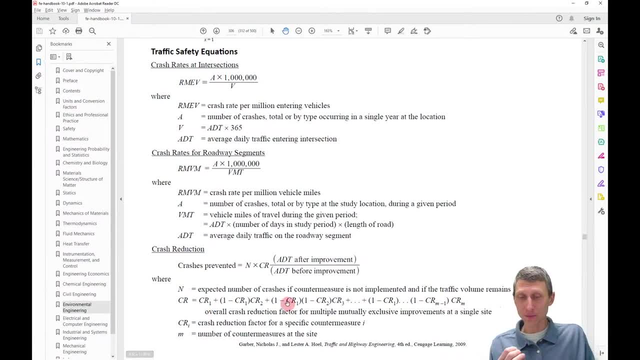 an intersection upgrade. you're not just doing one thing, you're doing a couple of things, So so you have to modify the percentage. that only gets a little bit trickier. Maybe, again, if I do another one of these, I will throw that in there. 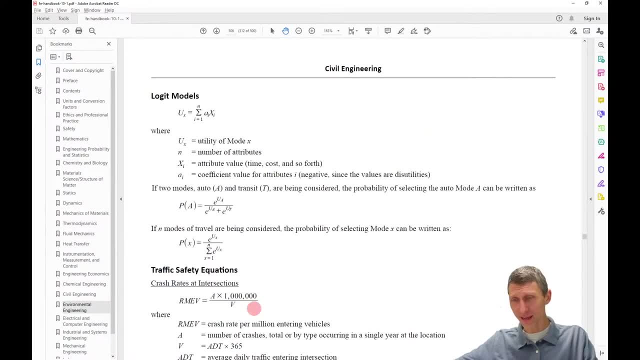 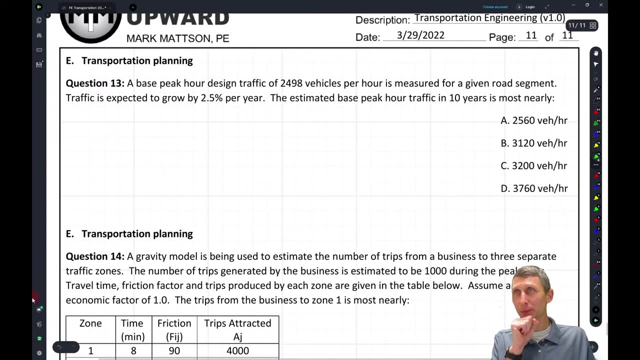 But what I wanted to, what I kind of wanted to focus on here, was just some basics, And this is where this one isn't exactly in the manual And I thought it was one of those ones where it gets used and typically you're designing. 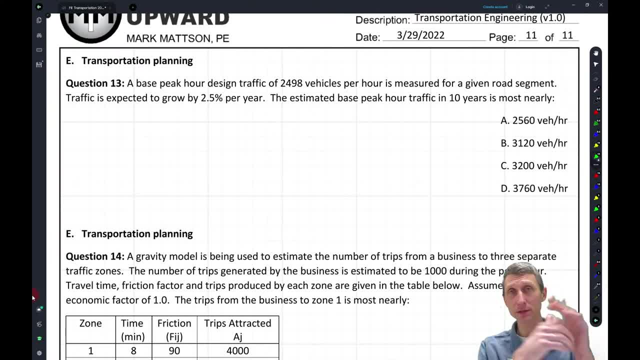 a project, but it's going to be three. you know a couple of years, maybe. know a couple years, maybe, especially it's a larger project- before it gets built, and then you're going to be looking at what's the 10-year capacity, what's the 20-year capacity, what's the capacity. 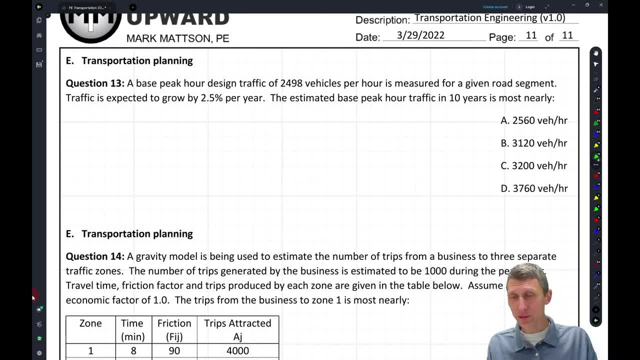 of lifespan in this thing and you're looking at growth, and this is interesting because we kind of get this idea that that sometimes the handbook is is contained, but we also have to know the different pieces of it. so we have a speak peak design traffic of of 24.98. right, that's our 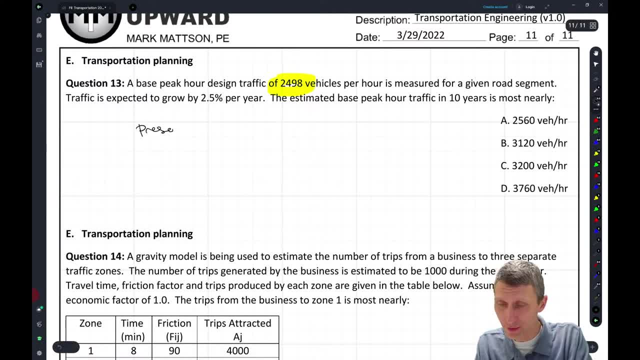 typical. that's our, that's our present uh traffic. you know, present traffic is 24.98. and then we're saying we're doing some things to it and we're expecting traffic to grow two and a half percent per year. and what's the? you know what's the? the traffic in 10 years. so 10-year volume, right is. 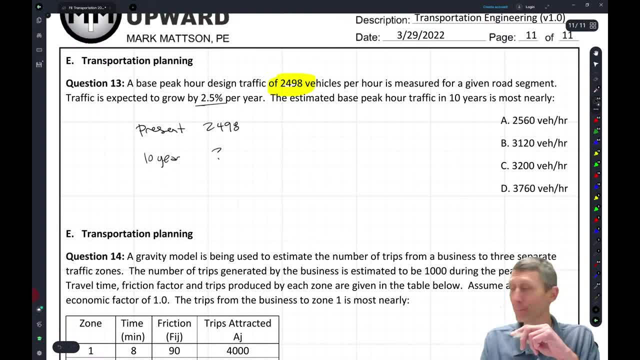 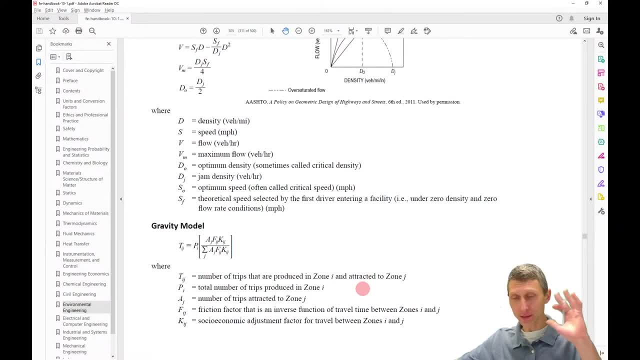 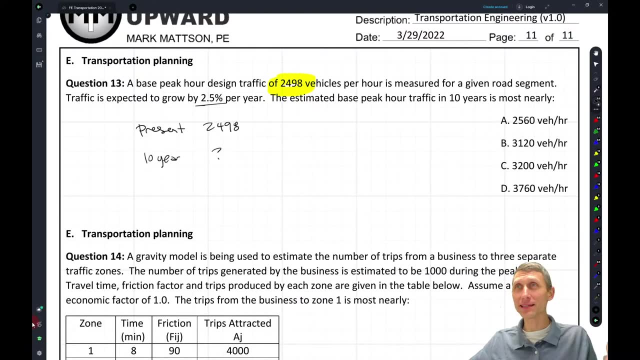 so what is that? what is that going to be? and we can come back in here and we can take a look at, you know, our, our models, we can take a look at gravity models and all these things, but, but, but this gets back to fundamentals that just you just keep multiplying by two and a half percent per year. so, yeah, this. 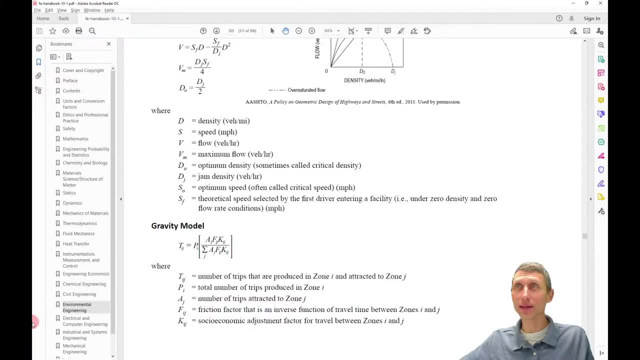 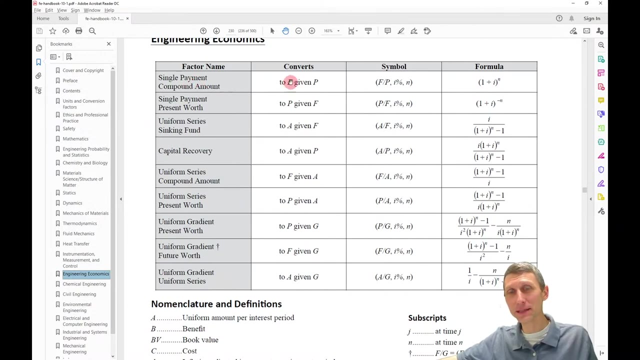 becomes compound interest, which is interesting because, uh, even if we come back into here, we have what we have- engineering economics. at some point where managing economics go, it's, it's somewhere and i always miss it there it is. engineering economics is pretty interesting because what do we get? this isn't a payment, but this is just a compound interest formula. 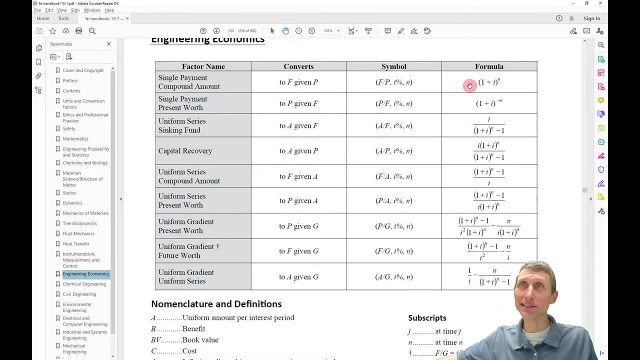 right one plus i to the n. that's one of those formulas. i joke it. it's like in the construction administration class that i've taught to in the past. it's like there's like virtually no math. it's like looking at contracts and administration and how to write forms and that sort of thing, but it's like 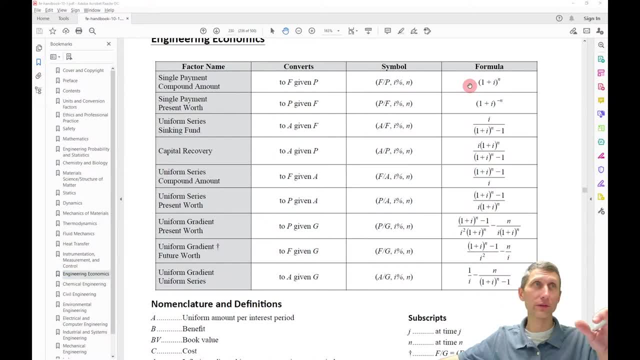 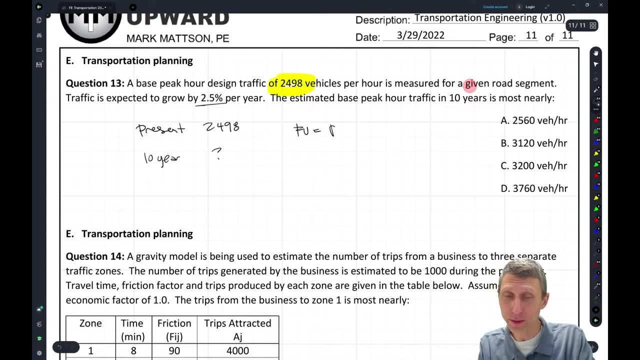 this is one of those formulas that it works in economics, it works in transportation, it works kind of everywhere, so that that formula looks like this: so the future value equals what the present value times one plus i to the n, so that's multiplying by two and a half percent over, and 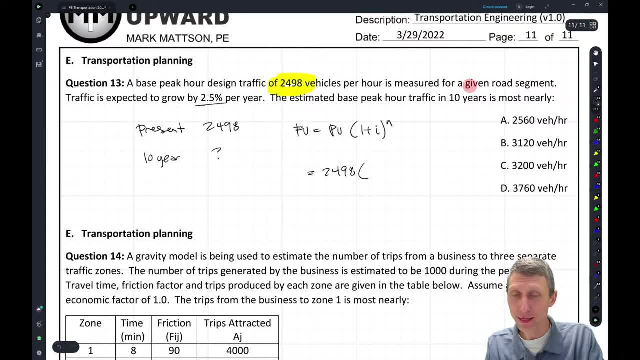 over again. but yeah, what do we get? we get 24, 98 times 1, plus 0.025 to the 10.. so this is kind of a simple question, but it uses one of those kind of like basic formulas that gets you know possibly. 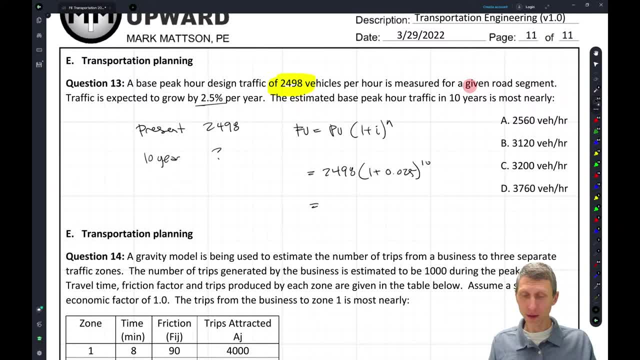 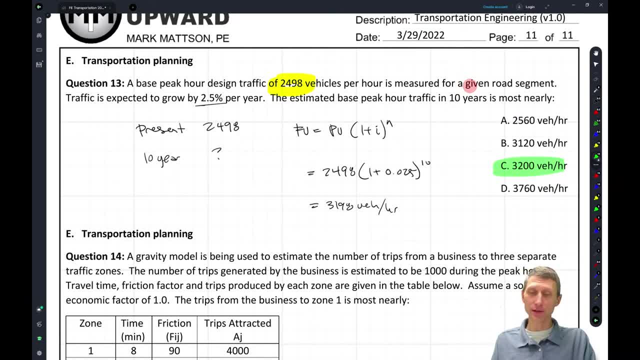 and then you know: but again, compound interest, whether you're looking at cars or you're looking at uh, you know, whatever you're looking at, this is. this is one of those things where it helps to kind of know some of those basics, like the compound interest formula. and here's that crappy model. 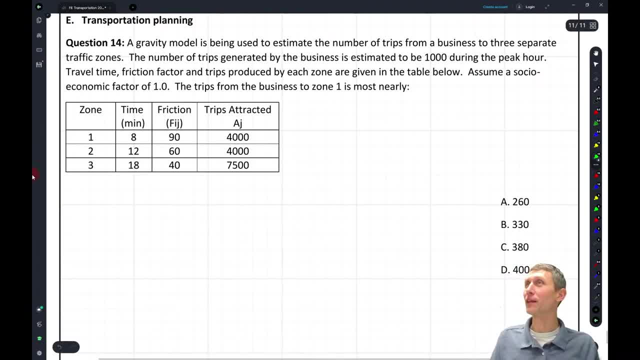 question. so this is the last question that'll tell a joke and hopefully i'll laugh about um the fact that you know the the stream cut out earlier, but we'll see how that goes and uh, hopefully this this stream worked okay, but um grevin miles being used to estimate number of. 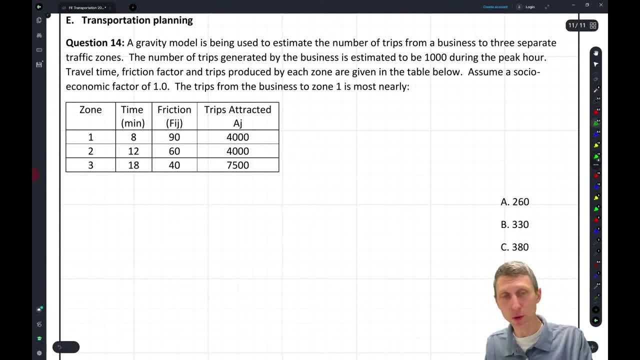 trips from a business to three separate traffic zones. so what we have here is typically, when you're doing a transportation study, um, you're put you, you're putting in some sort of you know business. am i spelling that right? i don't know. we're putting in some sort of business. 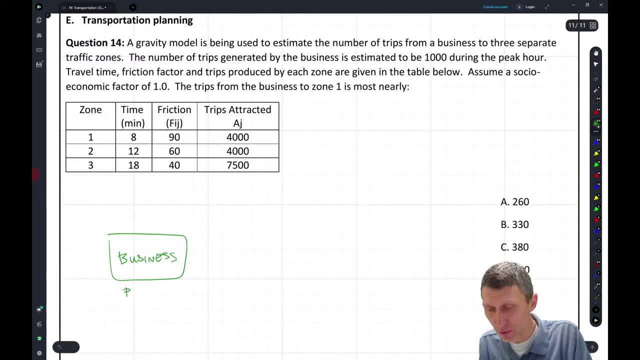 and we're generating trips from that business. so we're saying we're producing 1000 trips. so we're gonna, you know, we're taking a site, we're developing it, we're gonna produce a thousand trips for that site and we're wondering where they're gonna go. well, in order to figure out where they need to go, we need to know what's. 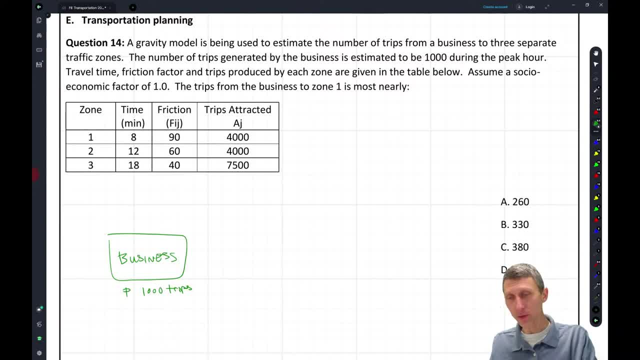 around that site. so this is kind of the way the gravity model works. it says, okay, well, i have three different zones that are near that site. i've got zone one, i've got, you know, zone two and i've got- oh, let's just use red, yellow, red and green, why not? i'm going to put them in the 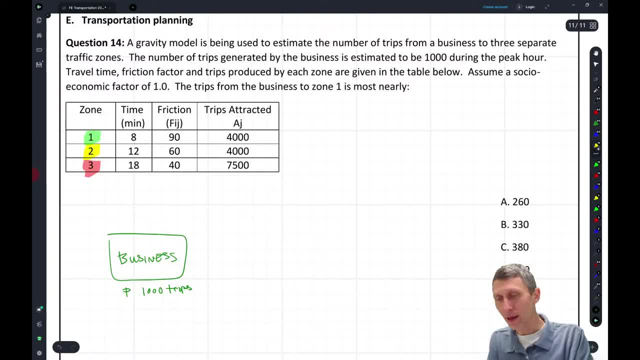 so, uh, we'll use yellow, red and green just because we're dealing with traffic, right. um, so we've got three zones that are going to attract the site, so it's like you got a business, but somewhere you know. this business might be in zone one, because it's pretty close to it, might be in 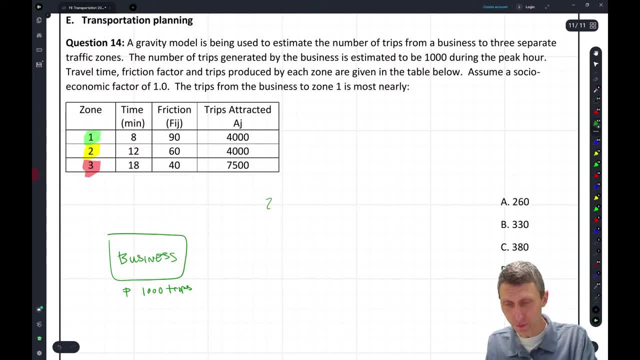 zone one. but we're going to say that we have zone one um, zone one over here and that zone attracts about four thousand trips. so that's you know, a1, it's ai a1. it attracts four 000 trips from kind of all over the place and it's going to attract some trips from the business. 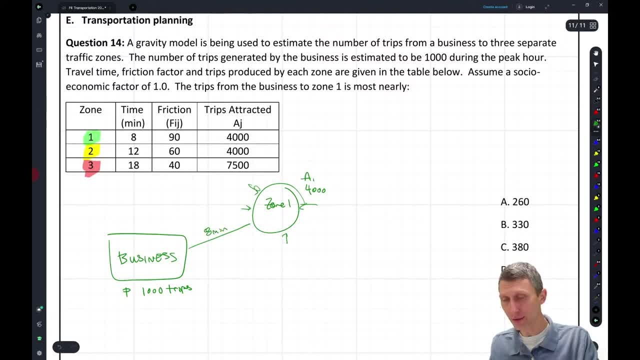 does that make sense? so the the time- that's the average travel time to get there- is going to be eight minutes. so some of these trips are going to go there, some of these 1000 trips are going to go there. and then we have zone two, and i'm going to draw this, you know. so actually, let me just 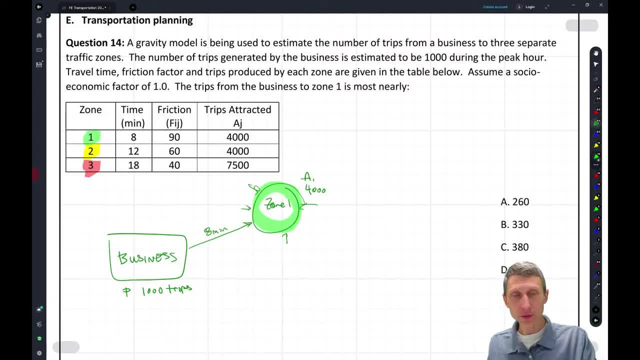 let me just highlight that one in. so that's zone one. okay, then we're gonna have zone two, and zone two is a little bit further. so instead of eight minutes, this is going to take us 12 minutes to get there. this might be a different. you know town, or the night, the other going, the? 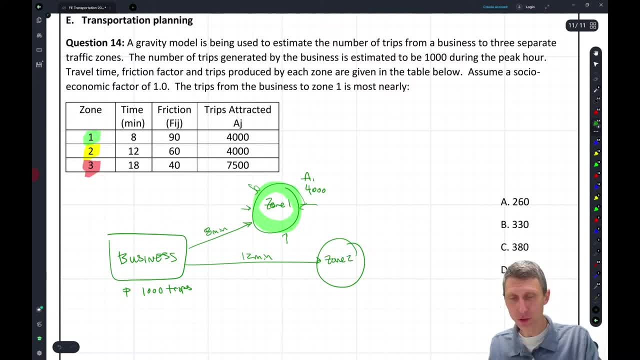 other direction. this is going to be zone two, okay, and i'm going to do that one in yellow, and overall this zone has, you know, a total of 4 000 trips coming in as well. so the the idea of the gravity model is, even though these both have 4 000 trips coming in, zone one is more attractive. 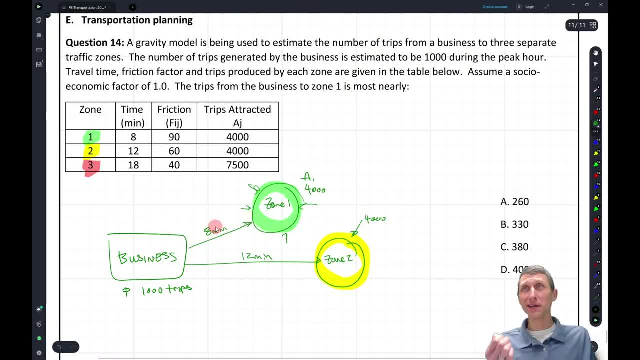 more people are probably gonna go from the business to zone one because it's a shorter travel time, right? i mean the the you start getting further away, you're less likely to go to that place. so the kind of idea here is this: is you know, it's gonna produce a thousand trips, probably gonna have, you know, more trips. 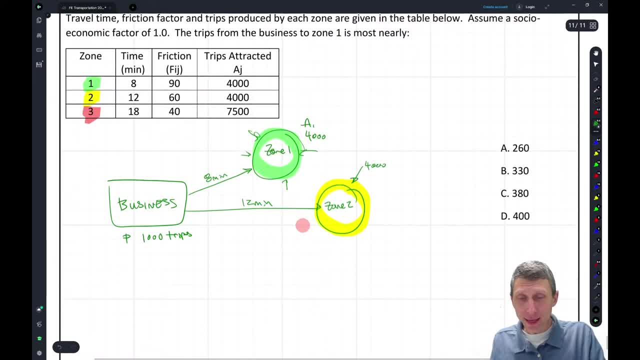 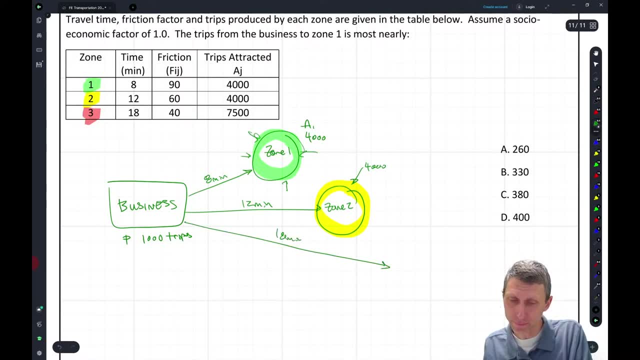 to zone one, even though these two are the same size. but then we get down here with zone three and zone three is even farther away. okay, so this is 18 minutes away, but this one's bigger. okay, and i drew that one bigger on purpose. this one's zone three, because zone three. right, what does zone three? 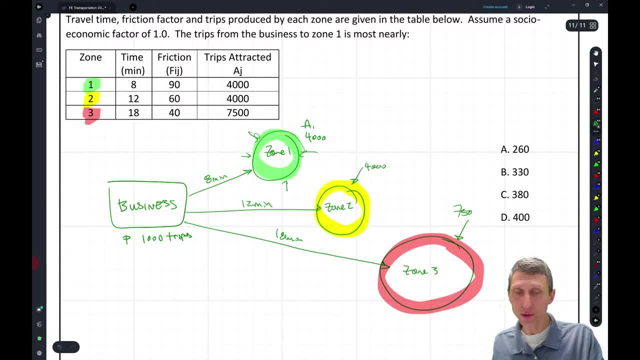 do? it attracts 7 500, right? this one's bigger than zone one, and zone two are going to be even further away, so this is going to attract a total of 7 500. this is like a three, so a one, a two and a three. 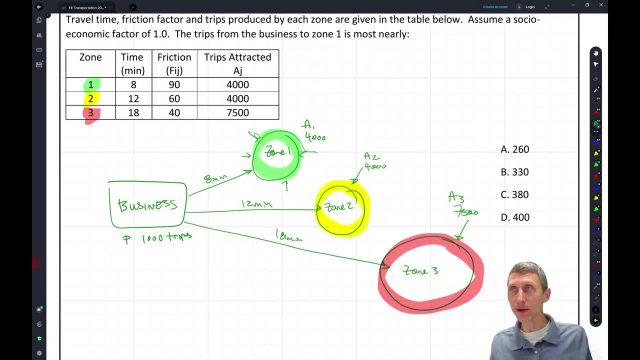 and this is going to attract some portion of the thousand trips from uh, from from. you know this, this business. so the idea, the question is: how many trips are going to go to uh zone one? okay, question is, how many of these thousand trips are going to go to zone one? so we're going to take part of that. 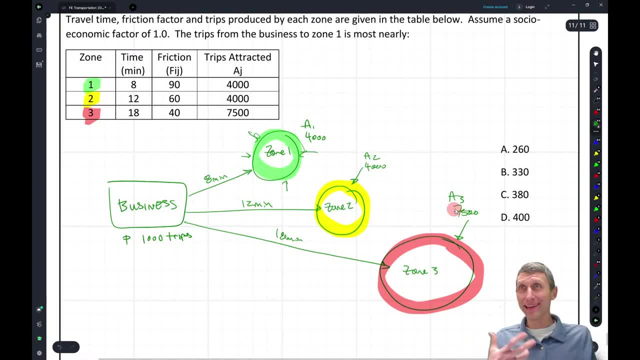 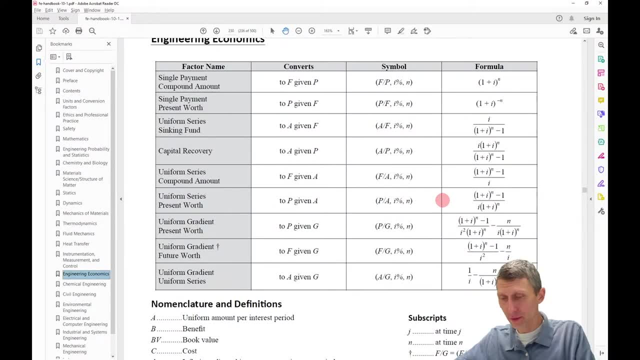 we're going to take that part of that thousand and just split it up, kind of each way, and we have to that out. so the what the gravity model says is is this: the gravity model says: uh, let me come back to civil engineering here. actually i'm going to go and do environmental. 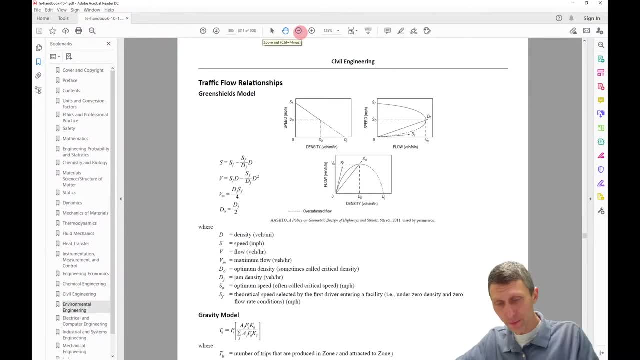 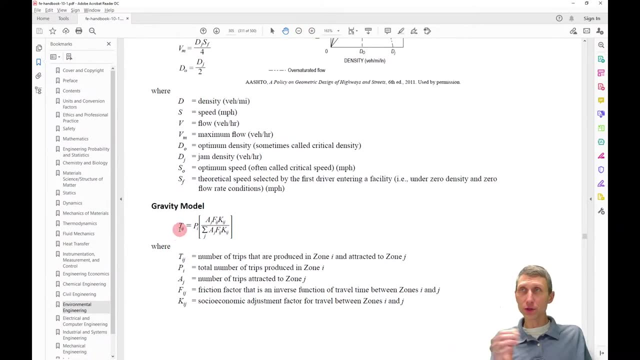 and then back a few pages and the gravity model says this. it says- let me zoom in a little bit- the trips from one zone to another, from one place to another, right, is equal to the trips produced in zone i, or this is the trips produced at the business times, the 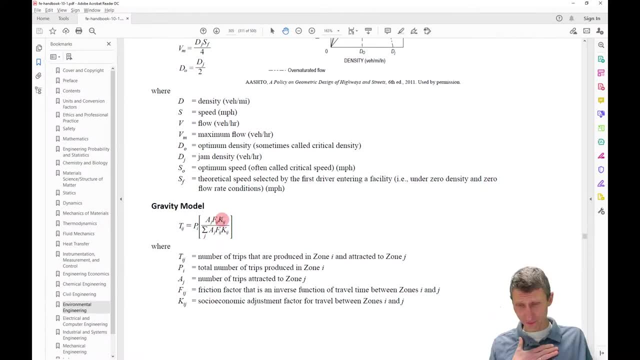 friction value, some socioeconomic factor. divided by the sum of those, this is kind of like a weighted average. okay, and what we have going on here is this is a- you know, this is a weighted average where we got aj, fij, kij, so let's let me just going to bring come back over here and write that down. 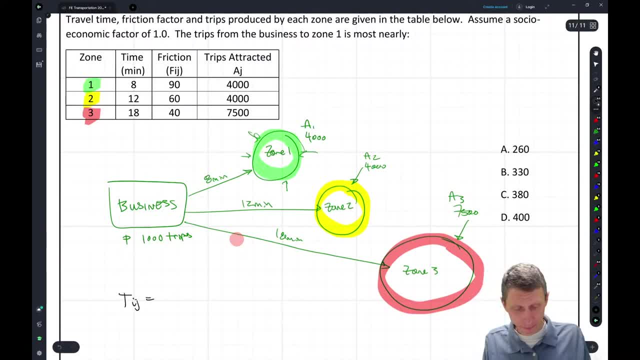 so i'm going to say the t i j equals. this is the trips from one zone to another. so equal pi times times uh aj times f i j times k i j, all over the sum of a j times f i j times k i j, and this looks kind of. 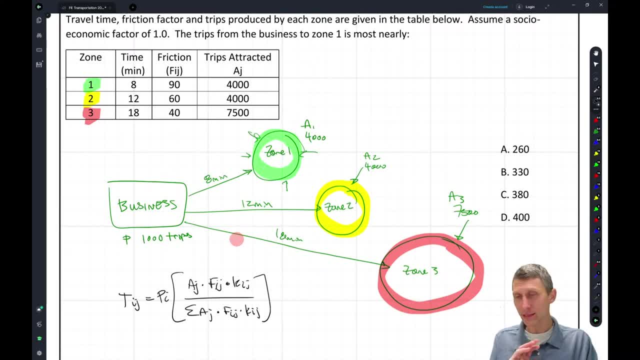 ugly and it kind of sort of is, but it's really not that bad. this is kind of as simple as i think i can get it for you in in terms of a fe type question, because normally if you're doing this type of thing you're going to be doing a spreadsheet, you're going to have a whole 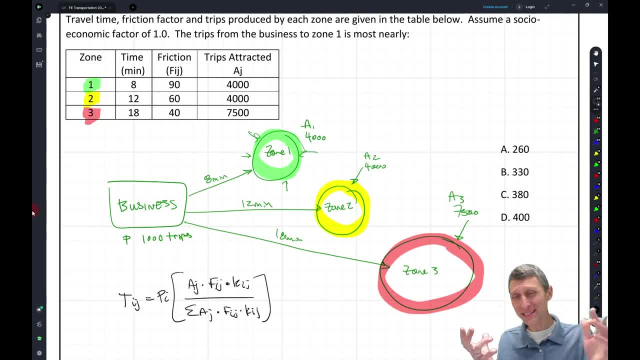 bunch of things worked out and a whole bunch of, you know, matrices going on, but this is a, this is just one business producing things and going to different zones. so let's, let's figure out what happens, basically what. we have this f i j, we have a j um, and and we, we were told the socio and 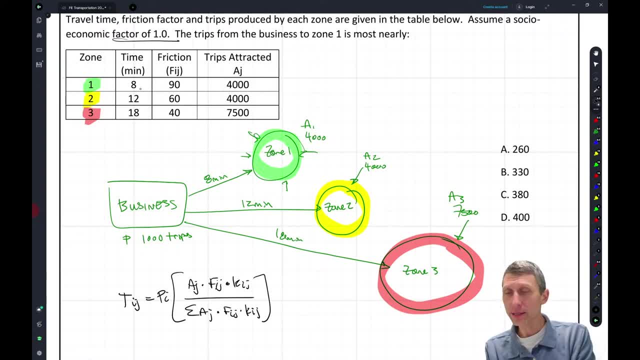 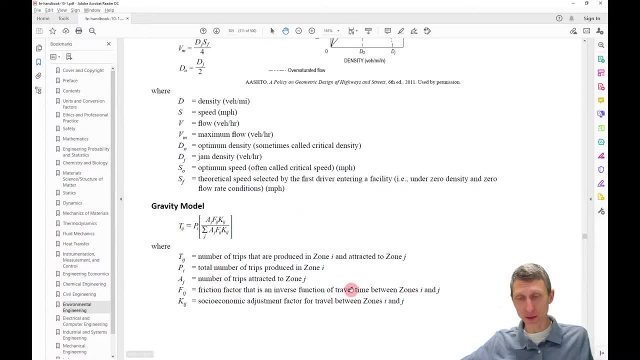 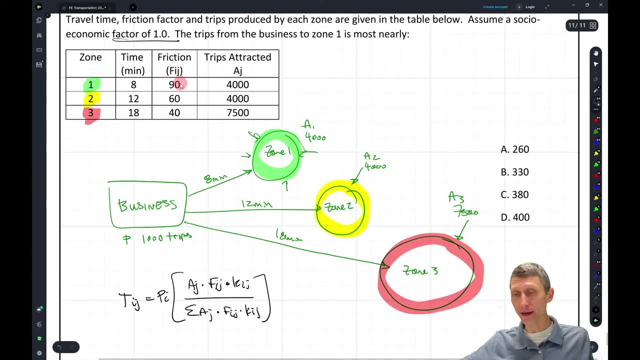 economic is one. one thing to note is the. the time and the friction are typically related, so typically the like. there's an inverse proportion here between um, the time and the friction factor. so the closer you are, the higher the kind of, the higher the attraction, if that makes sense. 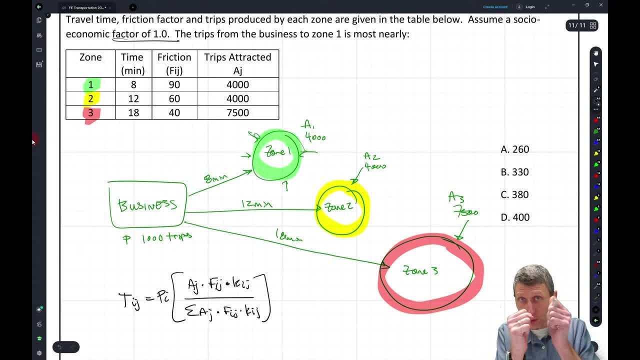 and that's where the gravity model, the gravity idea, comes from. the closer two bodies are, the more, the more force there is that attracts them. so all i'm going to do here is i'm just going to say: i'm going to make a new column. i'm going to say a, j, f, i, j, k, i, j, that's all right. so i'm just going to. 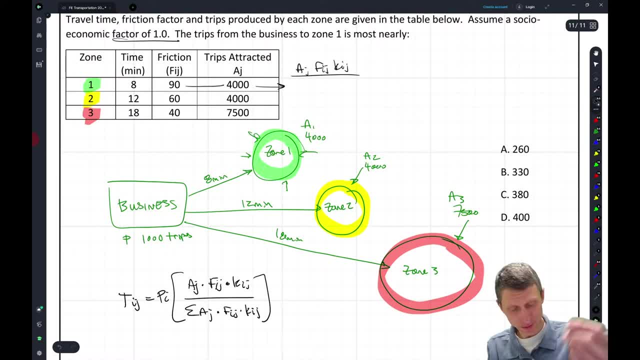 multiply 90 times 4 000 and get- i think it's what's that? 360 000, right? and then i'm going to multiply 60 times 40, 4 000, i'm going to 240 000, and then i'm going to take 40 times 7 500 and i'm 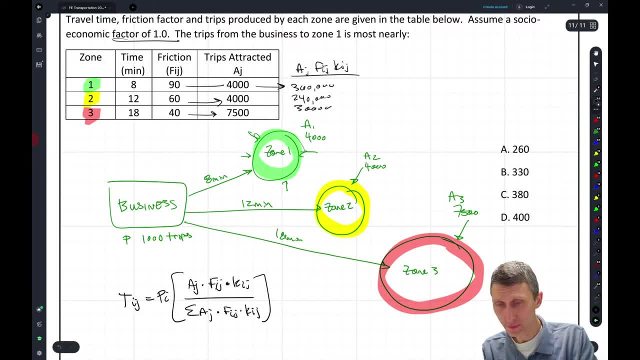 going to get um 300 000 and i'm going to move this out of the way just because it's in the way, um, and what i'm going to do next is i'm going to add all these up, so i'm going to. the sum is going. 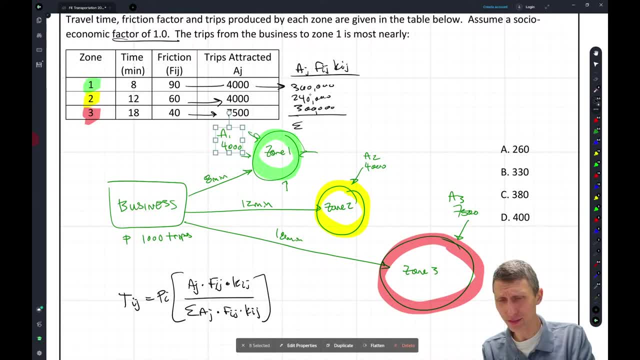 to equal. if i add all those up, the 60 and the 40 get added together. so that's like i think it ends up being nine hundred thousand, and then i'm going to multiply 60 times 4 000 and i'm going to get. 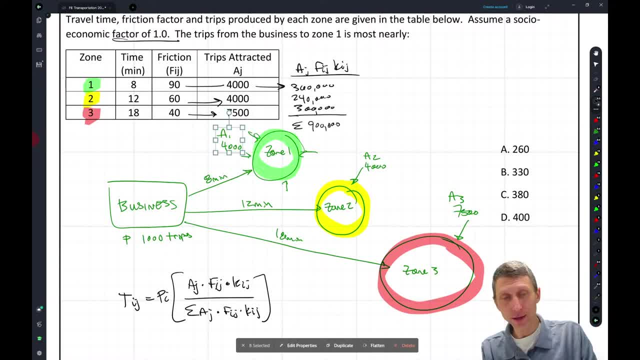 then i'm going to kind of get this percentage here, right, this, this ratio, um, that that we're trying to find. so this is going to kind of be what's next. this ratio, uh, is going to be what's next. i'm going to say a, j f, i, j, k, i, j over the sum of a, j, f, i, j, k, i, j, right. so what's that? it's just. 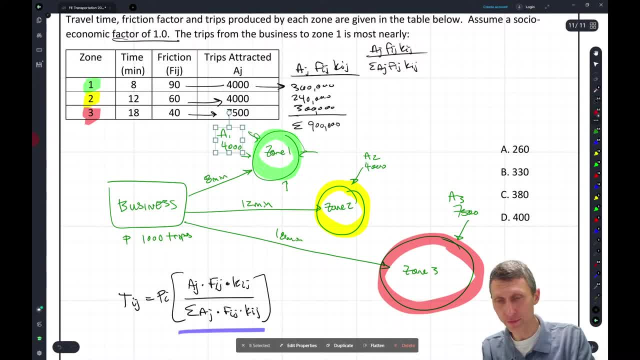 going to be. i'm going to knock off a whole bunch of zeros here, so i'm going to get rid of the, you know, all these zeros here, just because, um, i can. but what does this work out? it works out to 36, or 24 over 90, or 30 over 90, and if you add all these up together, guess what you get? you get 90. 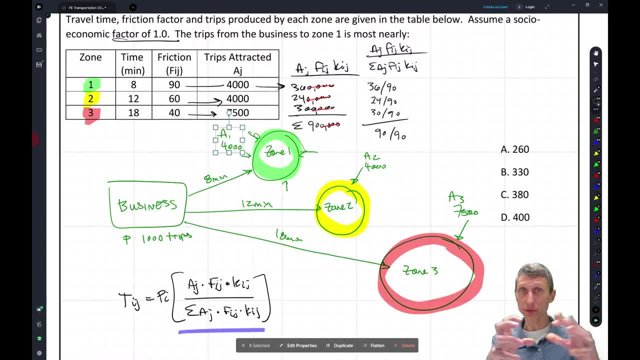 over 90, right, because it has to equal one. you have to distribute all those 1000 trips to the same spot. so this is kind of like our fraction here, and to get the tij, all that we're going to do is we're going to take, you know this- column times p pi, the number trips produced at. 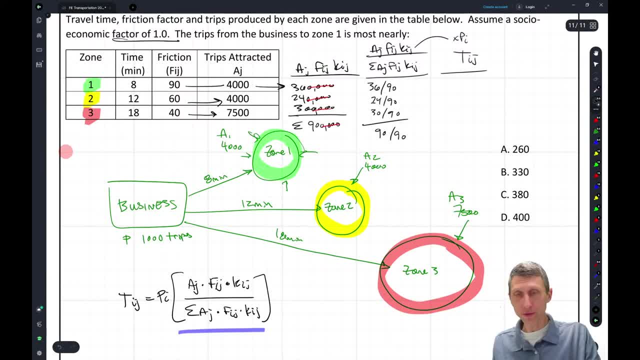 that business and we'll get our solution. so if i take this 36- 9, this 36 over 90, 36 over 90 and multiply it, right. so if i multiply it by that thousand, this is the, that's that p, right. if i multiply that by a, 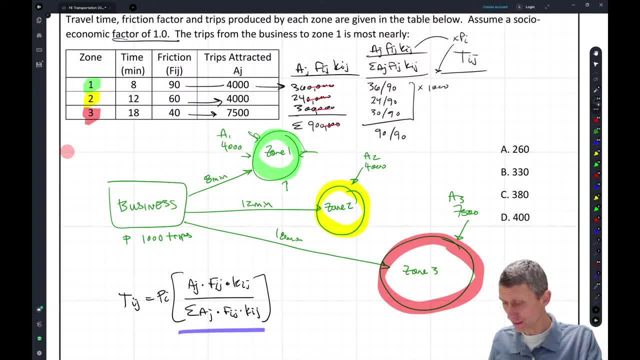 thousand i'm gonna get. what do i get? uh, if i put it in right to my calculator, i get 400 trips. and then if i do the same thing we would expect okay. so let's just, let's just double check this for a second. we expect zone two to have. 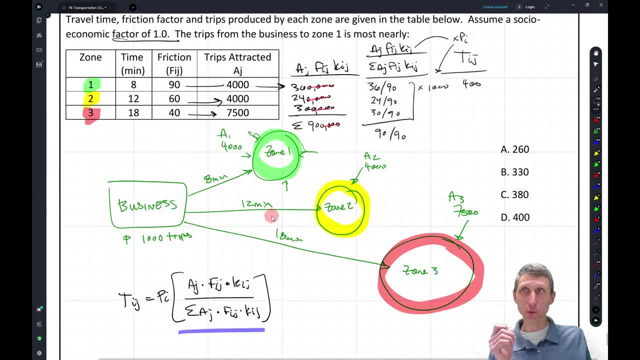 um, to have less because it's it's further away, even though it has the same number of attractions, same size. you know, earth ball or whatever you want to call it, um, it's the same size. we're gonna have fewer attractions there because it's farther away. we're gonna 267, and then this 3090 is going. 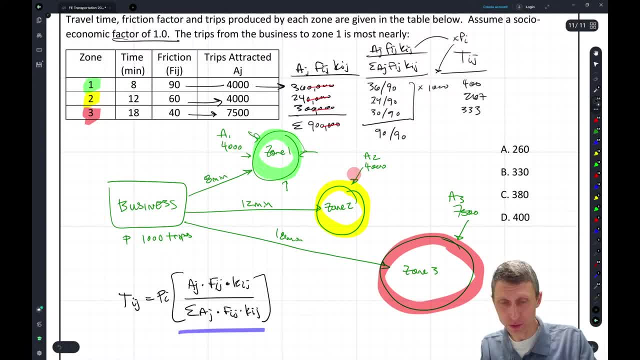 to be about 333. so the distance kind of impacts, you know, and that's what we're saying. we're saying this: this thousand trips is going to have the same number of attractions and then we're going to have going to get split up: 400, uh, 267 and 333.. so what's the socioeconomic factor? i put it in there. 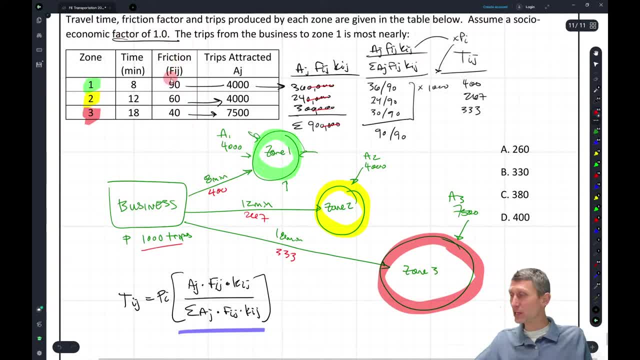 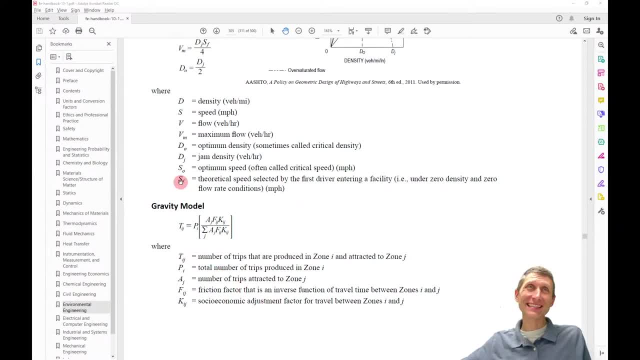 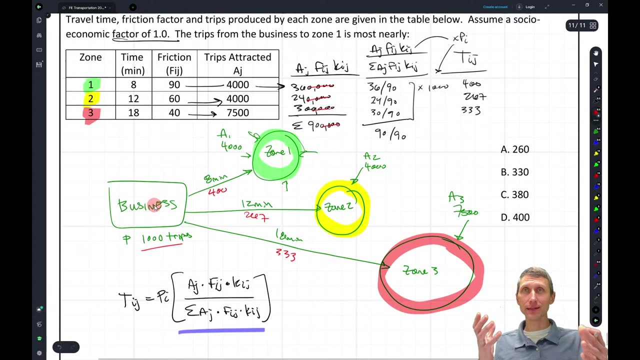 as one. i just i just called that out as one. that's kij, um that if we come back to this, you know we have kij socioeconomic adjustment factor, okay, and that's kind of thinking like, um, maybe you have a business that attracts, uh, you know, white collar workers, but there's blue collar workers in the. 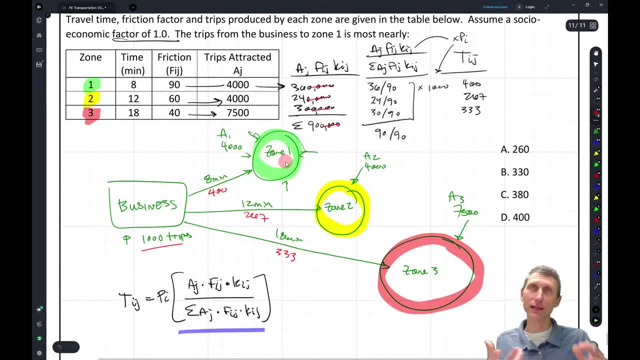 area that that could, that could adjust this thing. it's kind of like a calibration factor saying like, well, all these people don't shop at this store, so we have to. you know, we have to reduce this a little bit and it's just a way to calibrate the model. so there's a calibration based on. 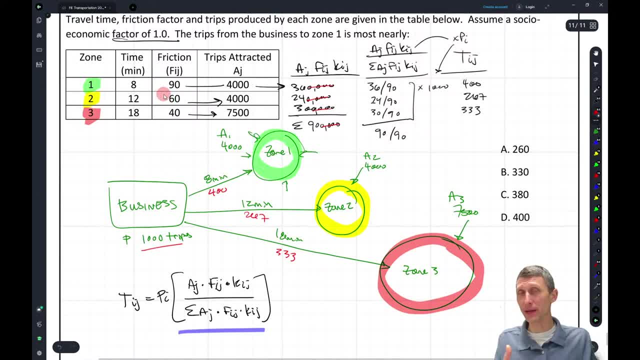 on time. on location, there's also a calibration based on, you know, whether it's a cultural factor or it's a socioeconomic. like again, you have a professional office building in a location where a lot of blue collar workers work, where they work in manufacturing, you're probably not going to get a lot of those. 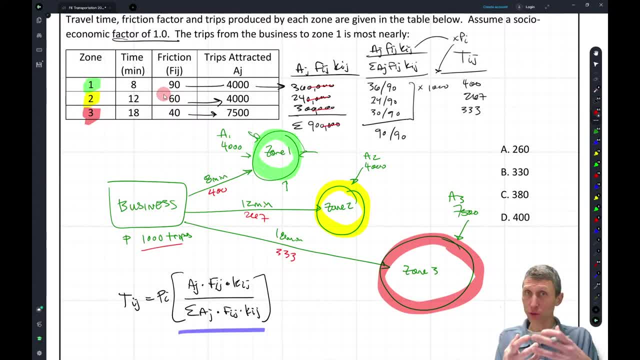 manufacturing people going to the professional office building even though they're close to it because they're, they have jobs in manufacturing, if that makes sense. so, um, that's an adjustment factor. but this gets us our answer. it it finishes us so that we can say that we have 400 trips. 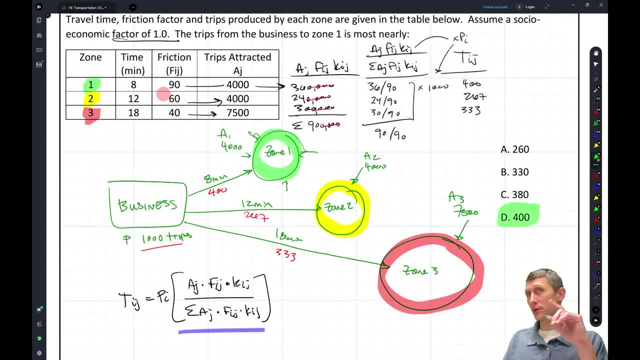 produced from the business to zone one. two trips to zone two, that's 2.5 million workers a year and then all kinds of other stuff. we have to look at that to get a good value. and the issue of the gravity model. but you know, i thought it was a. 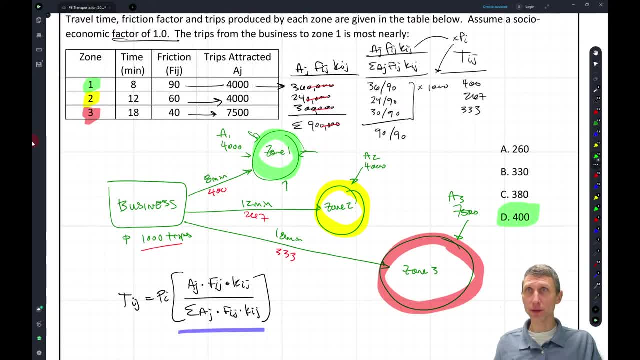 decent question, just to get the concept out there. it's not. it's it's sort of just a weighted average. it's really not. it's just looking at distribution factors, um, and nothing too too crazy. but the concept is one that, whether it shows up like on a question or just a concept question, it should work. 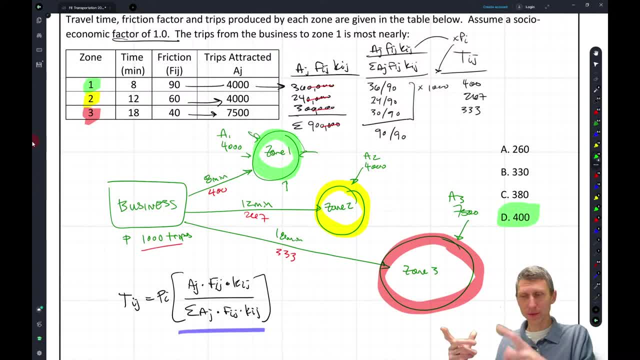 just like uh call it a night. i mean, i, i talked about maybe, maybe i'll even go through uh, go through the the first question or two and just review those quickly. but um, this was uh, it started out rough. i'll go delete that first half hour session. that just bombed. i mean i apologize for. 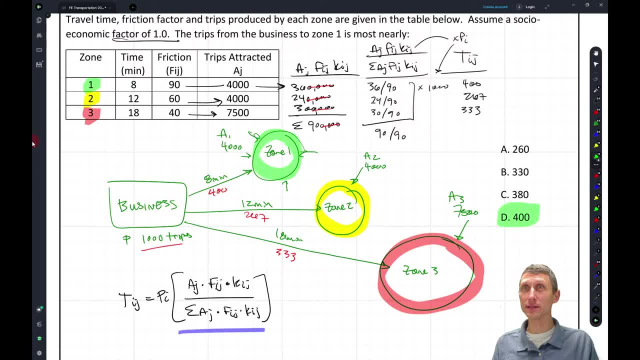 that my, my computer wasn't doing things the right way, but at least it fixed now. um, but hey, the next time you get pulled over by a cop and he says: why were you going there? well, first the cop was. the cop says: do you know? i pulled you over and say: well, officer, would you mind telling me? and 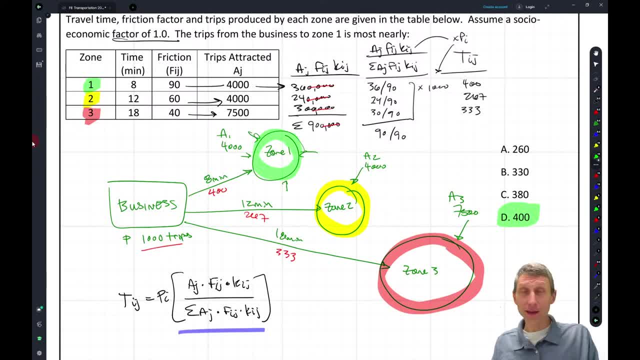 the officer says: well, do you have any idea how fast you were going? and then your response, of course, is: well, i was just trying to keep up with traffic, to which the officer responds, but there was no traffic. and then you could just get a sad look on your face and say: you see, i was so far. 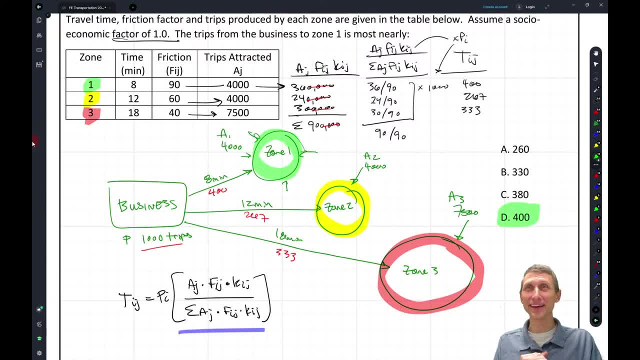 behind. i had to catch up. that really wasn't bad it. the other one i had was like: um, you know why does the red light turn red? because it's, it's, it's um afraid to to be seen changing. um, i, i don't know. you know there's bad jokes all around why? why did uh, you get a better, you get a better um grade when? 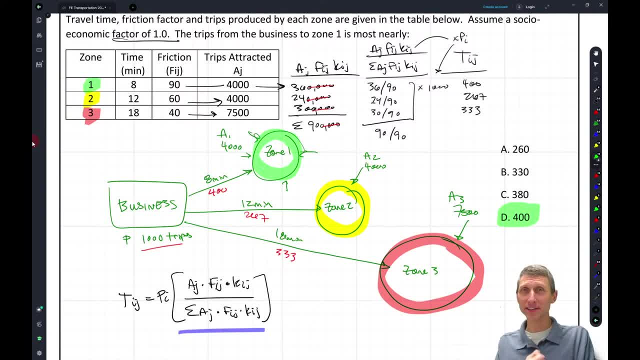 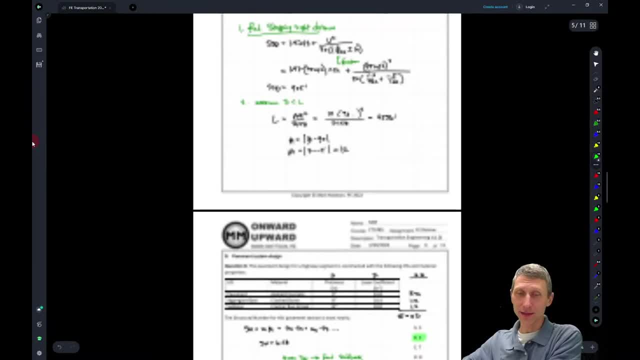 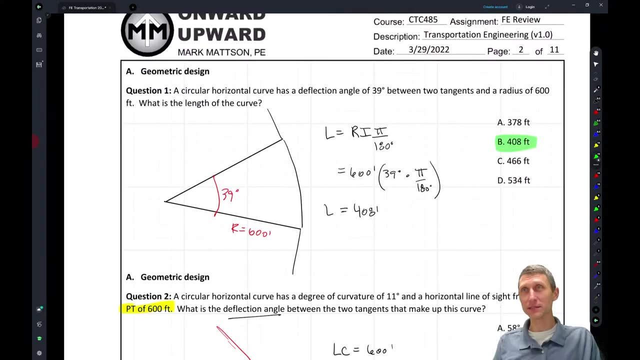 your professor was grading in the car because he was grading on a curve. okay, they're terrible, but hey, it's okay. um, you know, i think that's where we're kind of gonna quit here, just as we go back up to the front here. i think we kind of lost, i think the first half of this session we kind of